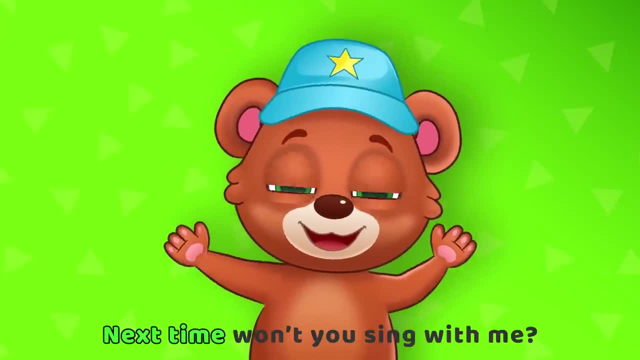 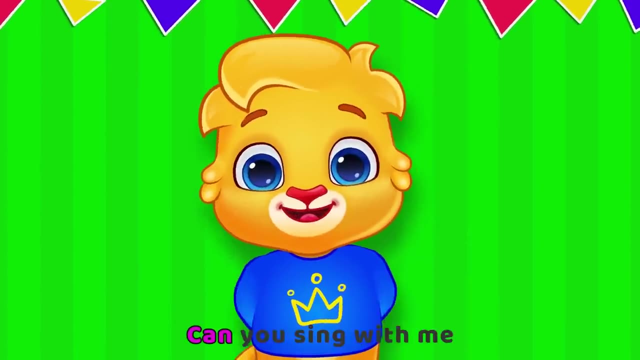 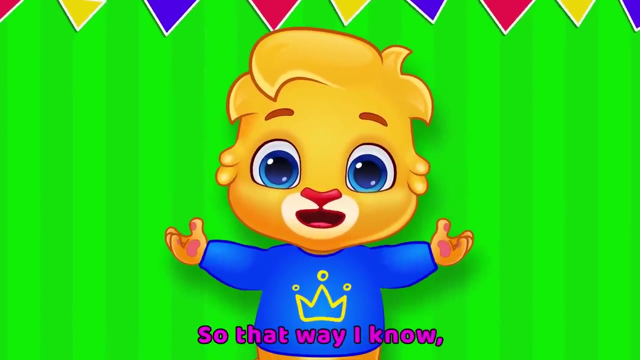 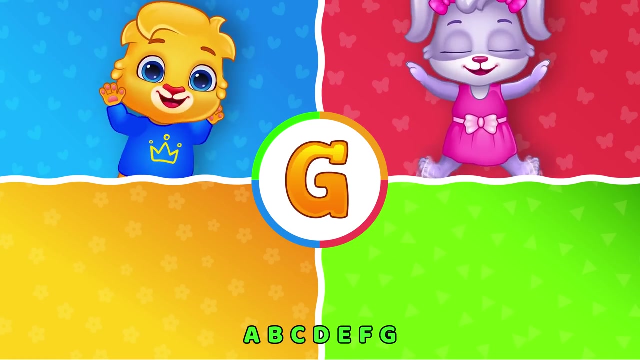 Now I know my ABCs. Next time won't you sing with me? Hi, I'm back again. Can you sing with me one more time with a loud voice, So that way I know you're listening. Let's do it. A, B, C, D, E, F, G, H, I, J, K, L, M, N, O, P. 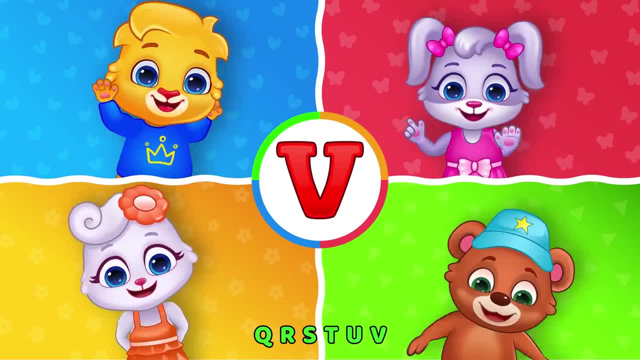 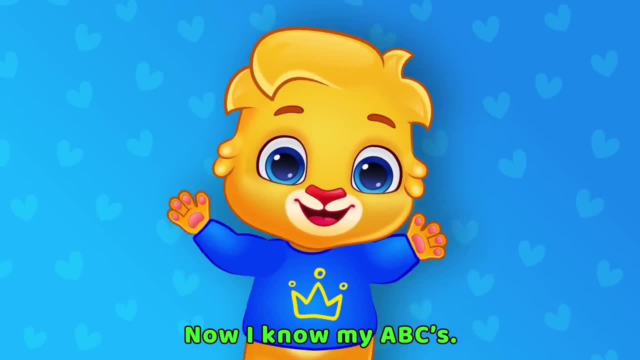 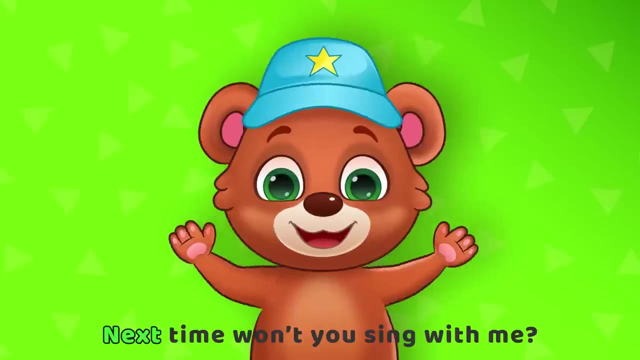 Q, R, X, T, U, V, W, X, Y and Z. Now I know my ABCs. Next time won't you sing with me? Now, I know my ABCs. Next time won't you sing with me. 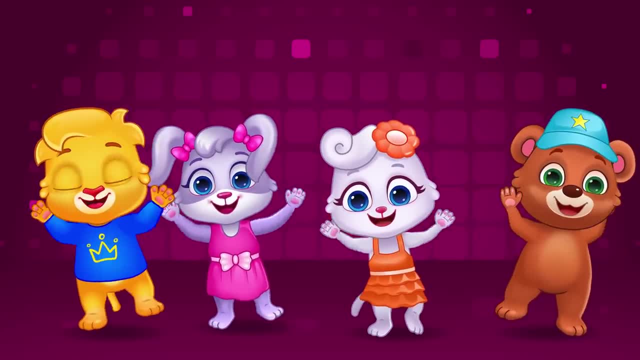 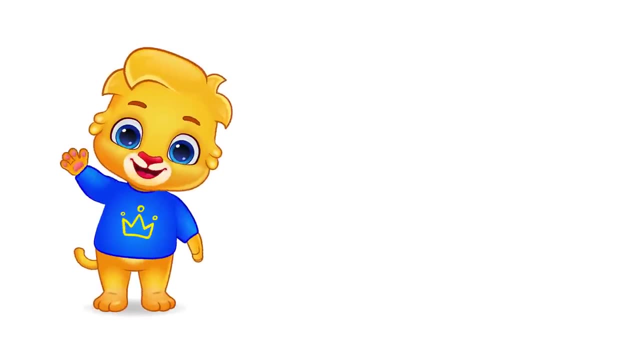 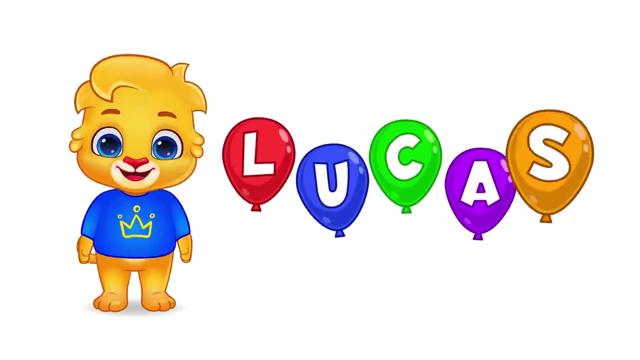 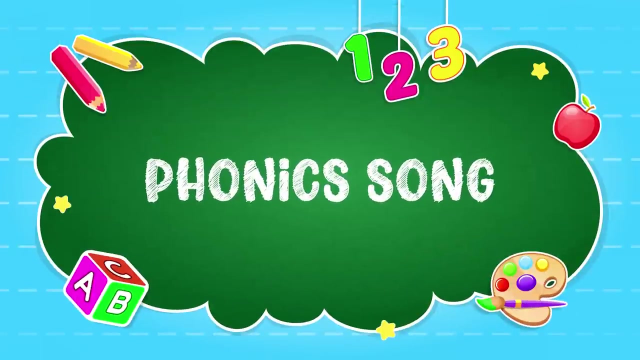 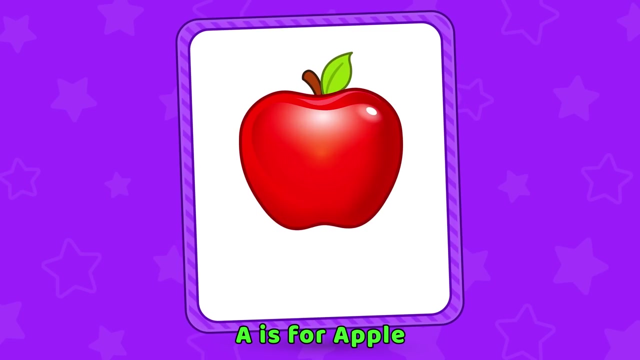 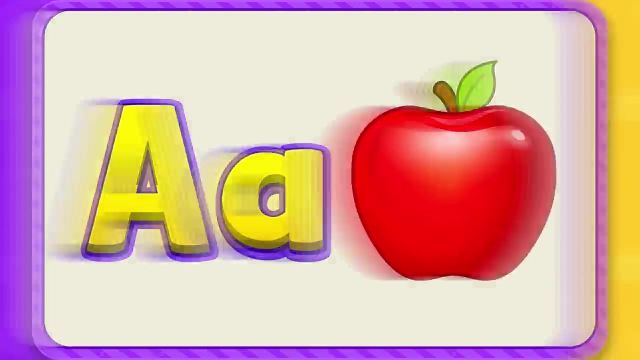 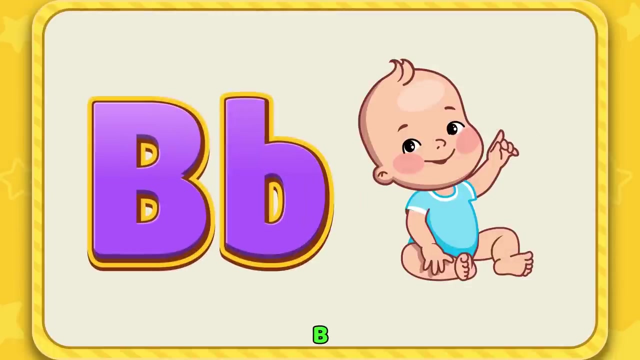 Next time won't you sing with me. A is for Apple A A. Apple A A, Apple A. Apple B is for Baby B B, Baby B B, Baby B Baby. 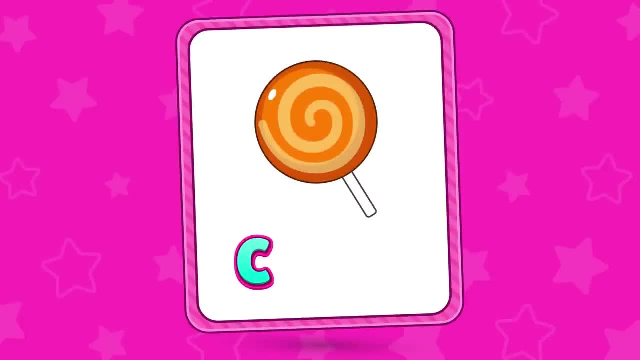 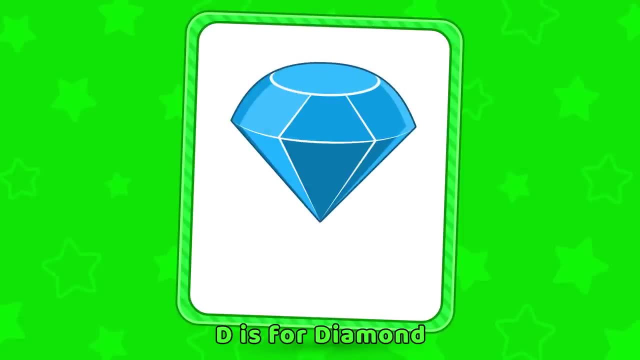 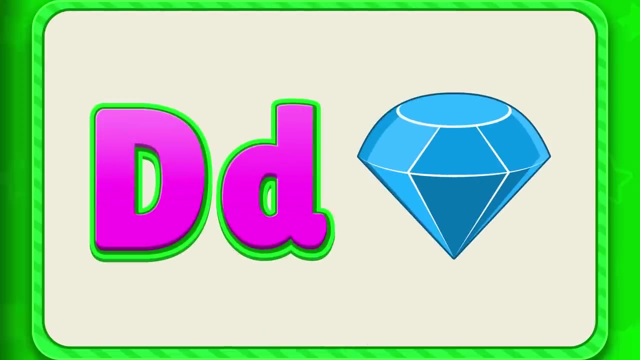 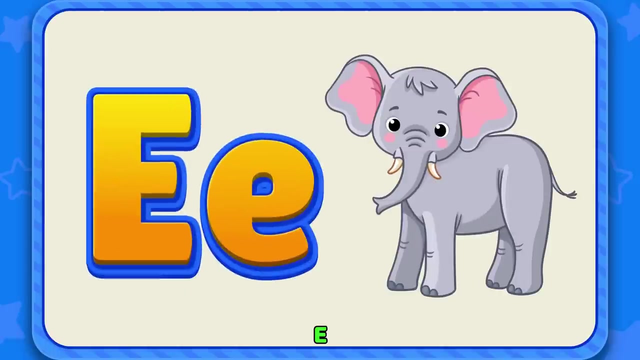 C is for Candy C C. Candy C C, Candy C. Candy B is for Diamond D D, Diamond D D, diamond D D, diamond D. diamond. E is for elephant E E, elephant E E, elephant E, elephant. 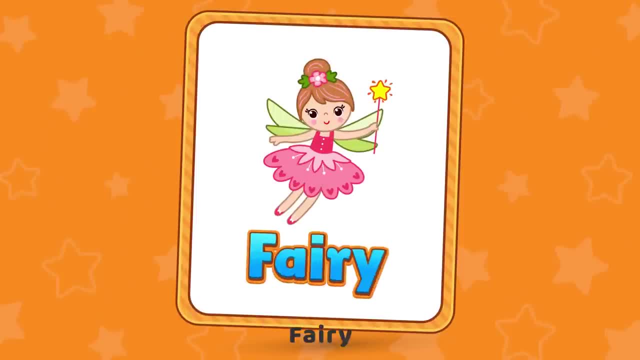 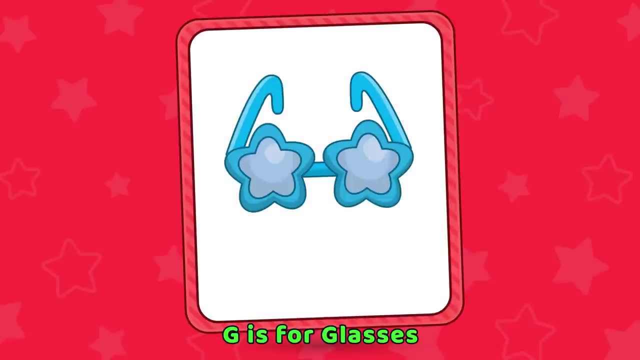 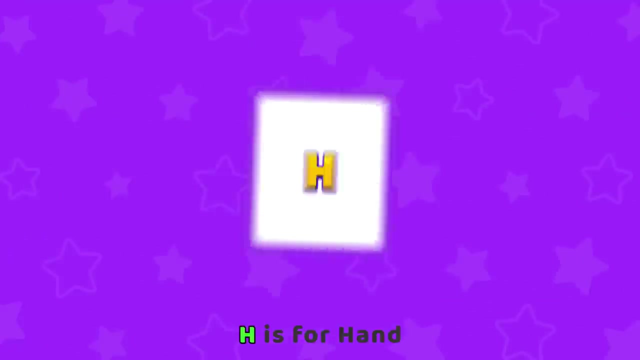 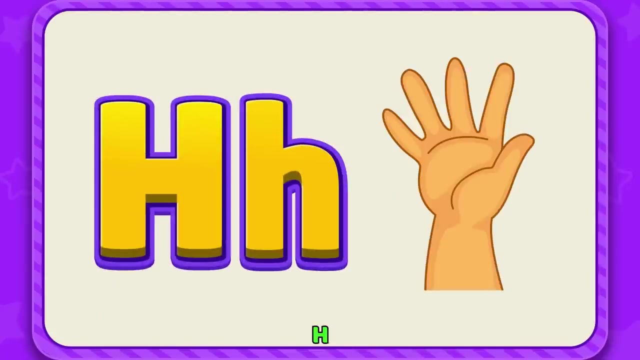 F is for fairy F, F. fairy F F. fairy A F. fairy G is for glasses G, G glasses G, G glasses G glasses. H is for hand, H, H hand. H, H hand, H, H hand. 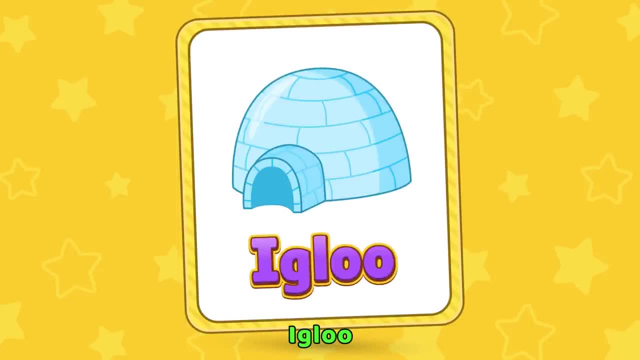 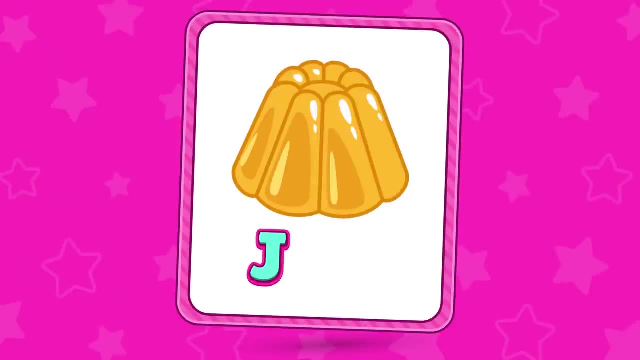 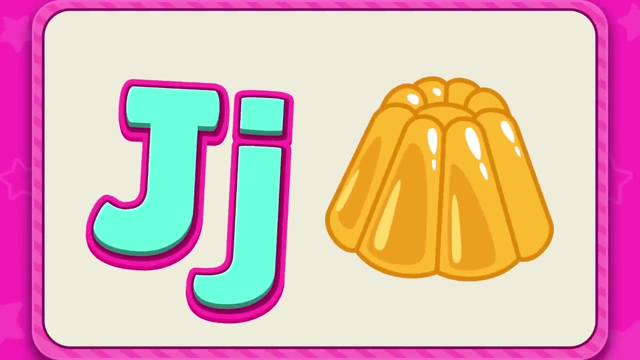 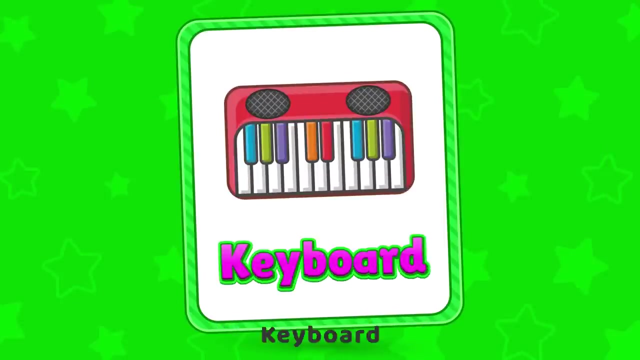 I is for igloo I, I, igloo I, I, igloo I. igloo J is for jelly J, J, jelly J, J, jelly J, jelly. K is for keyboard K K keyboard. K K keyboard, K keyboard. 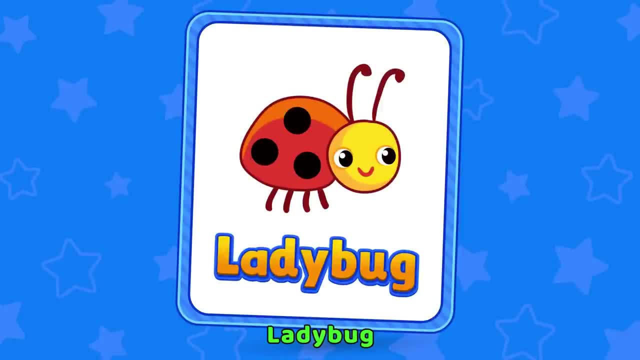 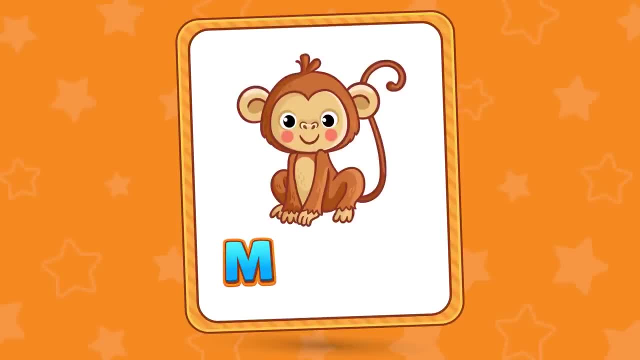 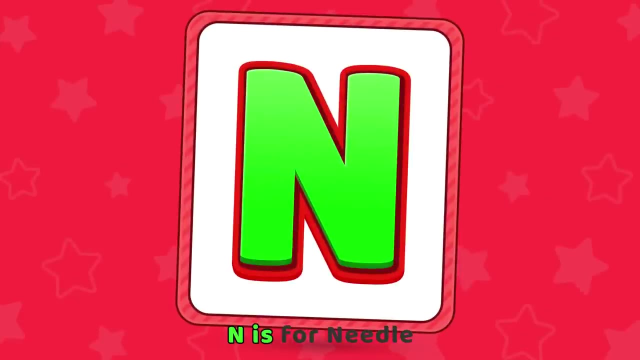 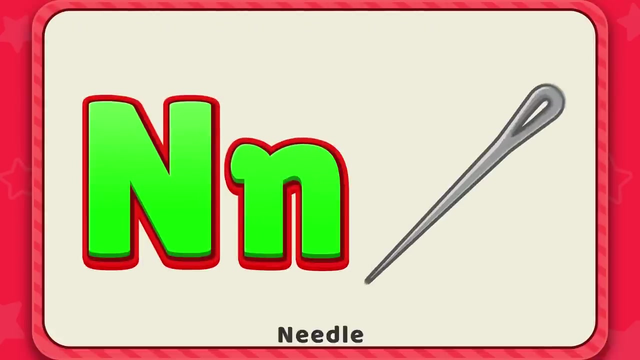 L is for ladybug U U ladybug U U ladybug L. ladybug M is for monkey U U monkey U U monkey M. monkey N is for needle U U needle U U needle N needle. 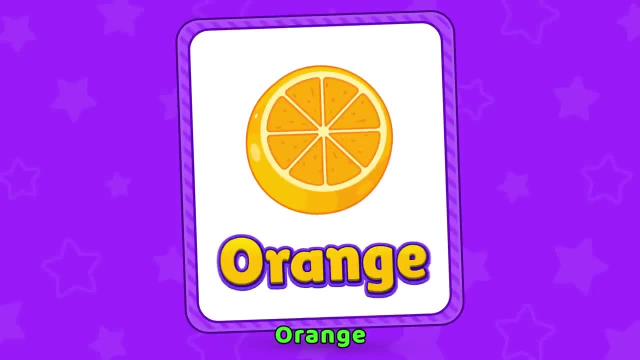 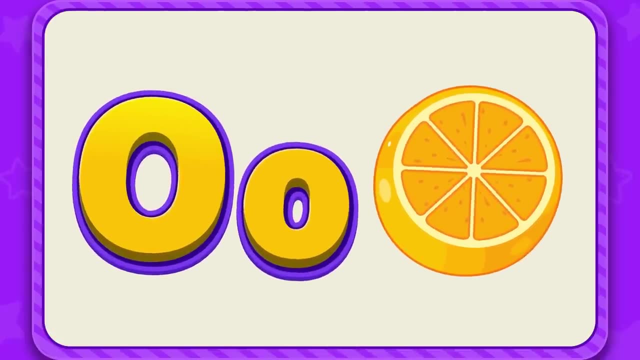 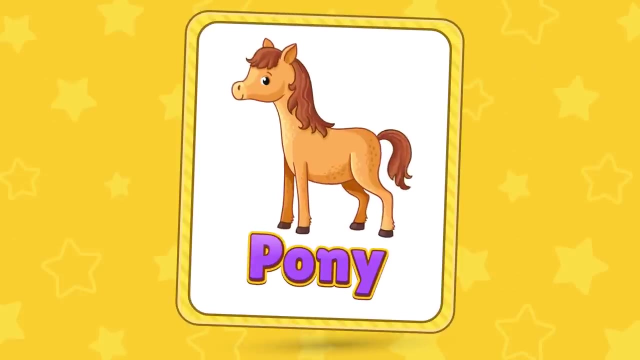 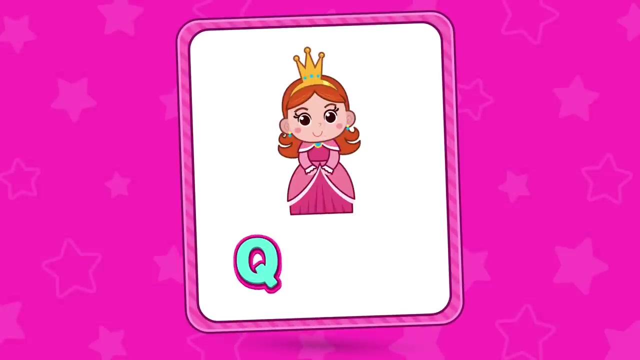 O is for orange O O, orange O O, orange O orange. P is for pony P, P, pony, P, P, pony, P pony. Q is for queen, Q, Q, queen, Q, Q, queen, Q queen. 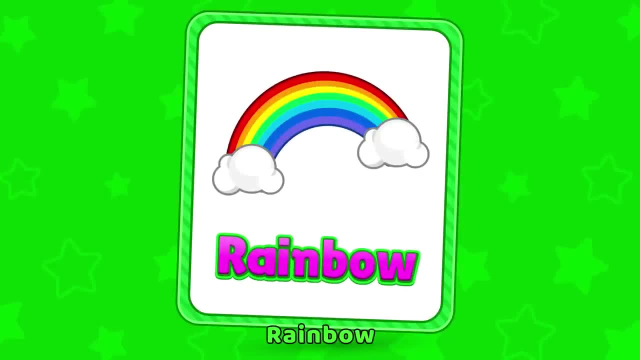 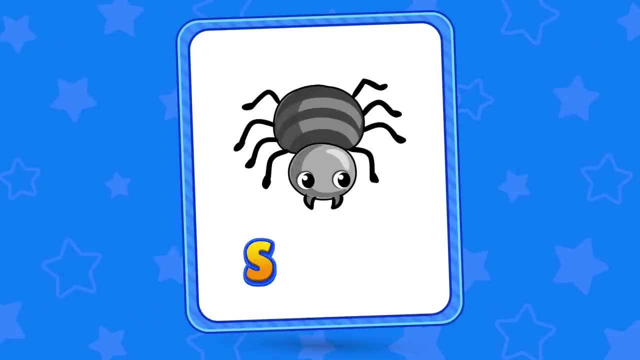 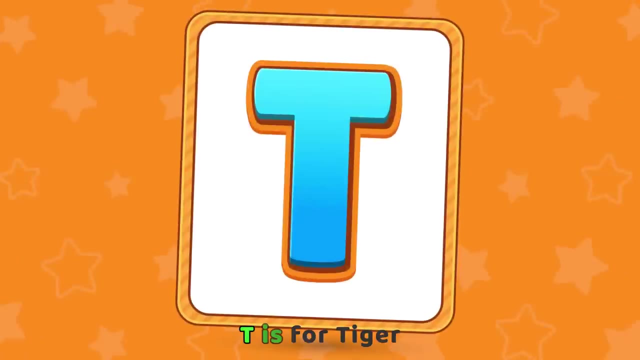 R is for rainbow R R. rainbow R R rainbow R. rainbow S is for spider S S, spider S S, spider S. spider D is for tiger T t tiger, T t tiger. 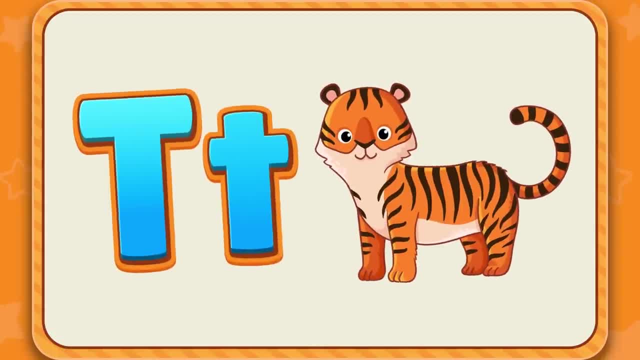 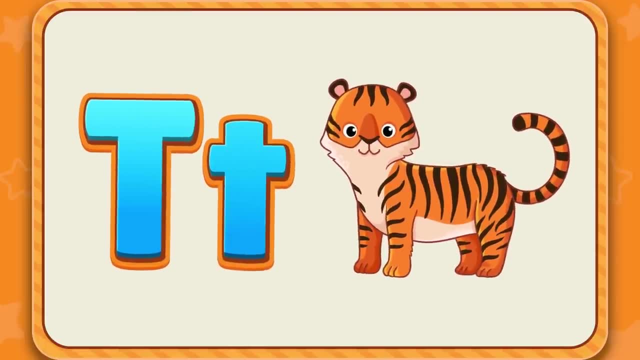 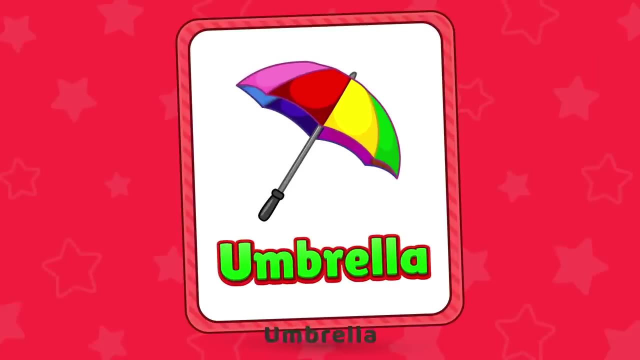 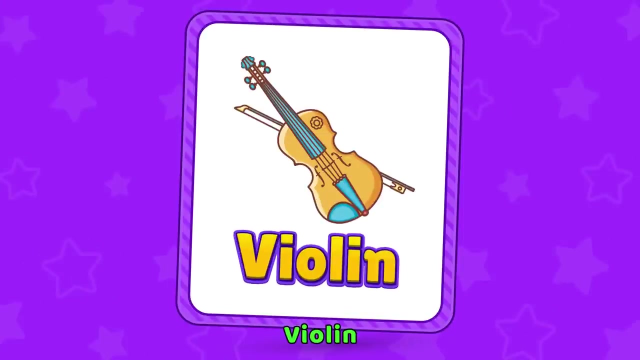 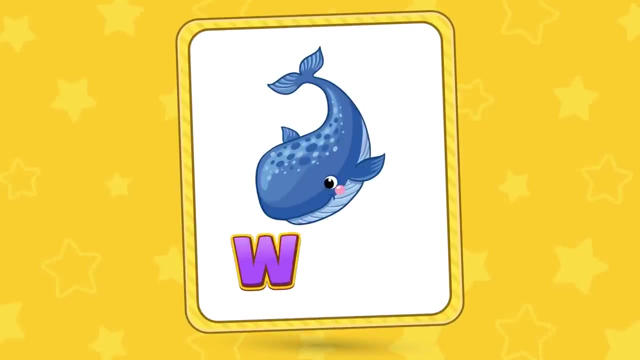 C tiger. U is for umbrella A a. umbrella A a. umbrella U. umbrella V is for violin V v violin V v. violin V violin. W is for whale: W w whale, W w whale. 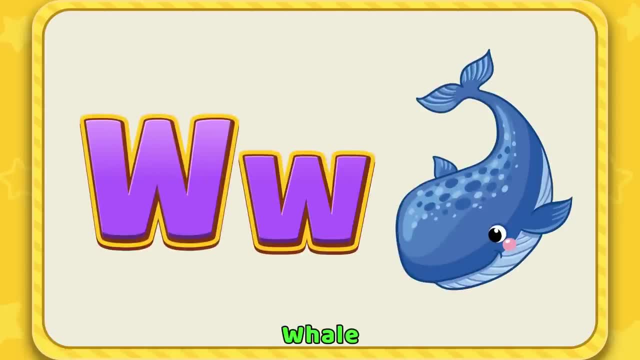 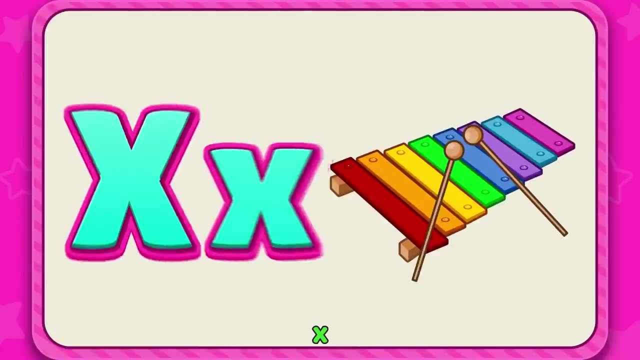 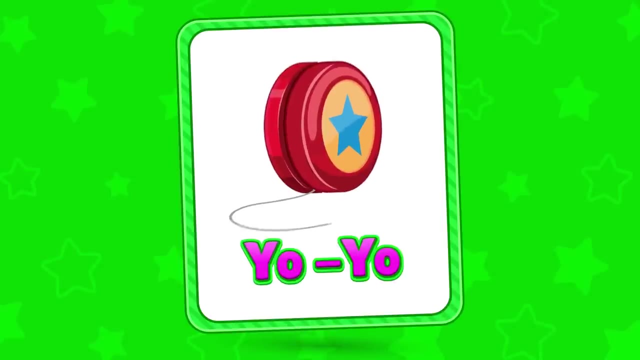 W w whale W. whale X is for xylophone Z z xylophone Z z xylophone X. xylophone Y is for yo-yo U u, yo-yo Y y, yo-yo. 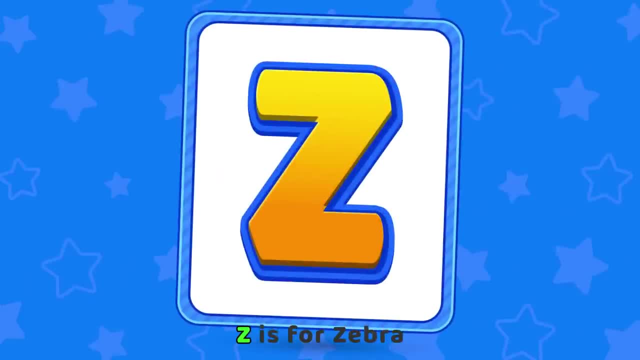 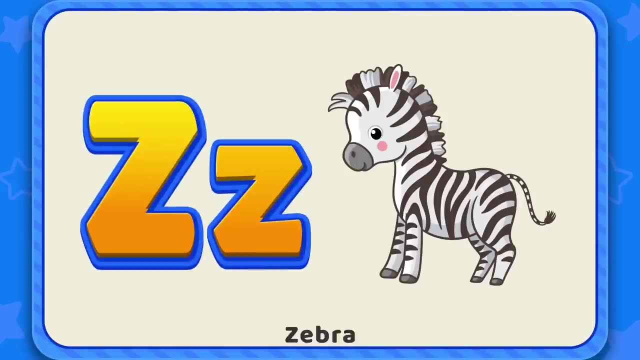 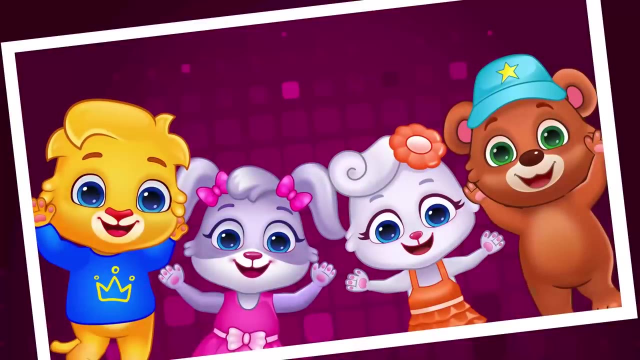 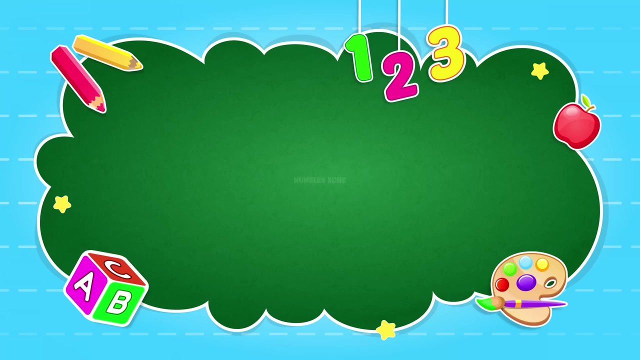 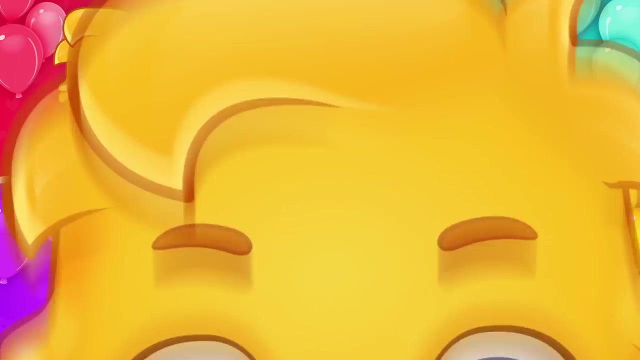 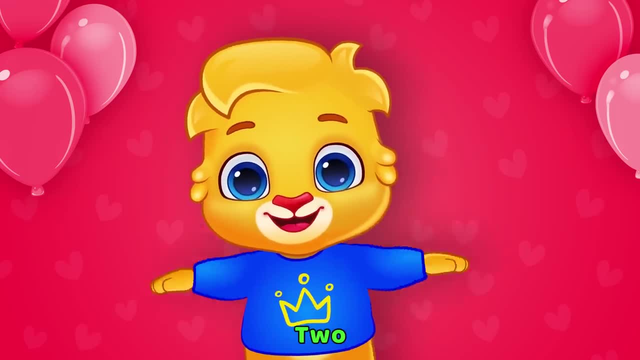 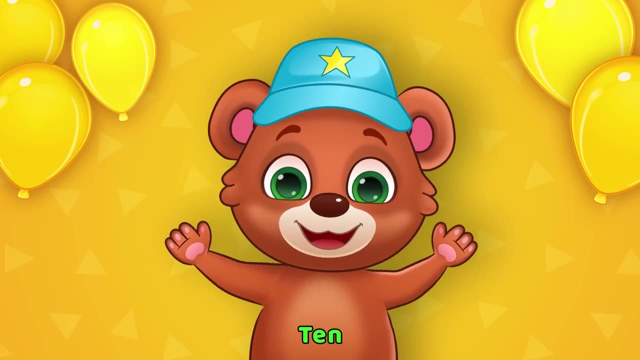 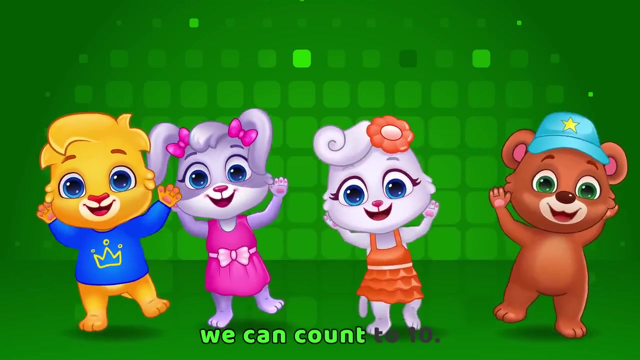 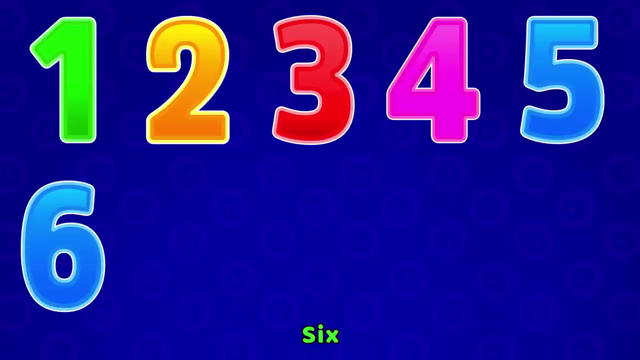 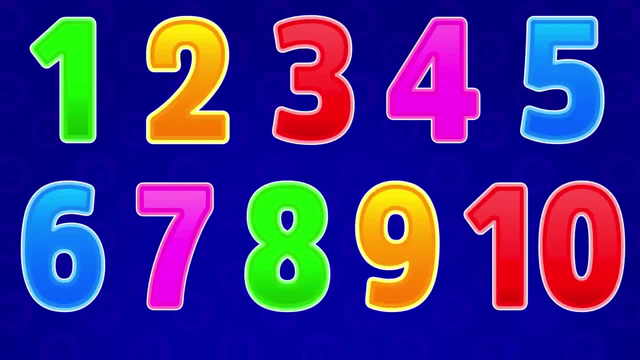 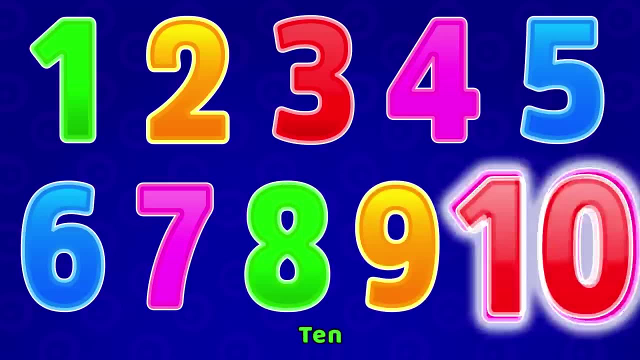 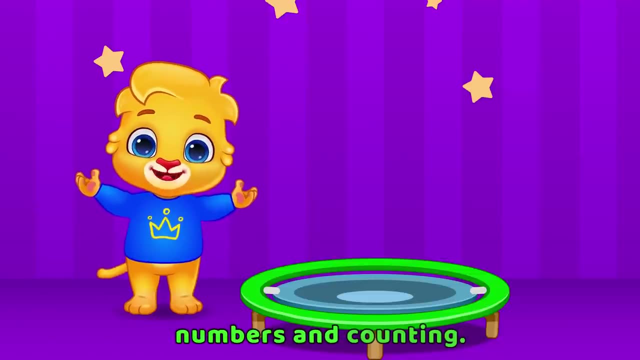 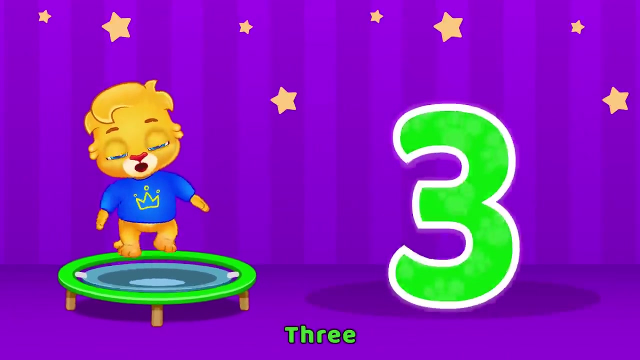 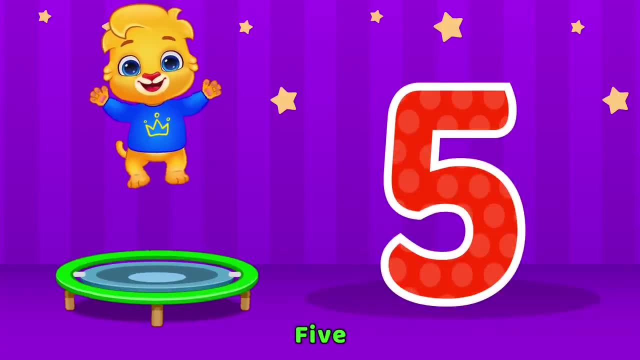 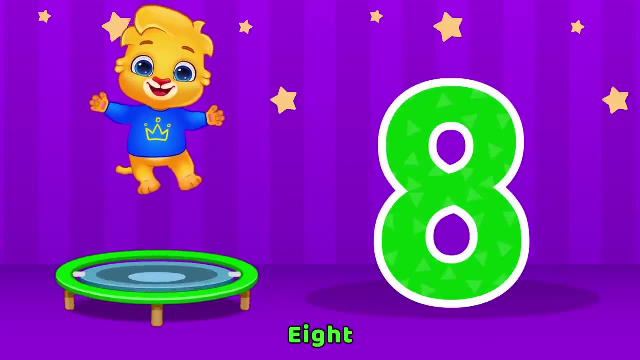 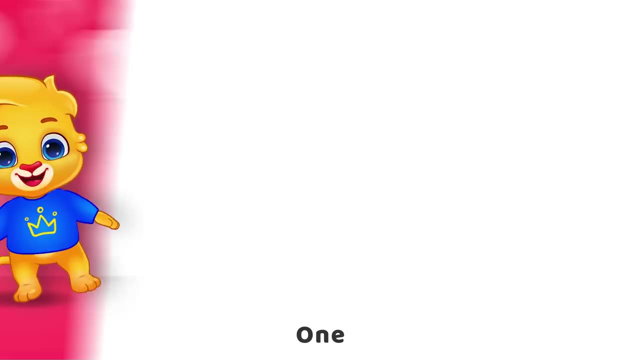 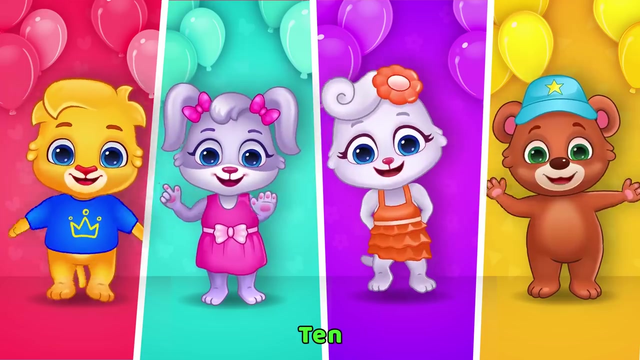 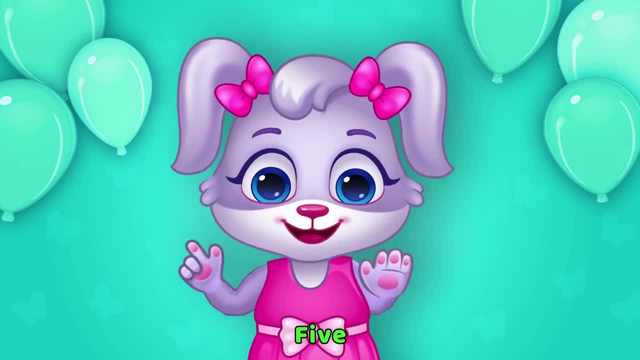 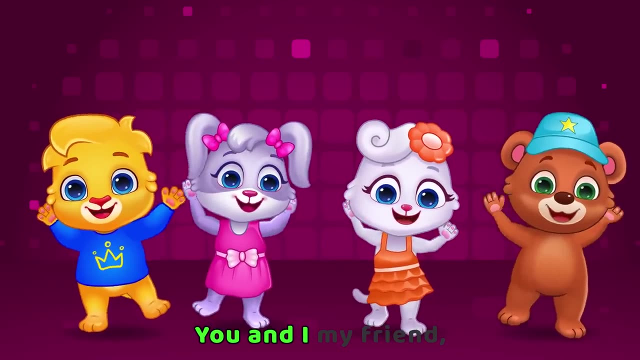 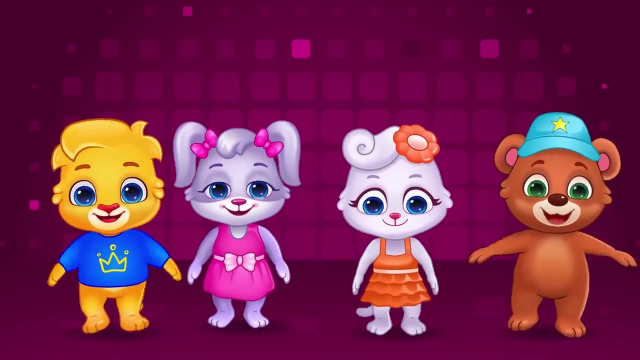 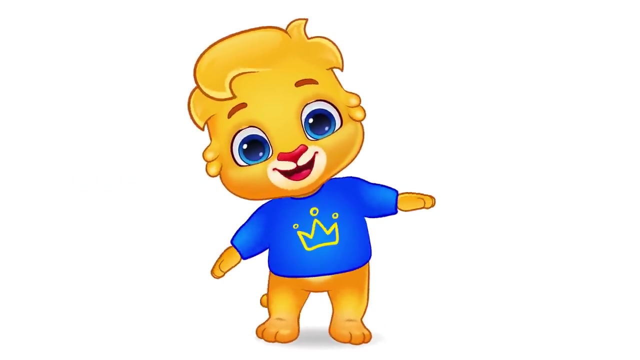 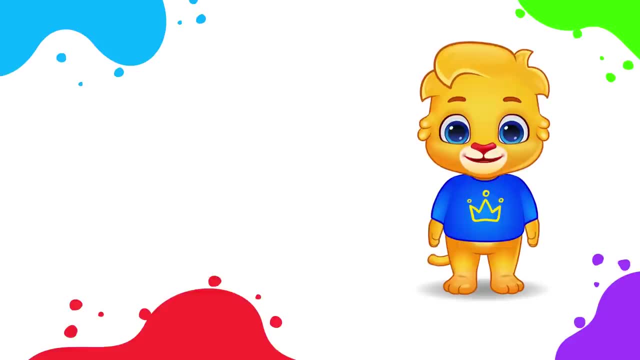 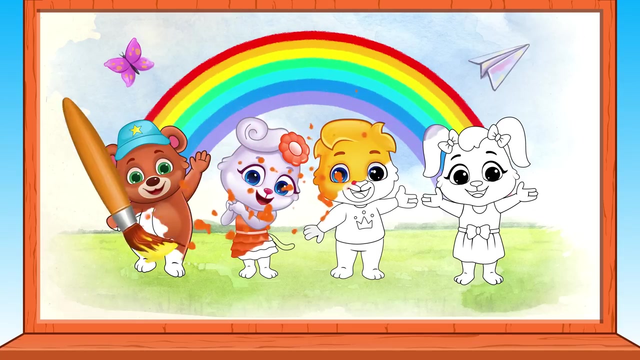 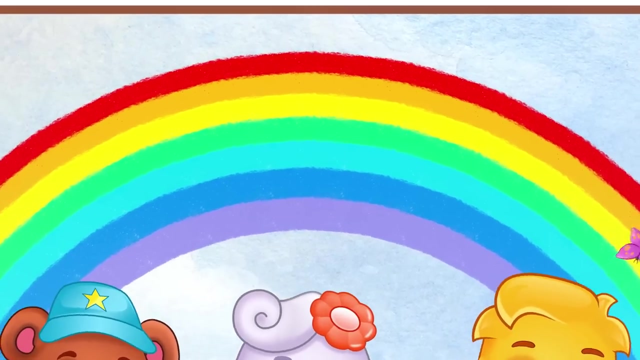 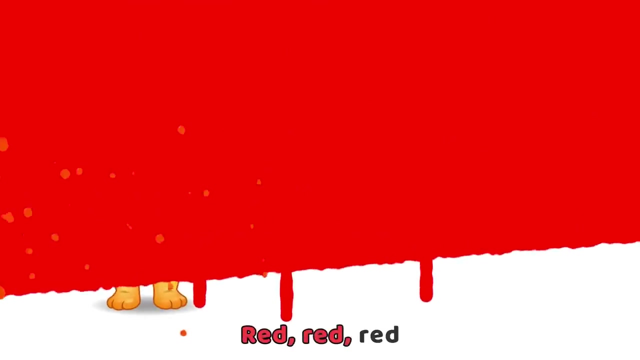 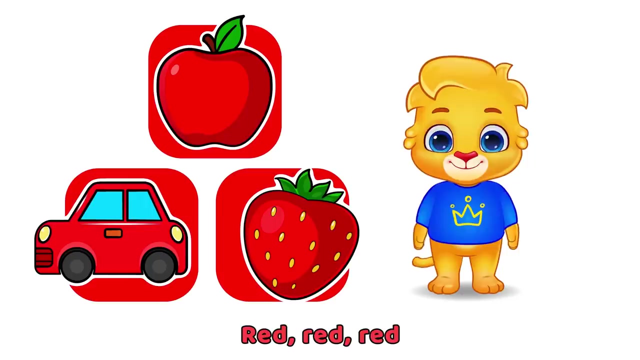 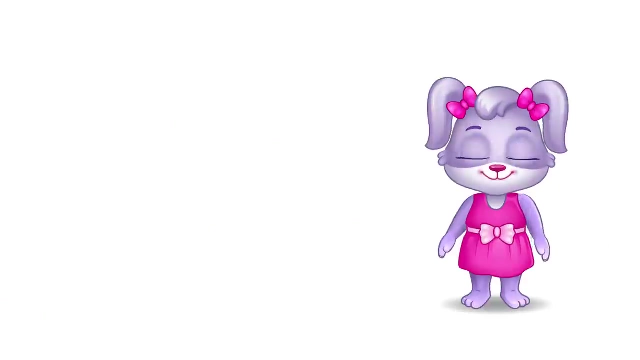 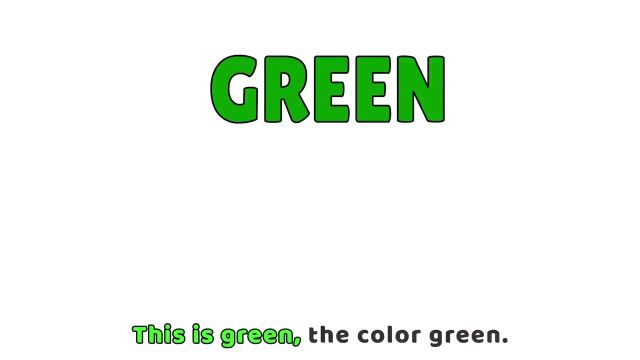 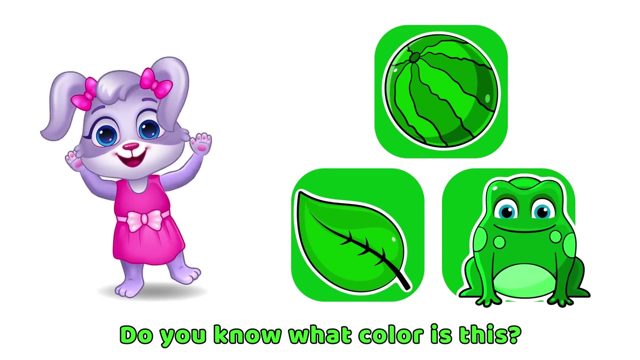 Z zebra, Z zebra. Hi, I'm Lucas, and guess what we're doing today? We're going to learn colors. This is red. the color red, red, red. Do you know what color this is? this is red. Green, green: Do you know what color this is? this is green. 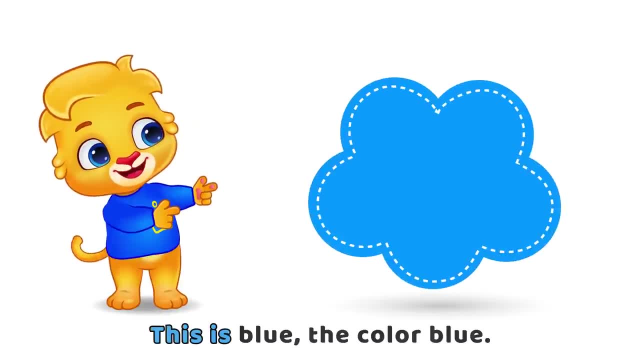 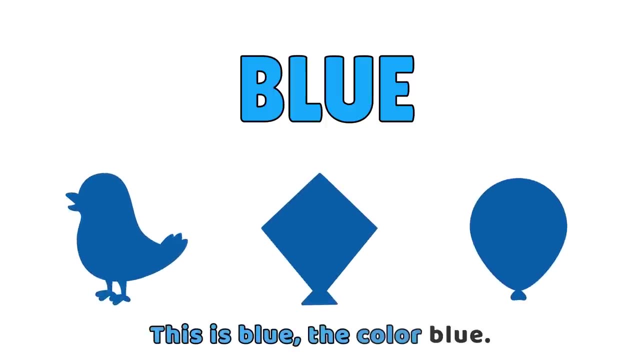 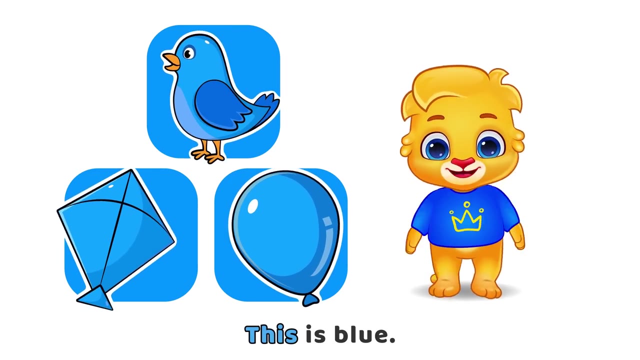 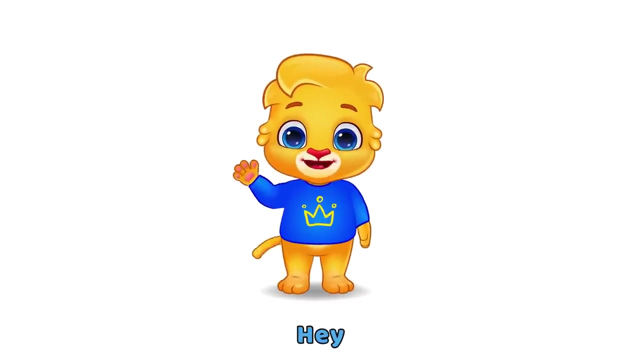 This is blue: the color blue, blue, blue, blue. This is blue, the color blue, blue, blue, blue. Do you know what color this is? This is blue. Hey, Do you know what color shirt I'm wearing? Hmm, it's the color blue. 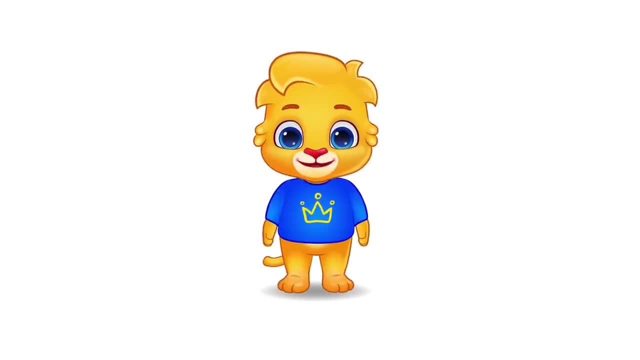 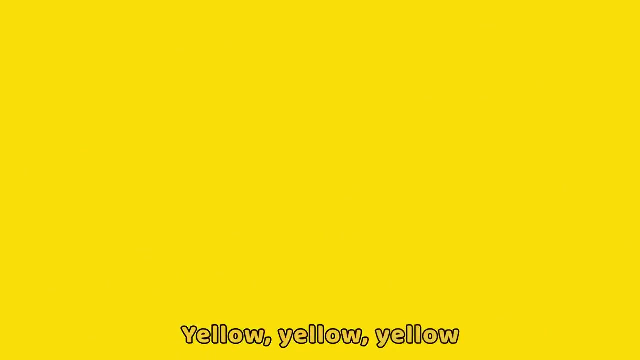 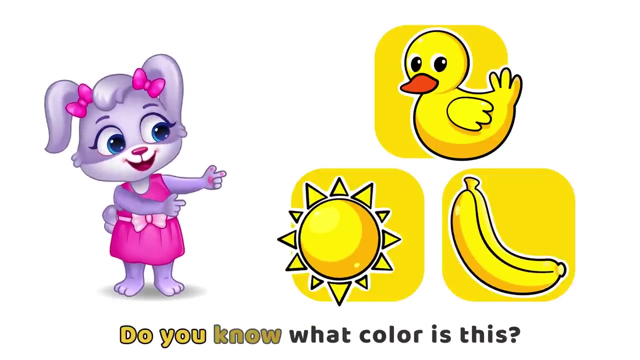 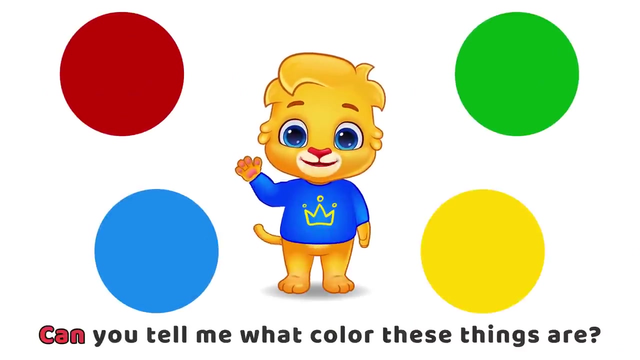 Blue. Great, This is yellow. the color yellow, yellow, yellow, yellow. This is yellow. the color yellow, yellow, yellow, yellow. Do you know what color this is? This is yellow. Hey, Can you tell me what color these things are? 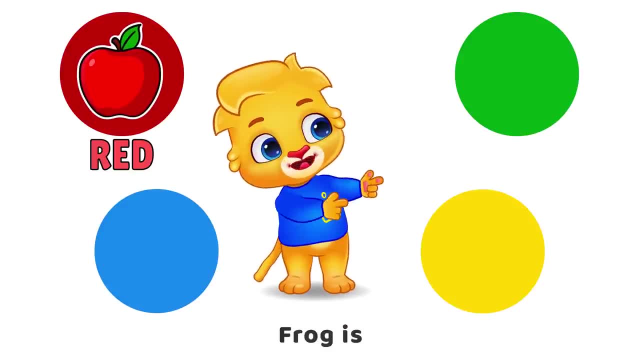 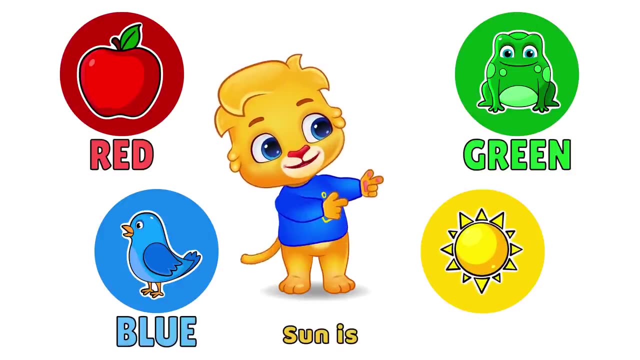 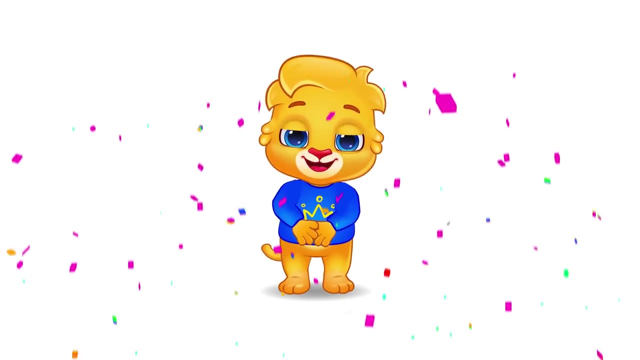 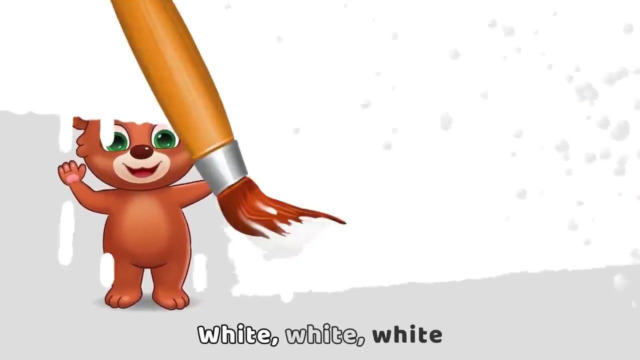 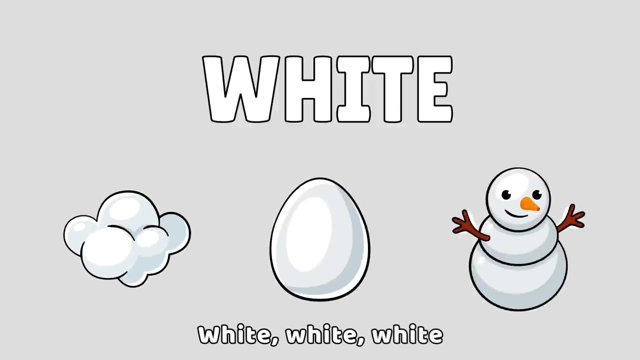 Apple is red, frog is green, bird is blue, sun is yellow. Great Woohoo. This is white. the color white, white, white, white. This is white. the color white, white, white, white. Do you know what color this is? This is white. 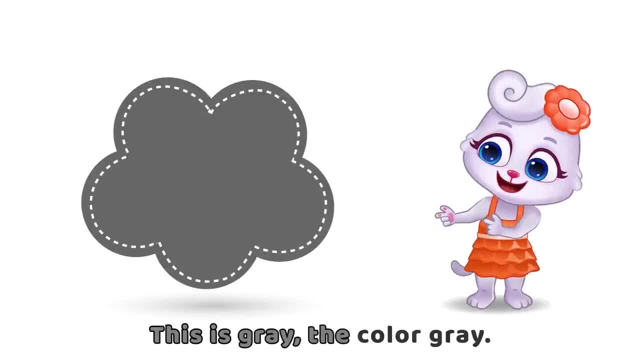 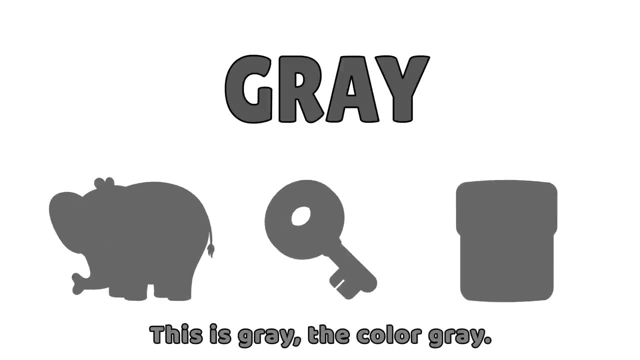 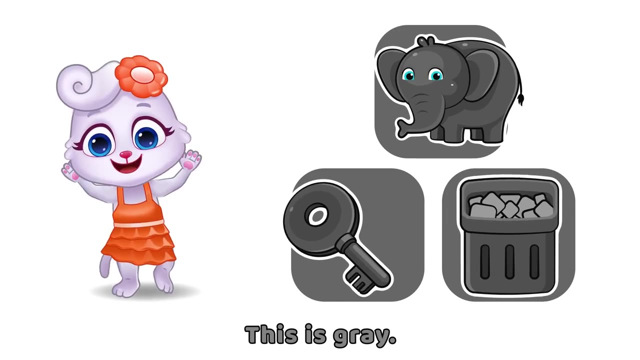 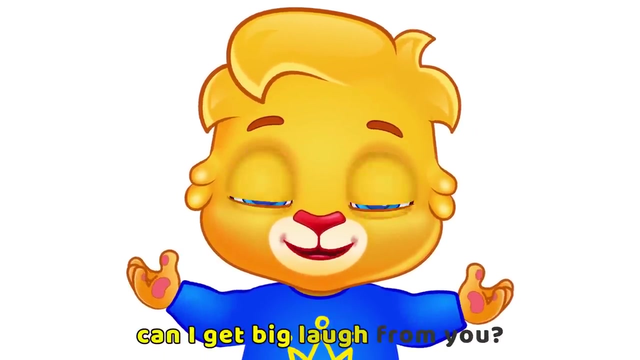 This is gray, the color gray, gray, gray, gray. This is gray, the color gray, gray, gray, gray. Do you know what color this is? This is gray. Hey, my friend, Can I get a big laugh from you? 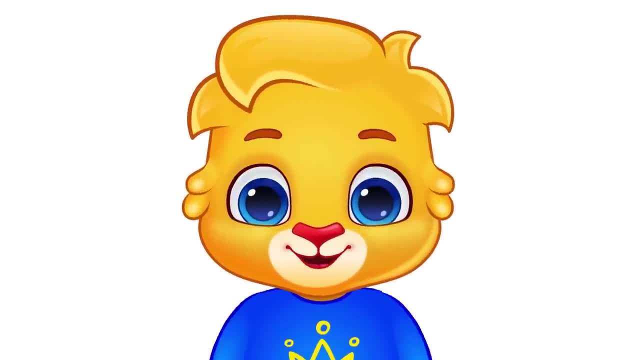 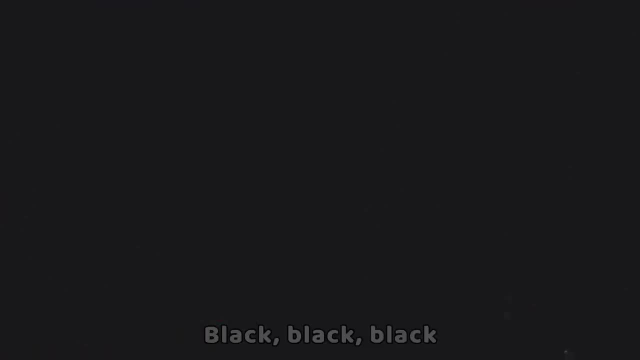 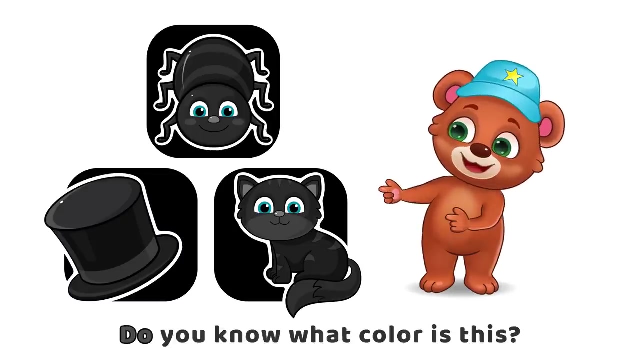 Ha, ha, ha ha. This is black. the color black, black, black, black. This is black. the color black, black, black, black. Do you know what color this is? This is black. This is red. the color green: green, green, green. 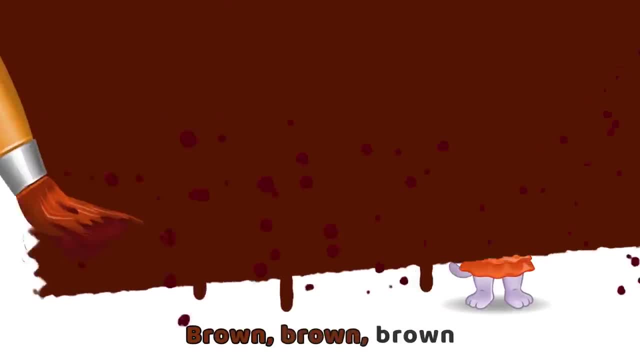 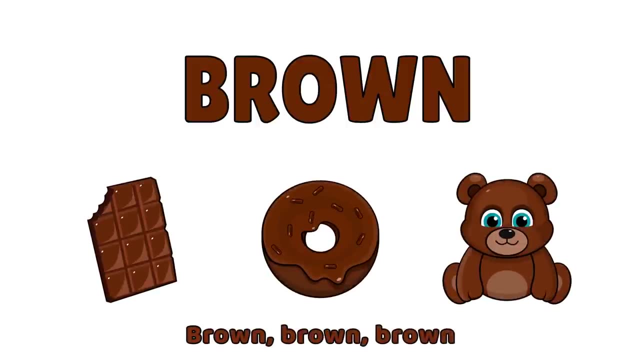 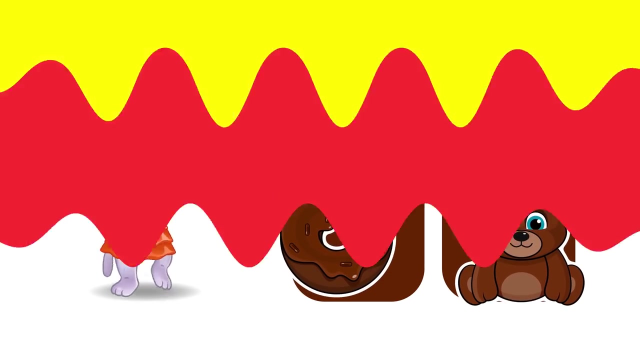 This is brown, the color brown, Brown, brown, brown. This is brown, the color brown, Brown, brown, brown. Do you know what color this is? This is brown. Hey, what color are these things? Do you know? 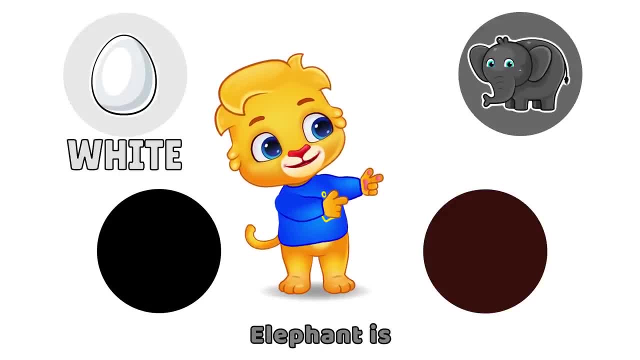 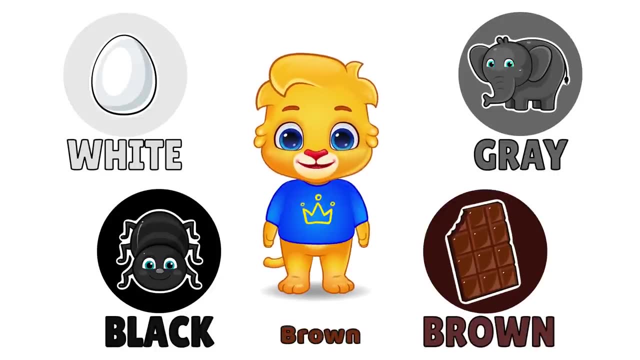 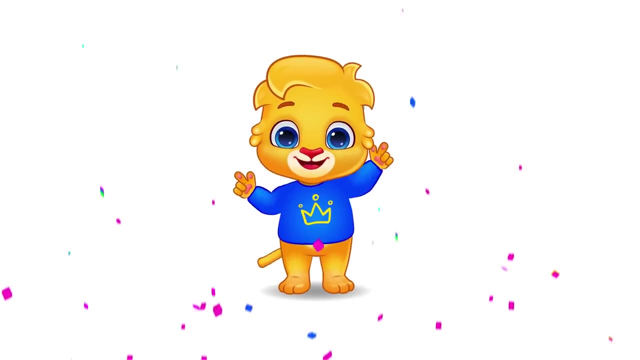 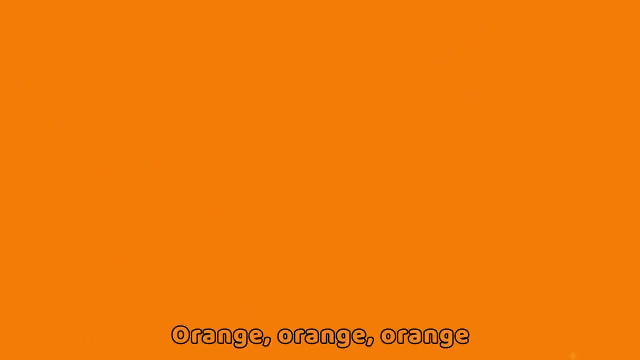 Egg is White, Elephant is Gray, Spider is Black, Chocolate is Brown, Superb, Woohoo. This is orange, the color orange. Orange, orange, orange. This is orange, the color orange, Orange, orange, orange. 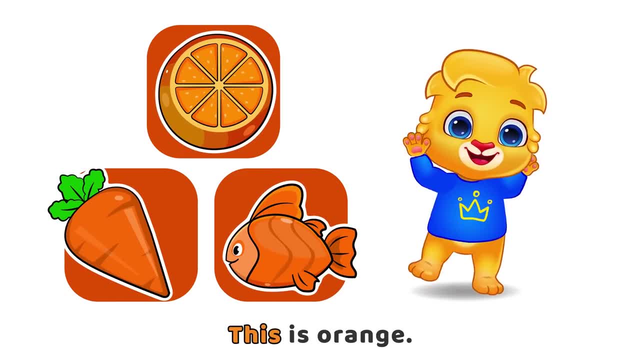 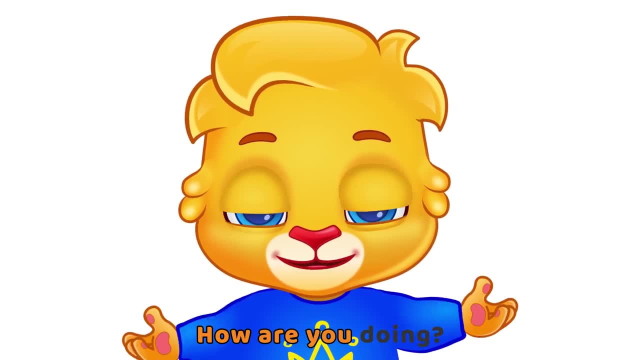 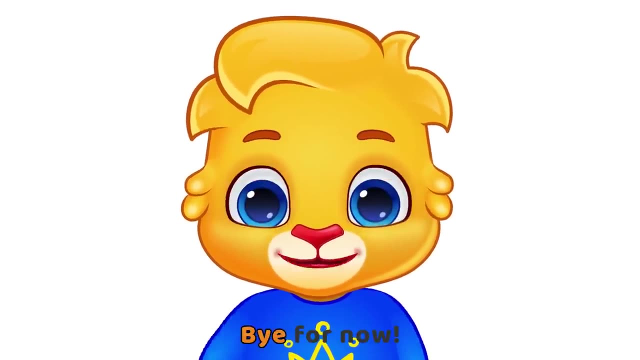 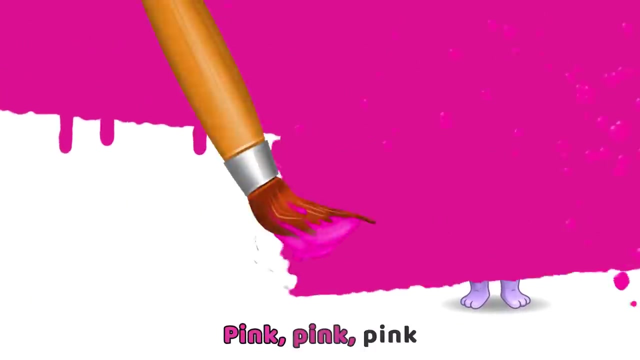 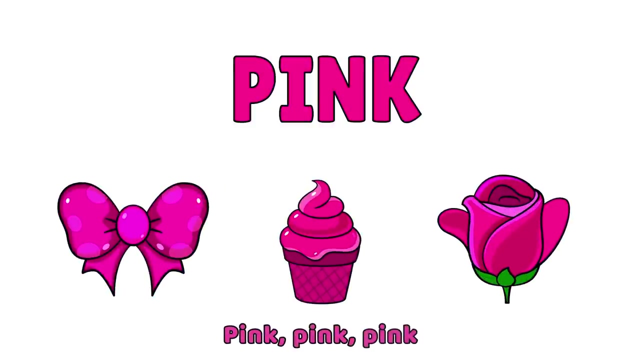 Do you know what color this is? This is orange. Ah, what color is orange? APPLY Hi. how are you doing? Wanted to say hi, Bye for now. This is pink, the color pink. Pink, pink, pink. This is pink, the color pink. 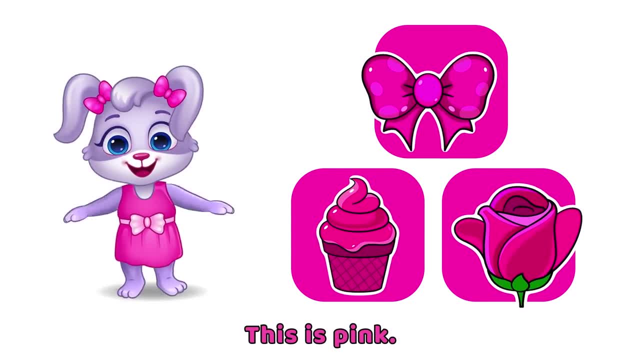 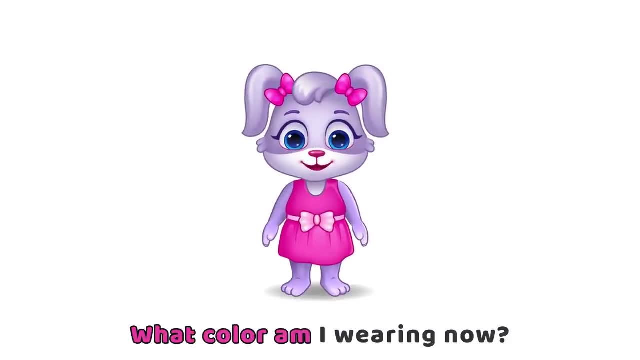 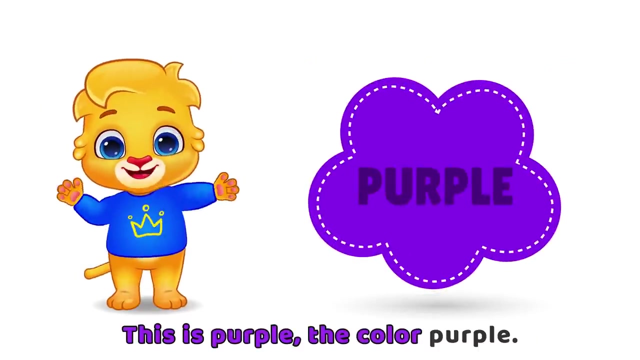 Pink, pink, pink. Do you know what color this is? This is pink. Hey, What color am I wearing now? That's right, It's the color pink, Pink. Well done, This is purple, the color purple, purple, purple, purple. 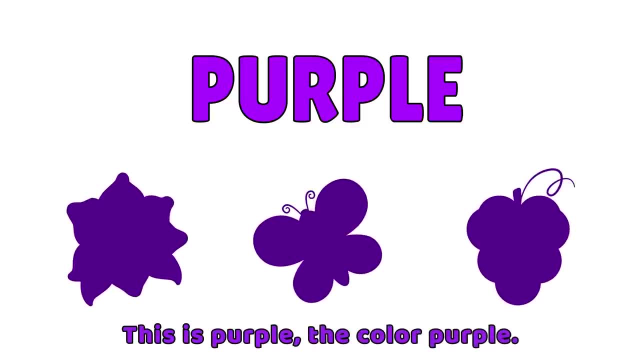 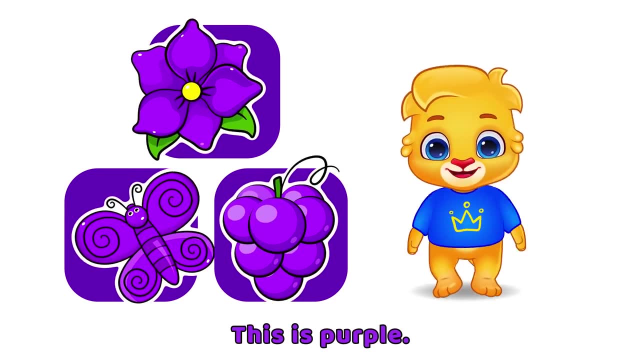 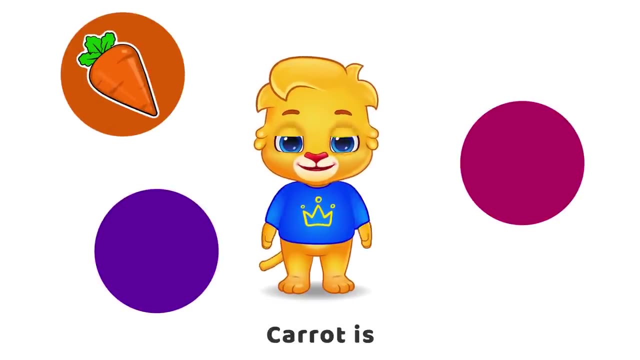 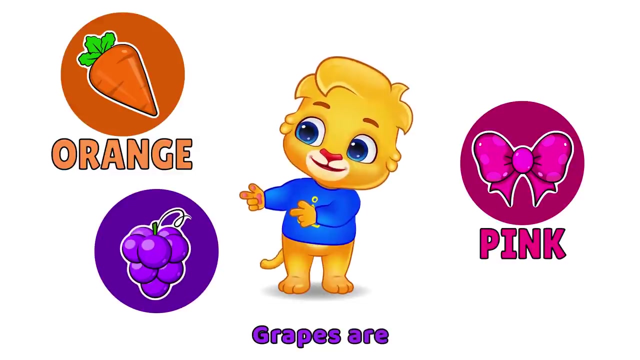 This is purple, the color purple, purple, purple, purple. Do you know what color this is? This is purple. Hey, Can you tell me what color these things are? Carrot is orange, Bow is pink, Grapes are purple. 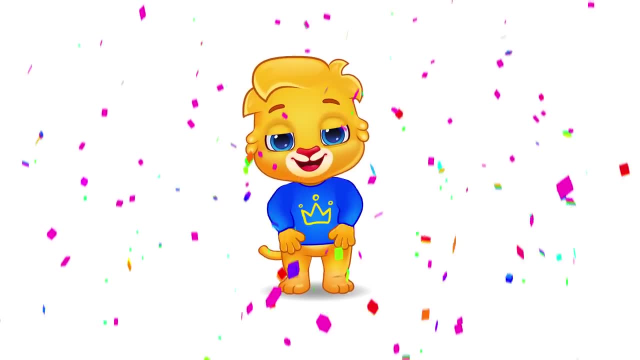 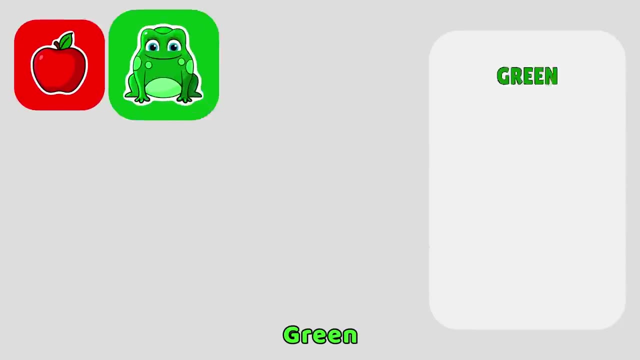 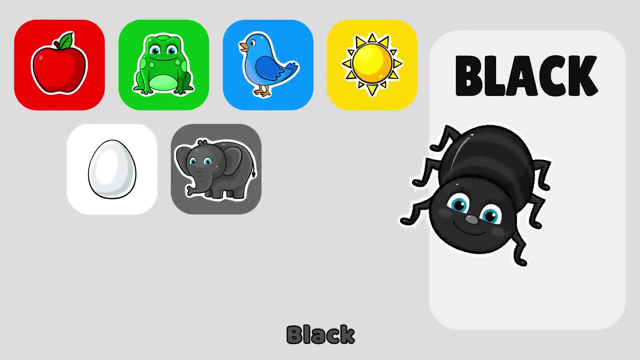 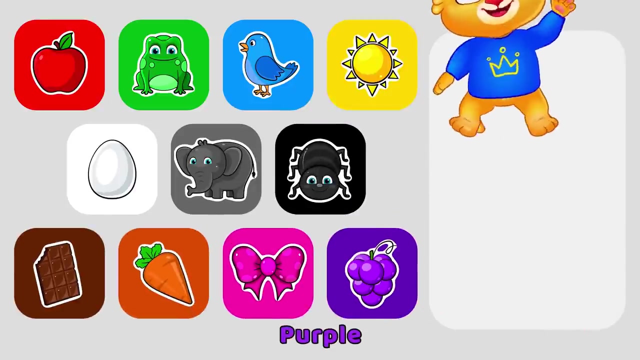 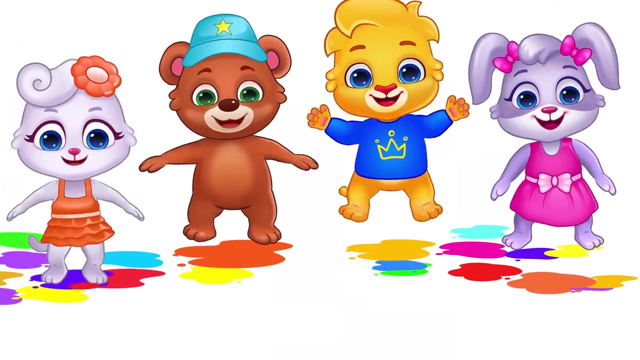 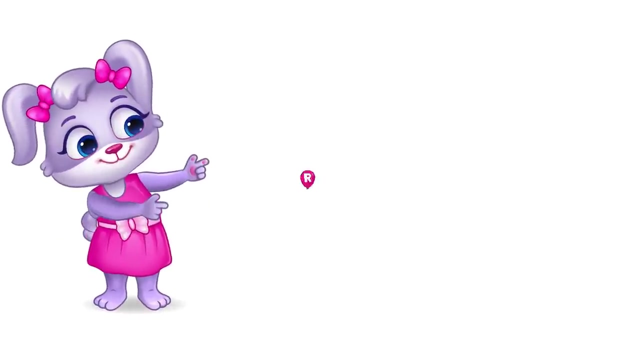 Awesome, Woohoo. Red, Green, Blue, Yellow, White, Gray, Black, Brown, Orange, Pink, Purple, White. This is pink. We are the pink hair. Hi, I'm Ruby. It's spelt R-U-B-Y: Ruby, Ruby, Ruby, Ruby. 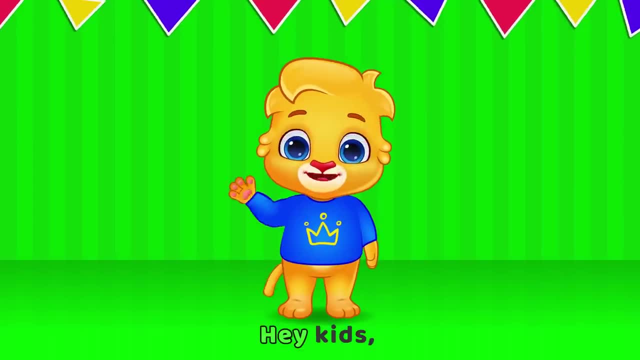 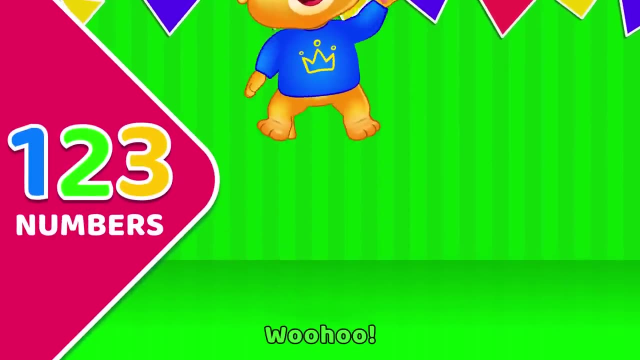 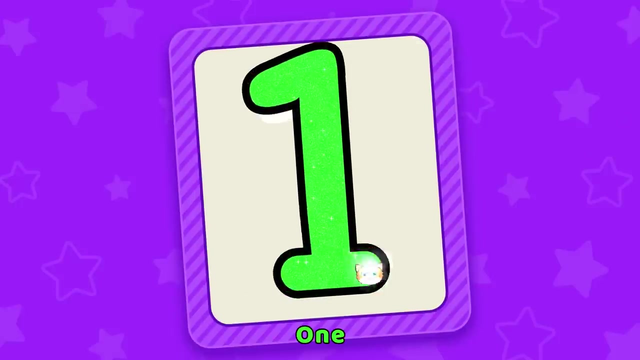 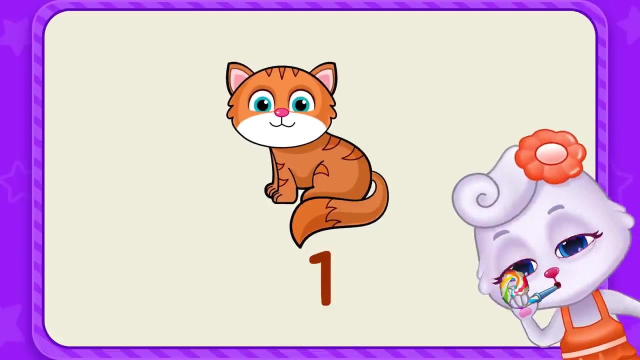 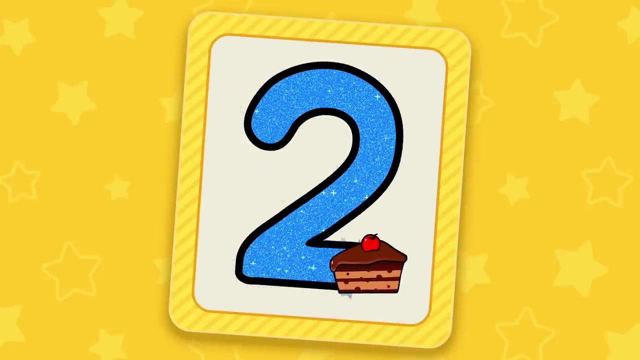 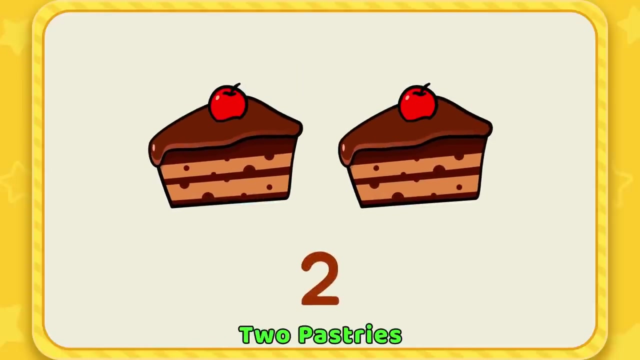 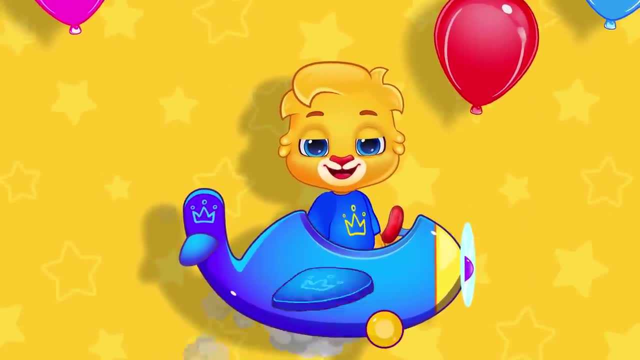 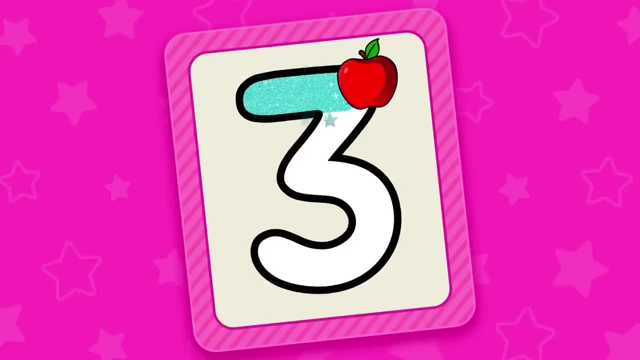 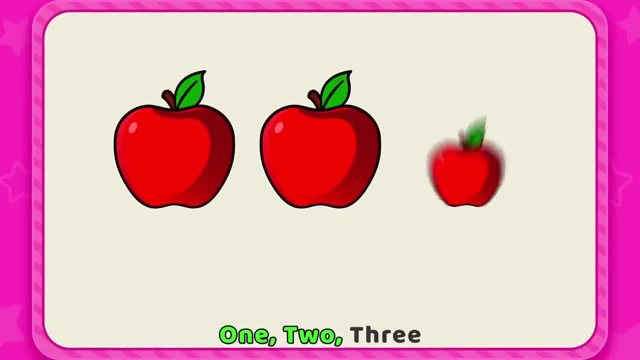 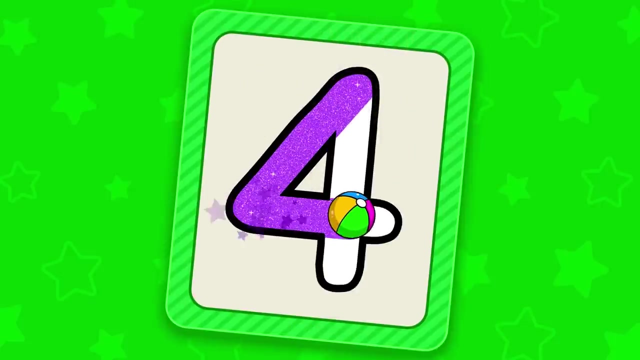 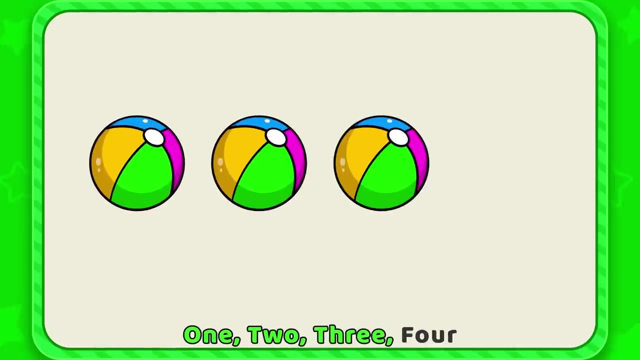 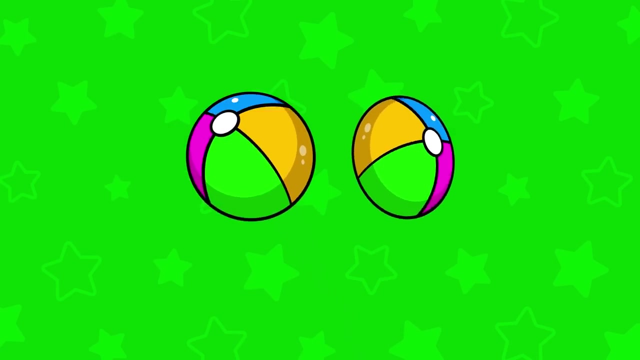 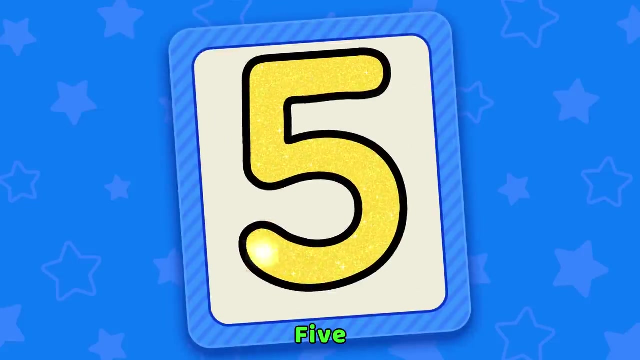 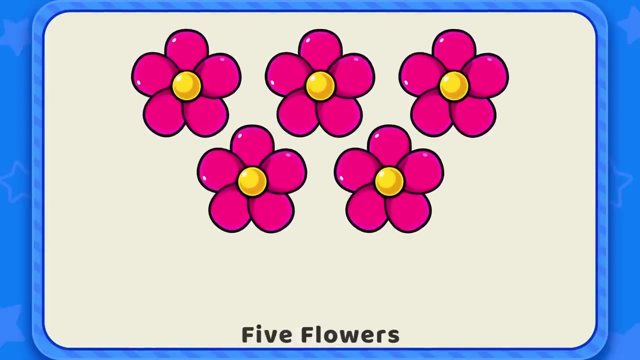 Keep learning, keep smiling. Three, Three, One, two, three, Three apples. Four One, two, three, four, four balls, Five, Five. One, two, three, four, five, Four, Five flowers. 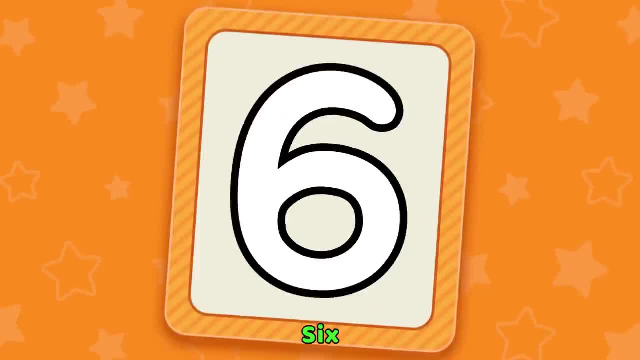 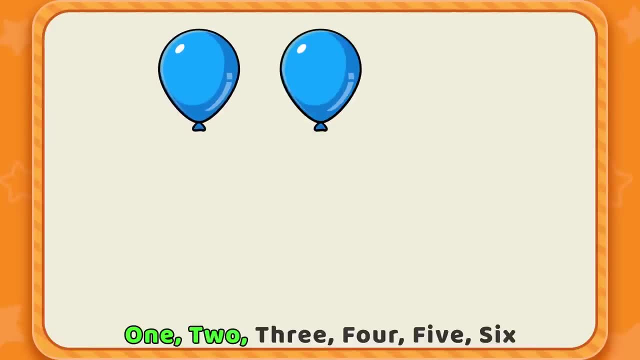 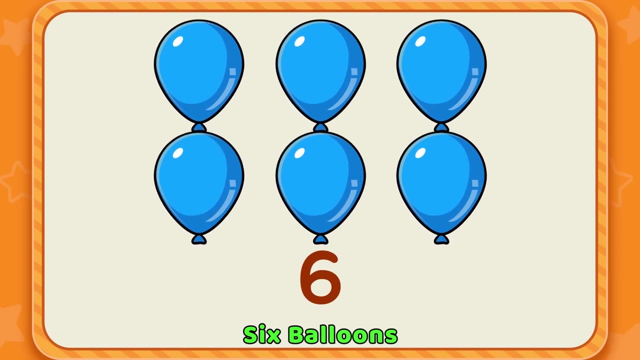 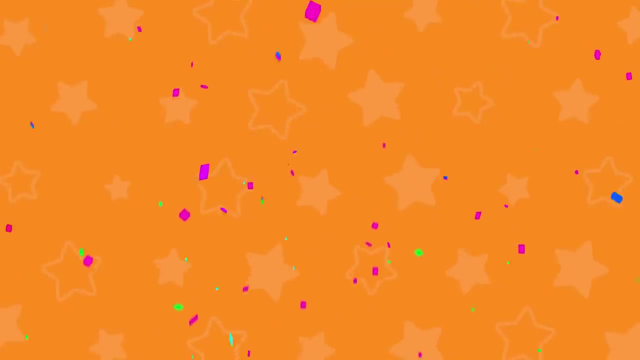 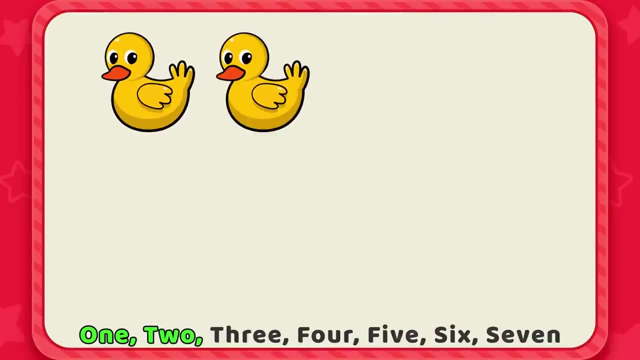 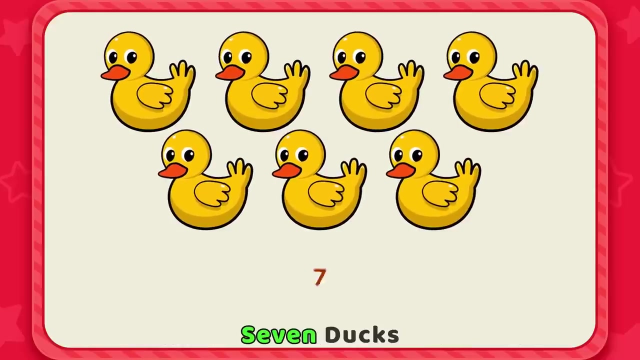 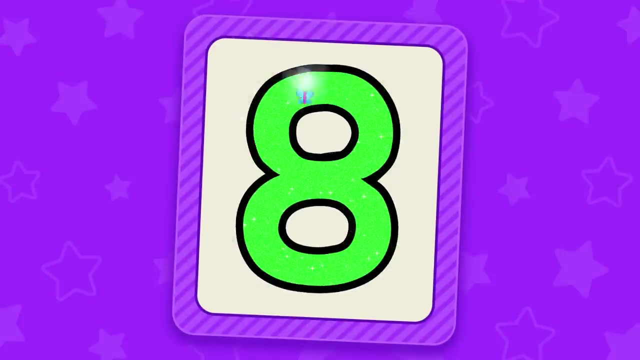 Wonderful. Six, Six, One, two, three, four, five, six, Six, six balloons. Seven, seven. One, two, three, four, five, six, seven, Seven, ducks Eight. Hello, What's this? 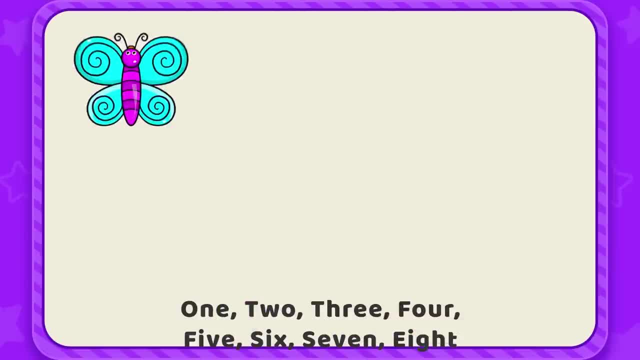 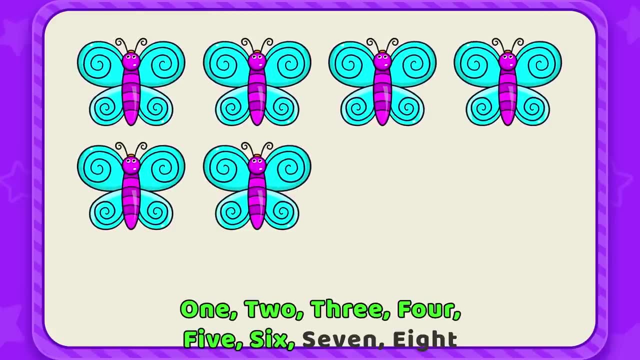 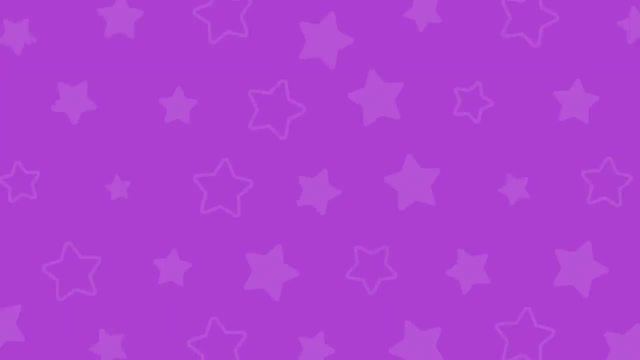 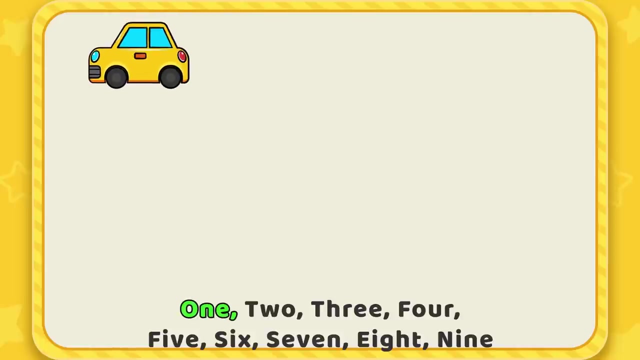 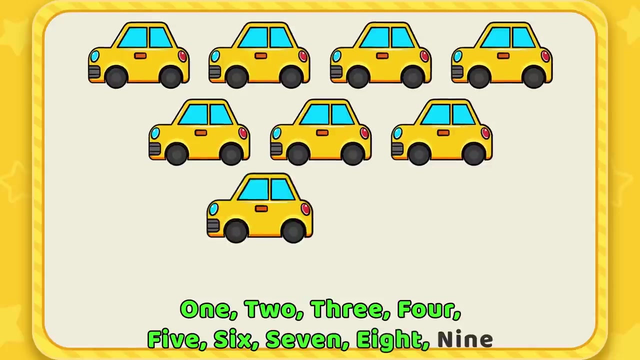 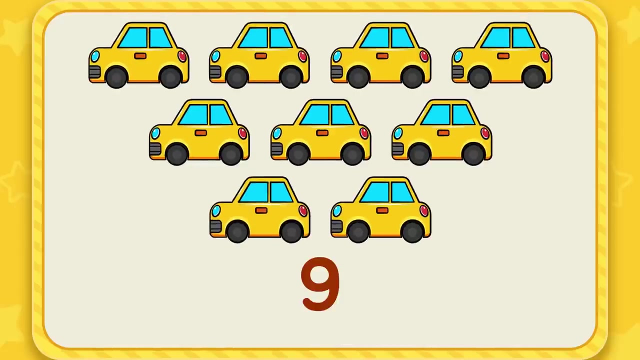 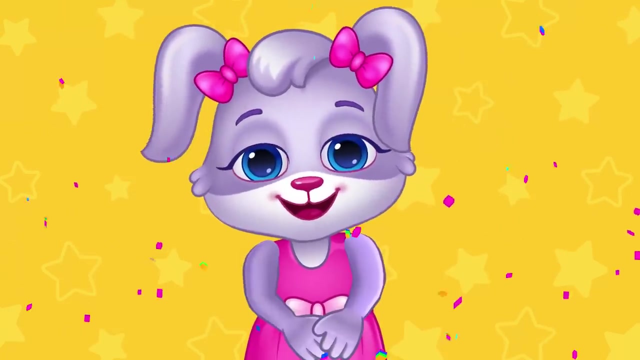 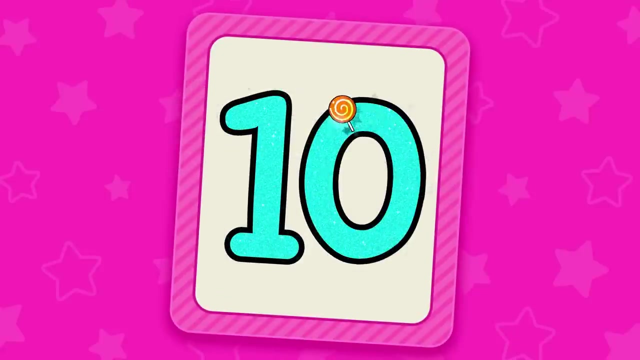 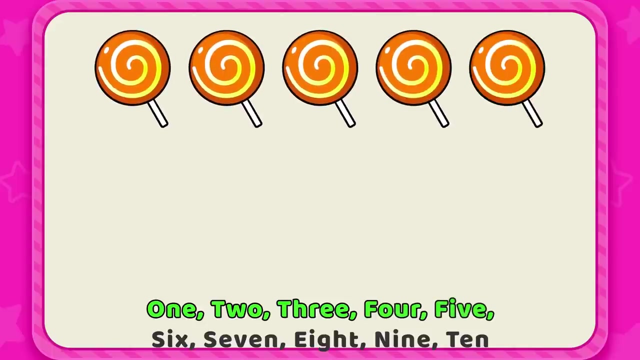 Eight: One, two, three, four, five, six, seven, eight, Eight butterflies: Nine: Nine: One, two, three, four, five, six, seven, eight, nine, Nine cars: Ten: One, two, three, four, five, six, seven, eight, nine, ten. 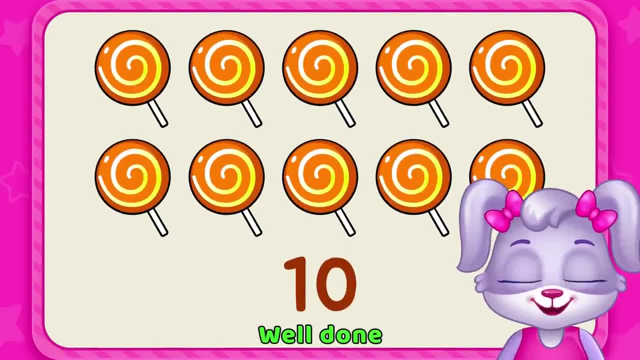 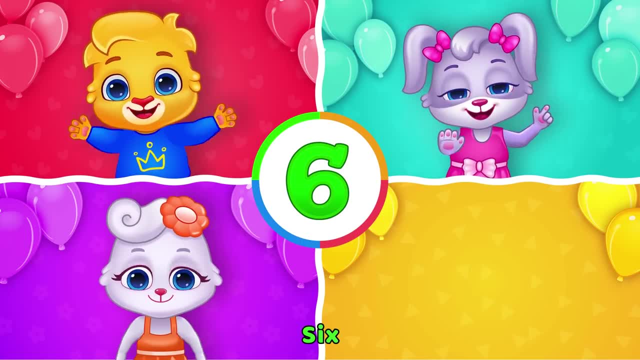 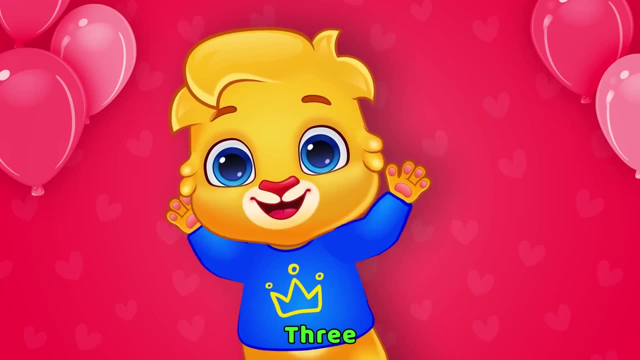 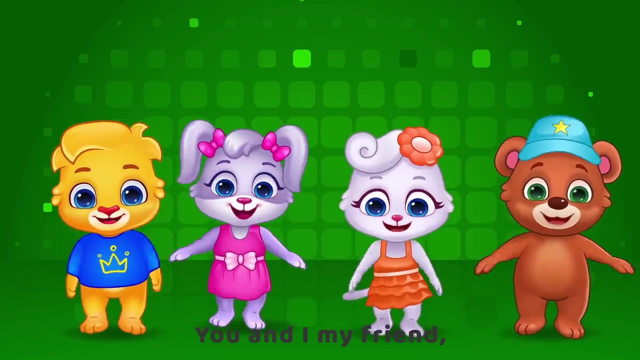 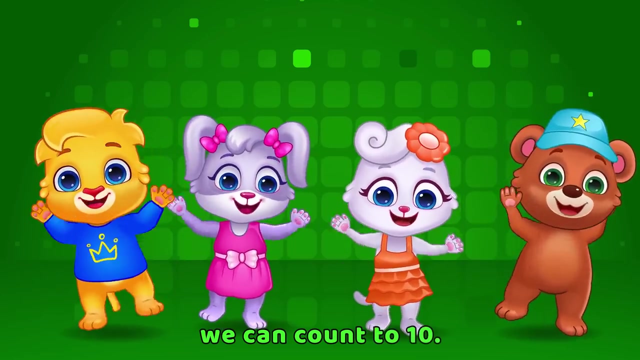 Ten candies Well done. One, two, three, four, five, six, seven, eight, nine, ten. One, two, three, four, five, six, seven, eight, nine and ten, You and I, my friend, we can count to ten. 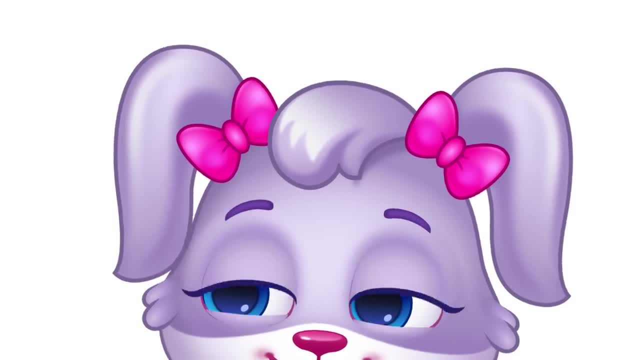 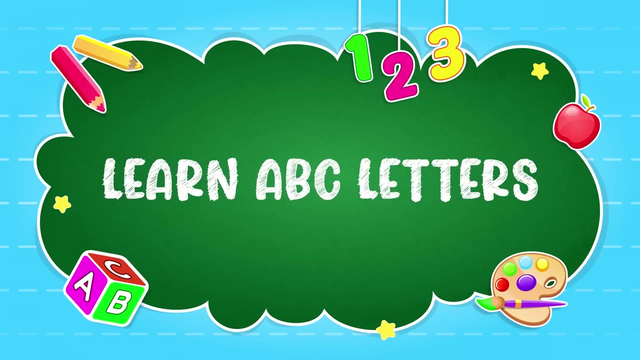 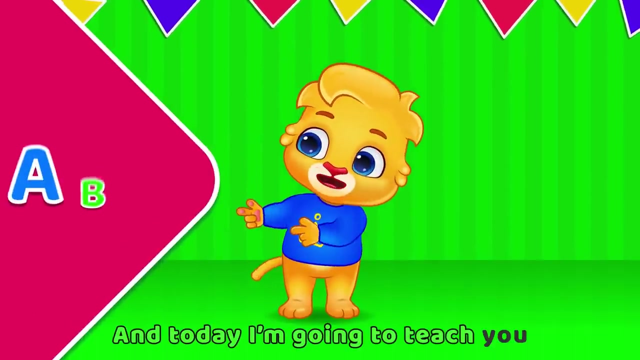 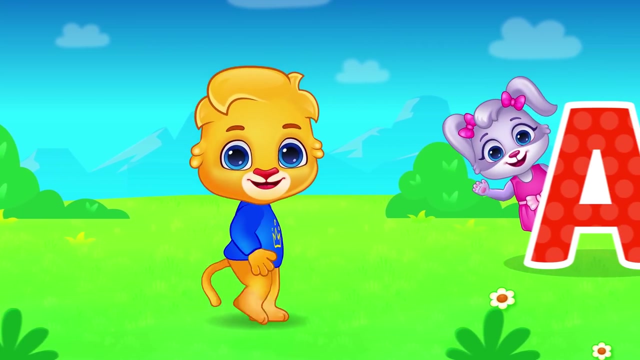 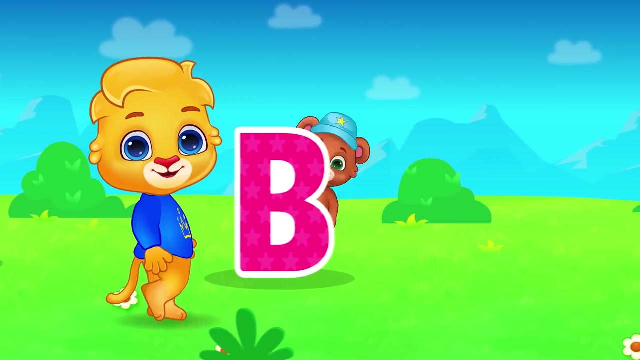 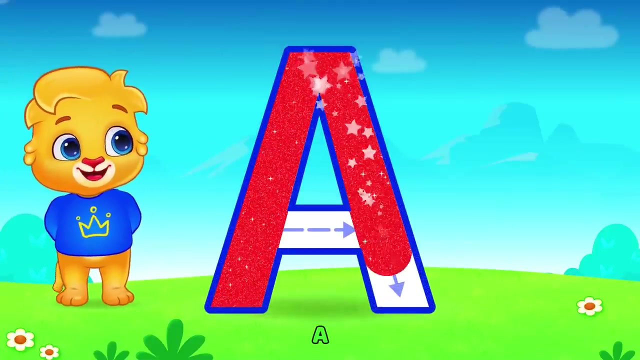 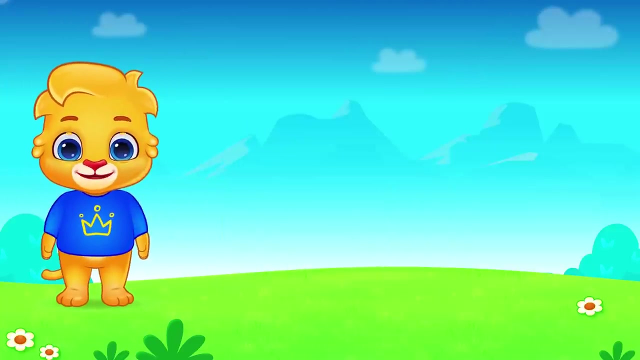 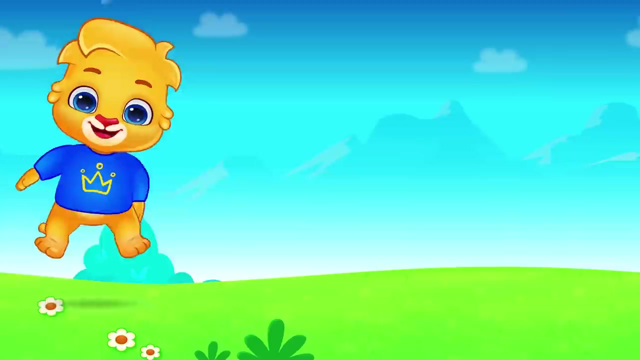 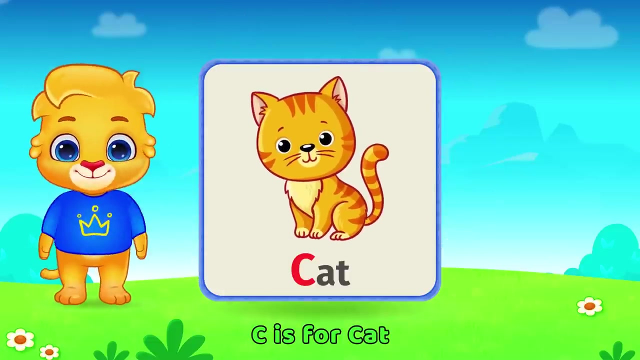 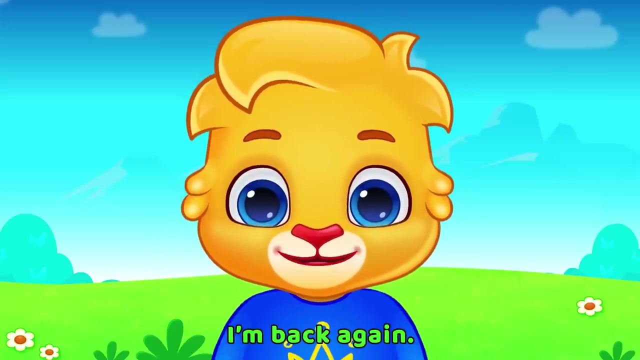 You and I, my friend, we can count to ten. Hello, Let's go. A- A is for apple, B, B is for ball, Awesome, C, C is for cat. Woohoo, Hi, I'm back again. 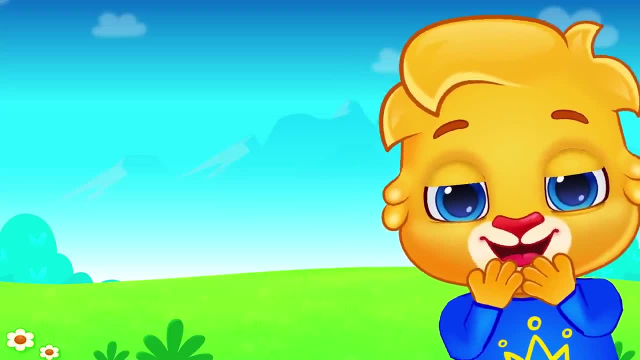 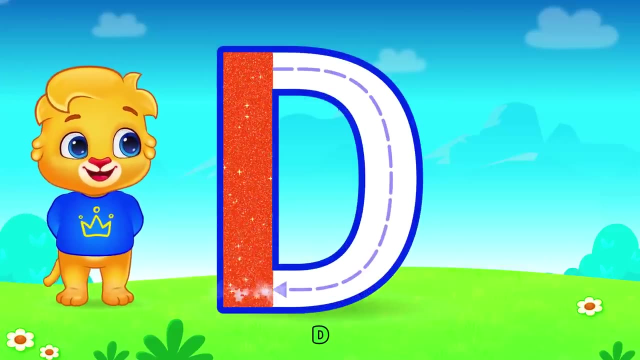 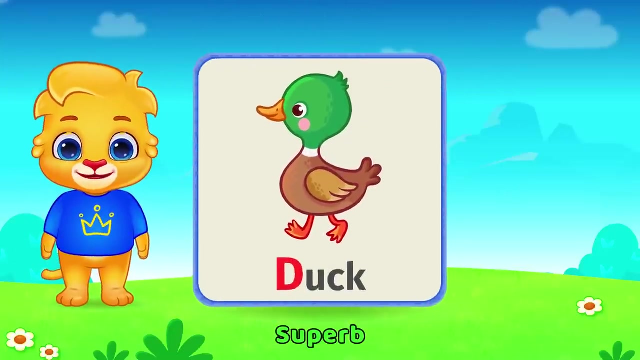 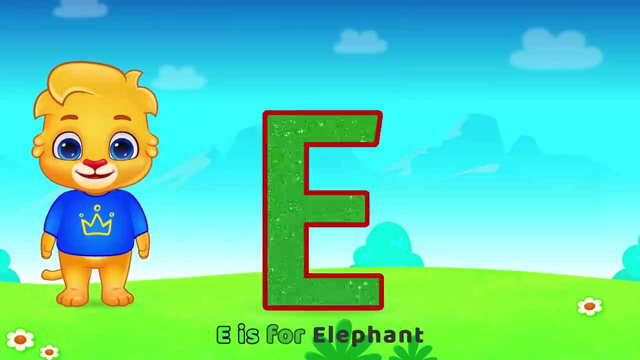 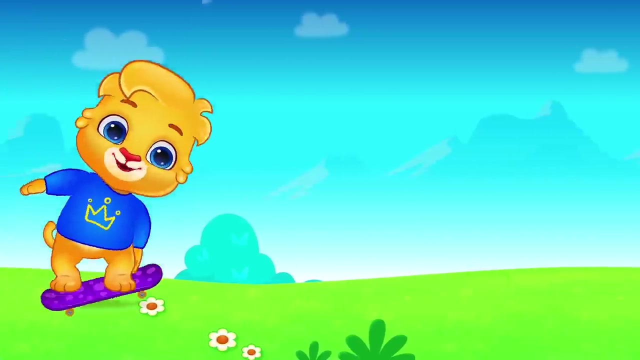 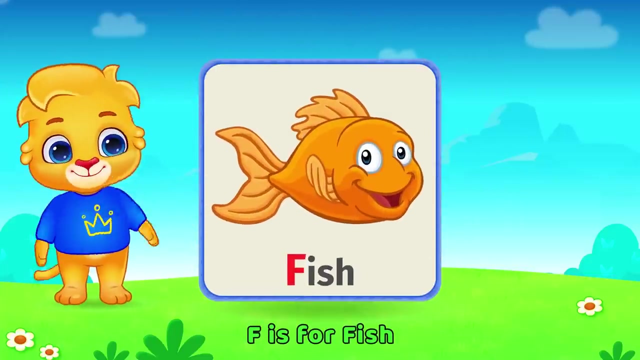 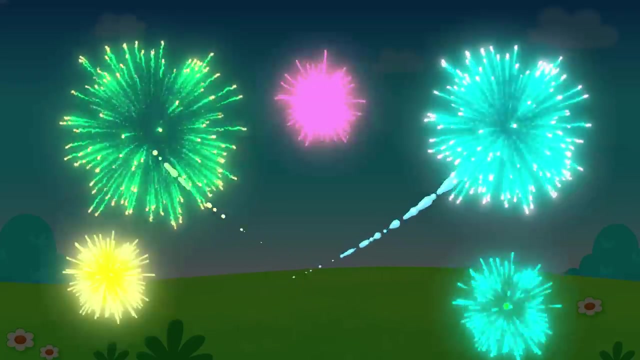 Can you laugh with me? D D D. D is for dog, D is for duck Superb, E. E is for elephant, Hello, F. F is for fish, E is for cat, F is for elephant. 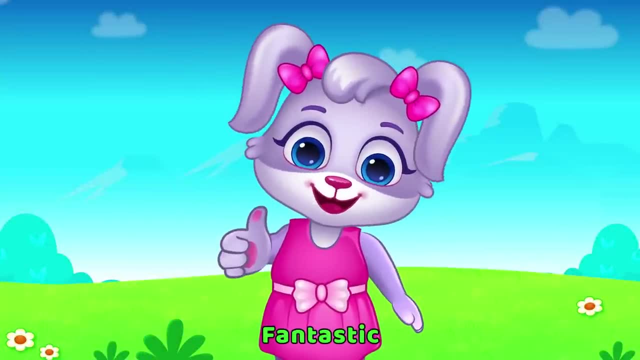 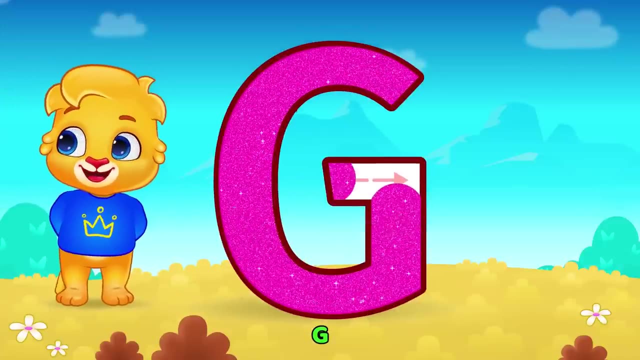 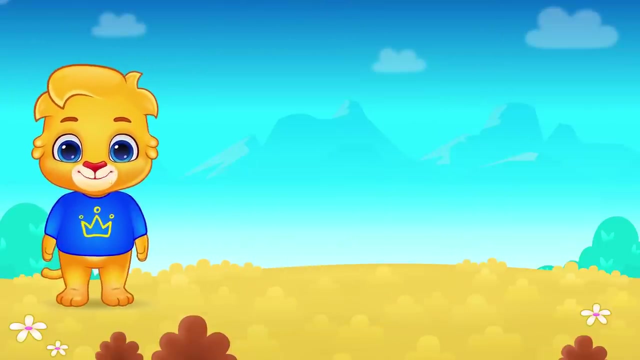 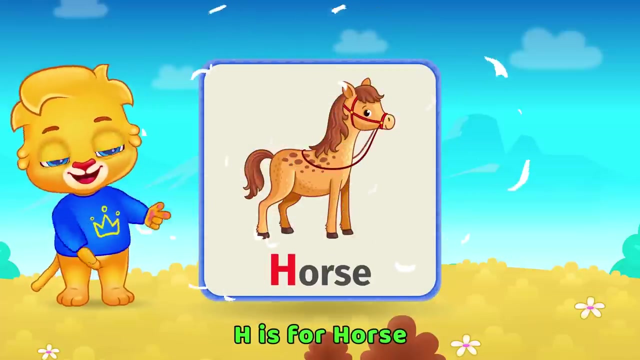 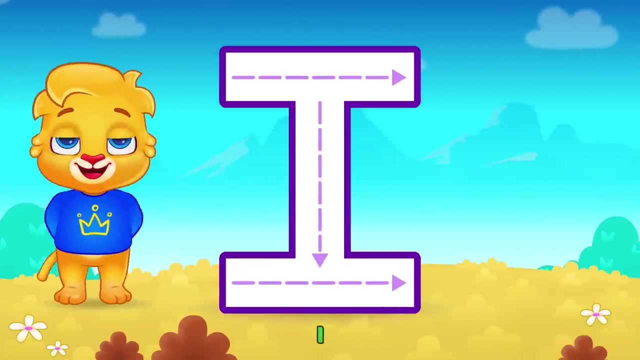 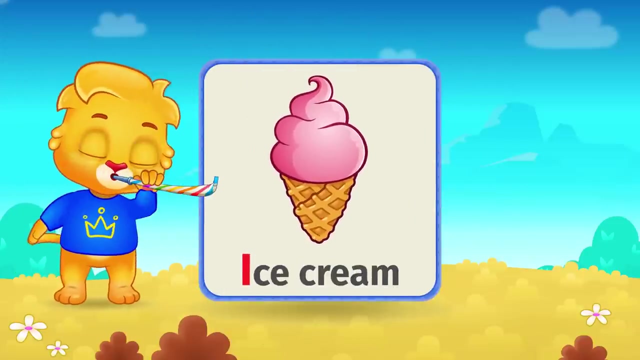 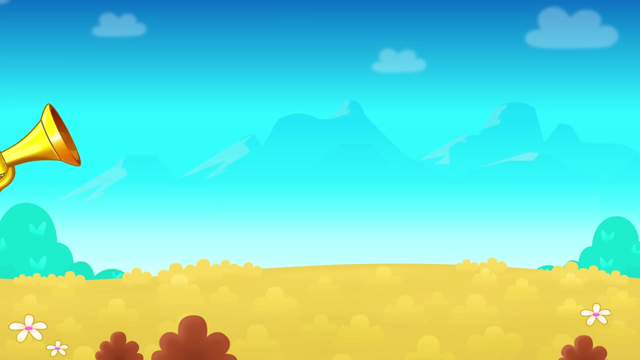 E is for mouse, E, E, E, H, H is for sheep, H is for Thomas, H is for ruffles, H is for hungry H, H is for horse. great job, I. I is for ice cream. hello, my friend. 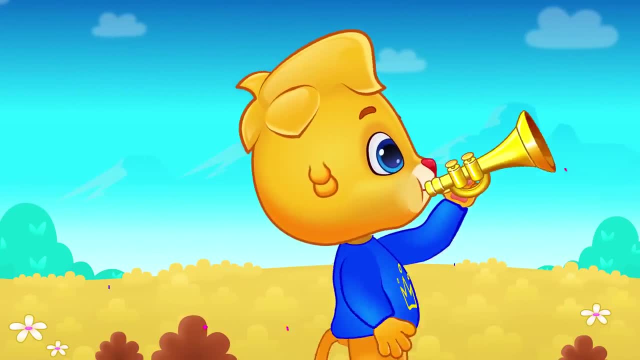 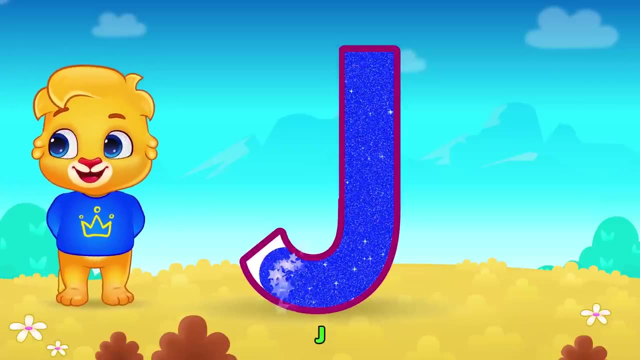 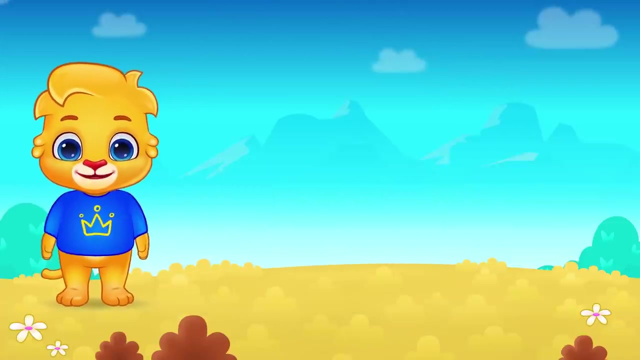 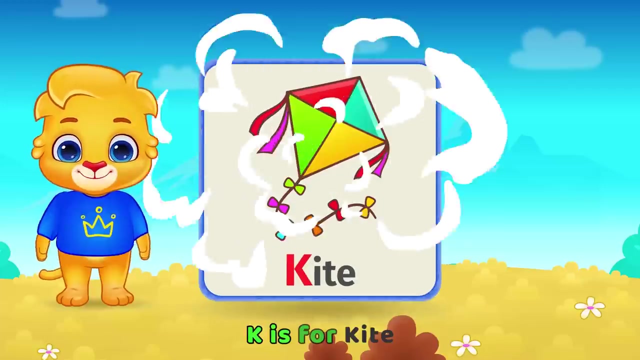 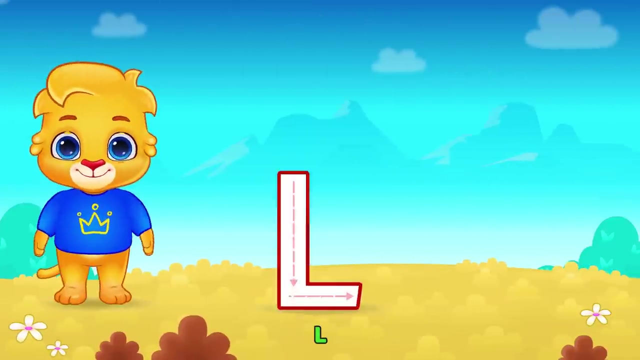 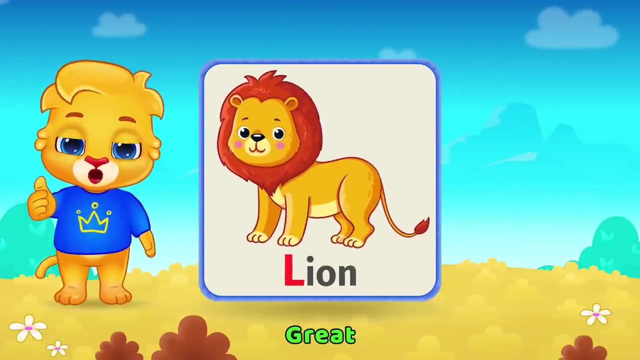 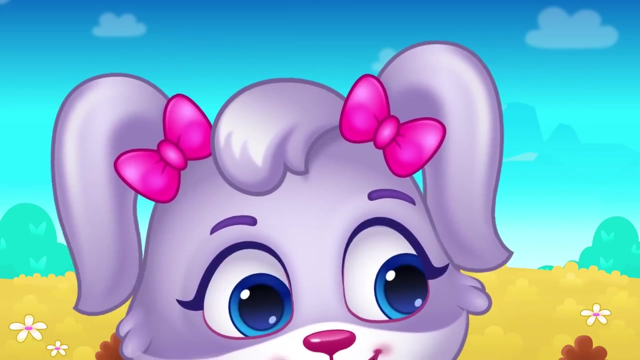 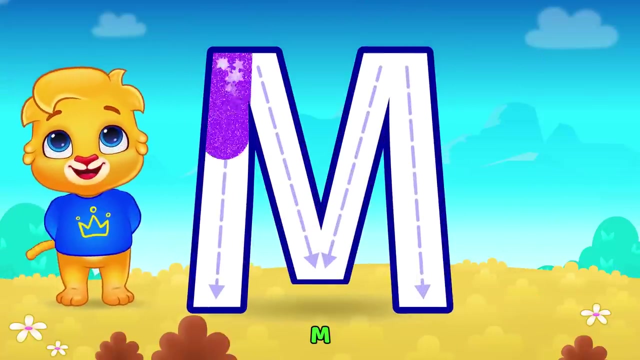 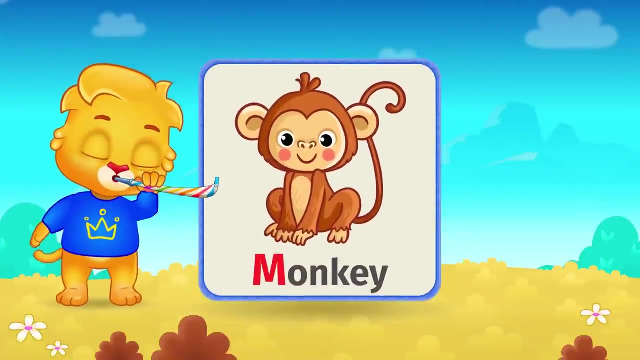 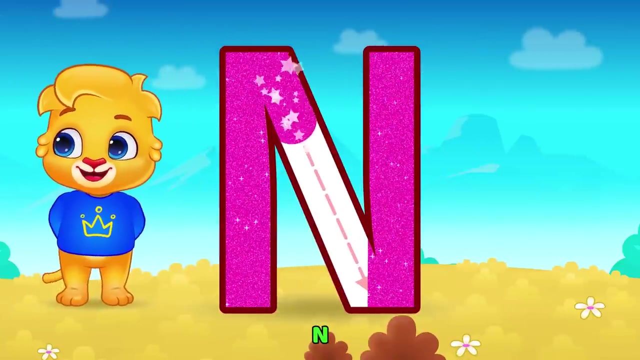 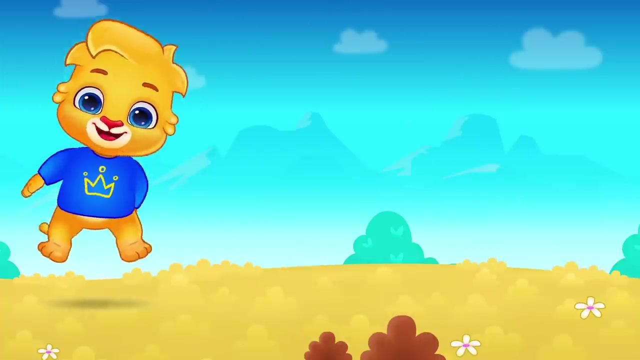 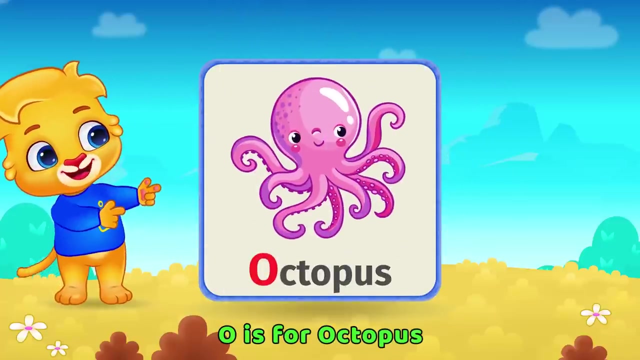 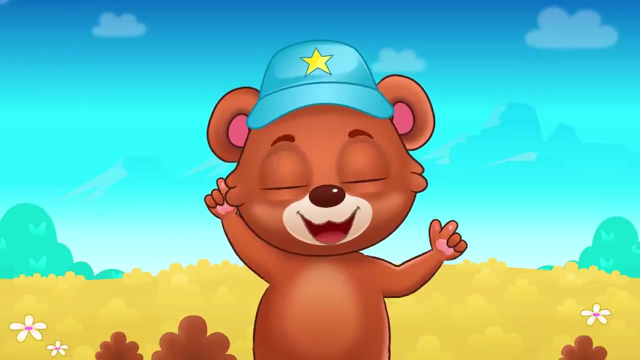 J, J is for juice, K, K is for kite, L, L is for lion, great, M is for monkey, P is for lamb N and P is for necklace. Q O, M is for Ox, O is for ox, N is for bear. well, I, N is for chicken, N is for chicken. 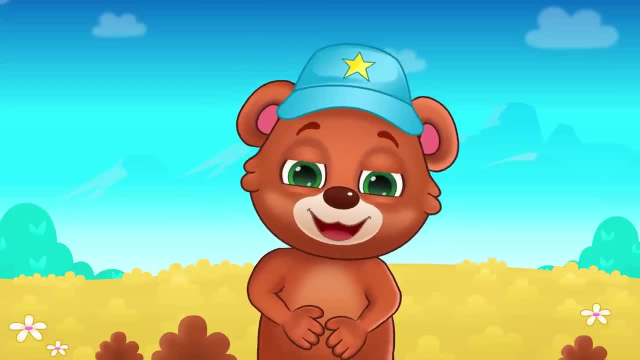 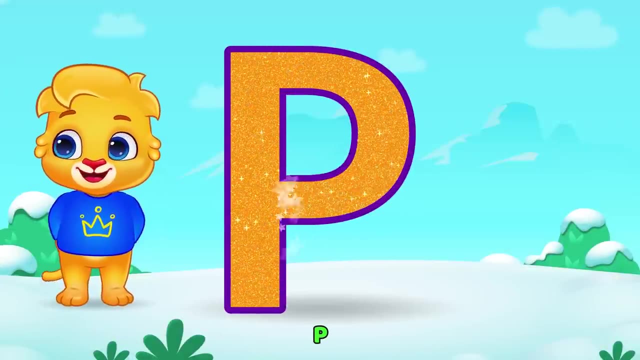 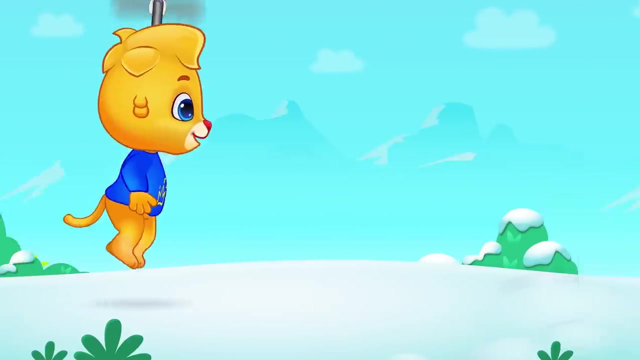 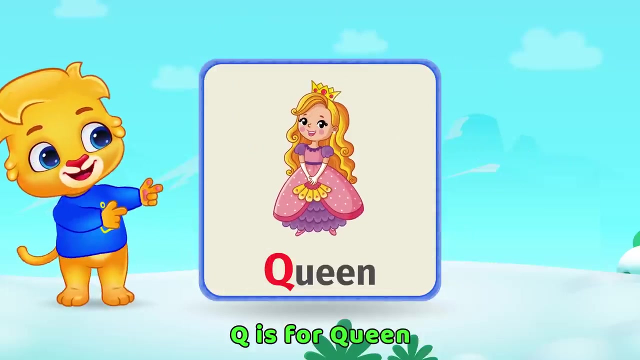 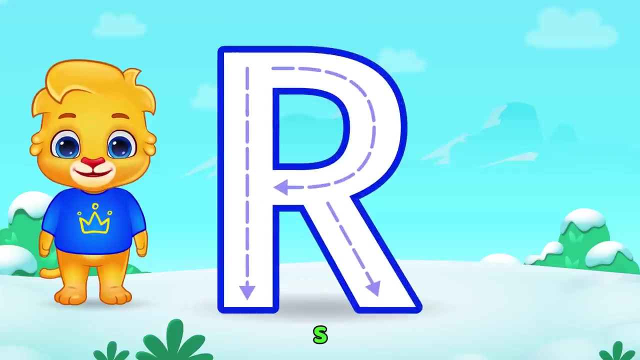 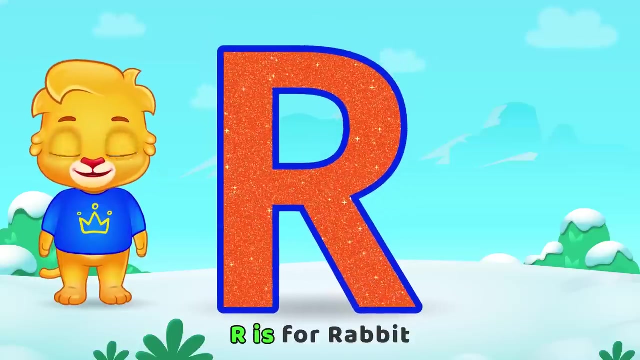 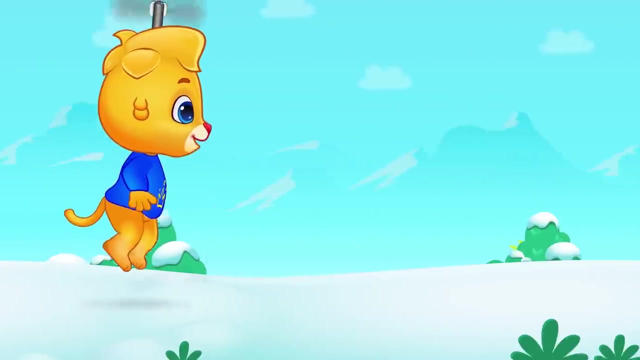 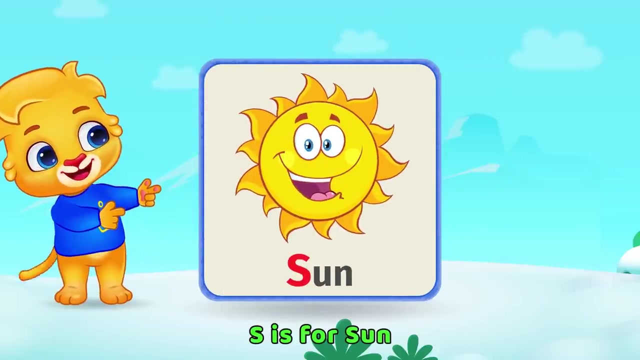 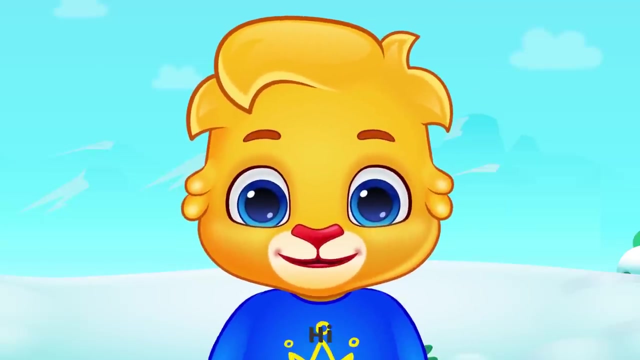 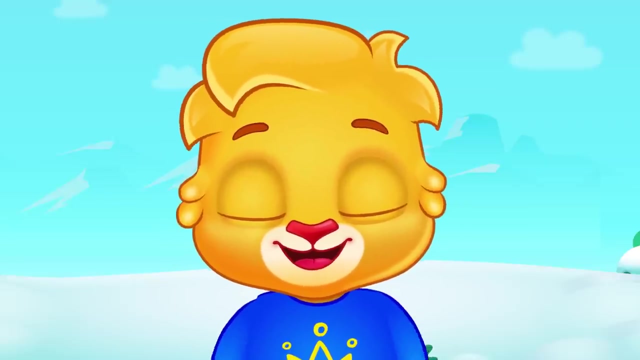 P is for pig, Awesome Q is for queen, Yay S R, Great R is for rabbit S S is for sun. Woohoo, Hi, How are you doing? Wanted to say hi, Bye, for now. T. 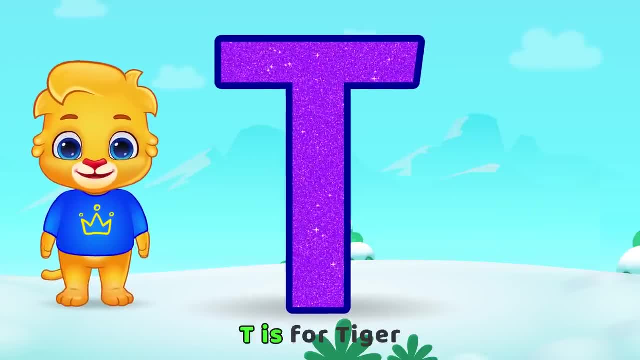 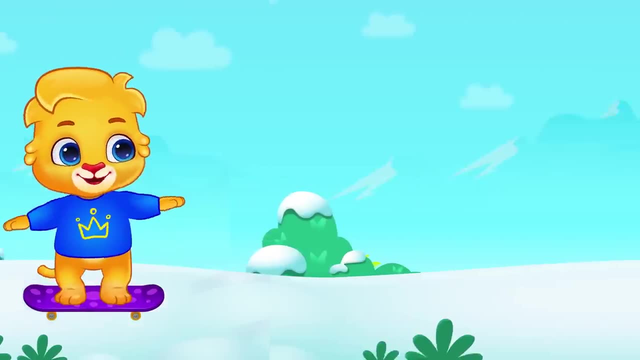 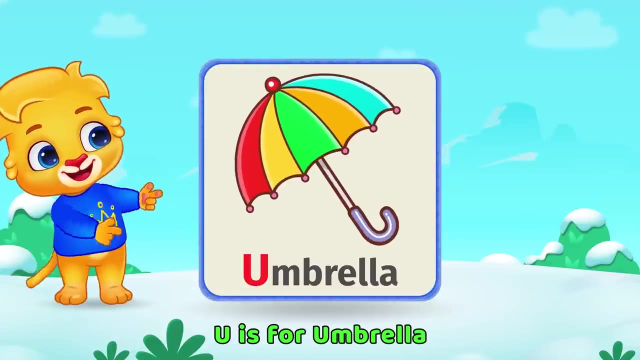 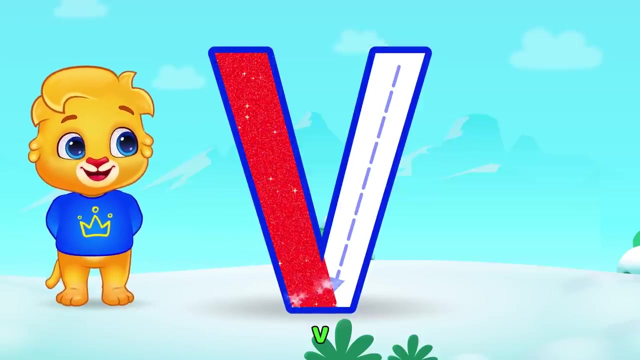 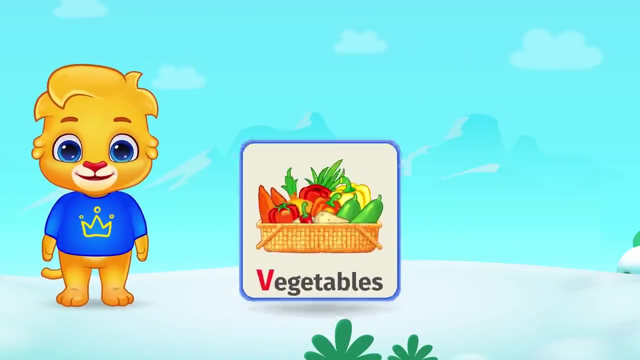 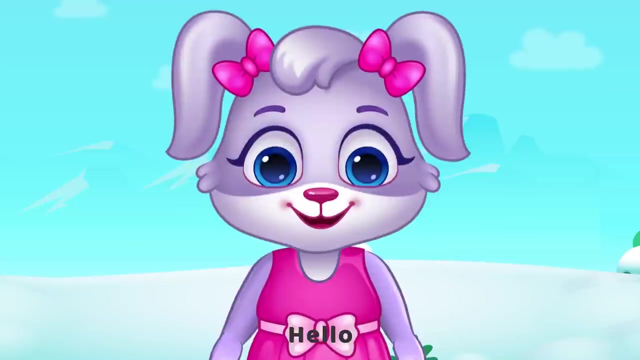 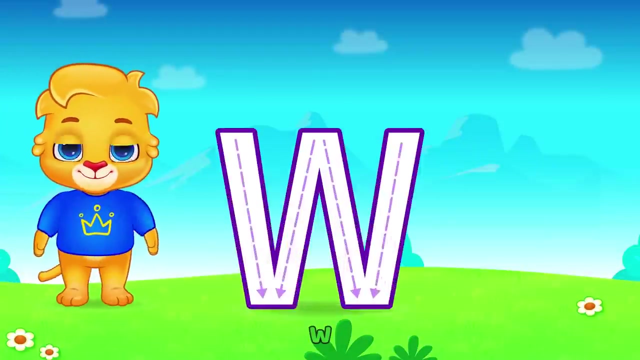 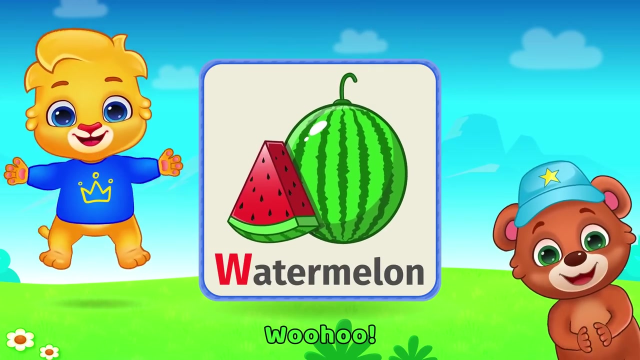 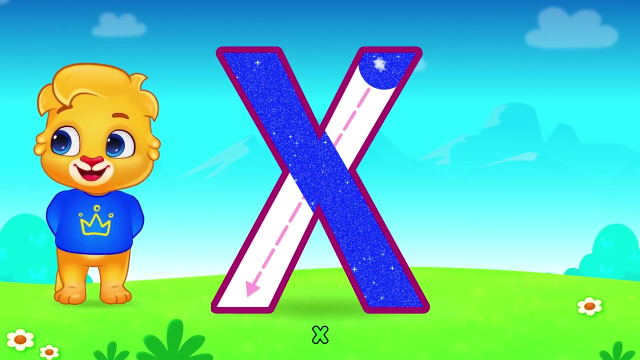 T is for tiger, Well done, U. U is for umbrella, V, V is for vegetables. Hello, Hello, Hello, Hello, Hello, Bye-bye, Bye-bye. W. W is for watermelon, Woohoo, X. X is for xylophone. 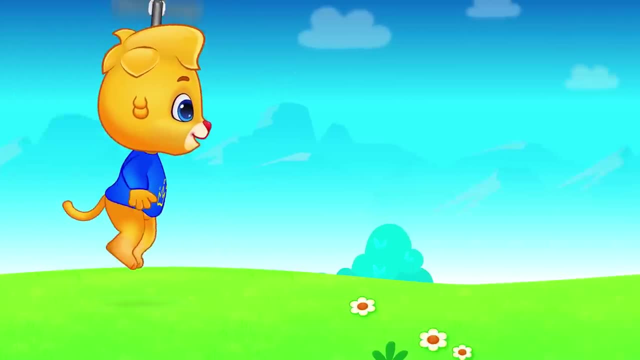 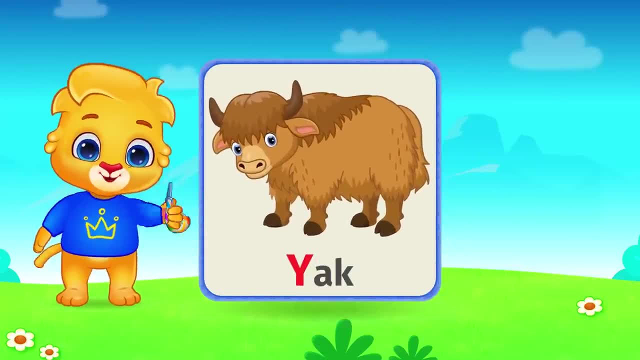 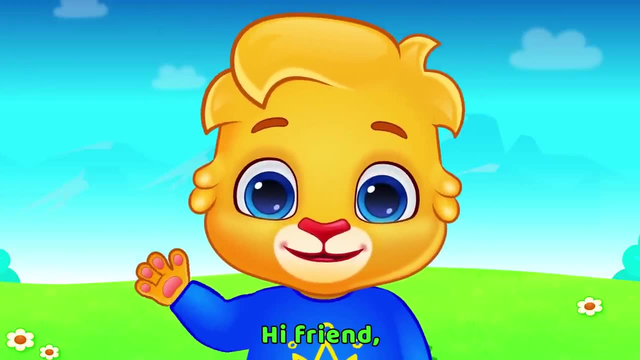 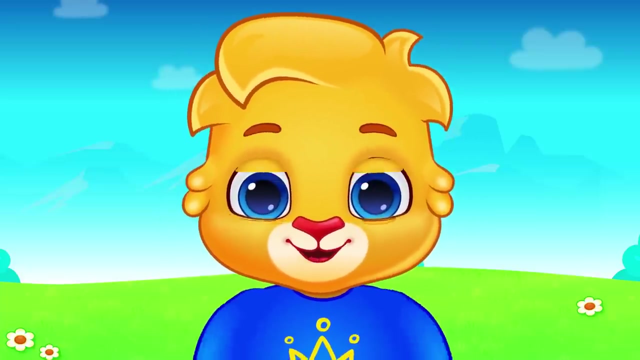 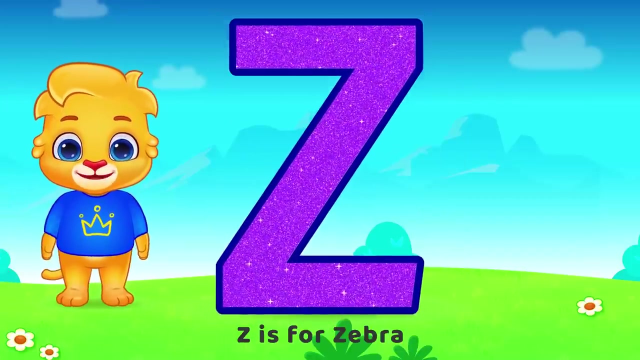 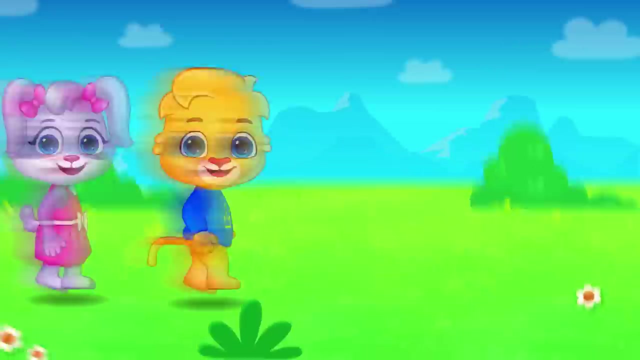 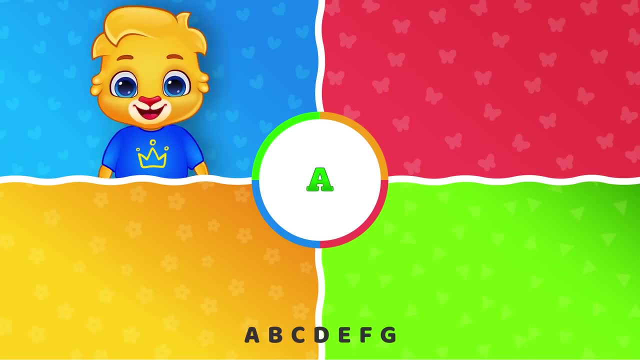 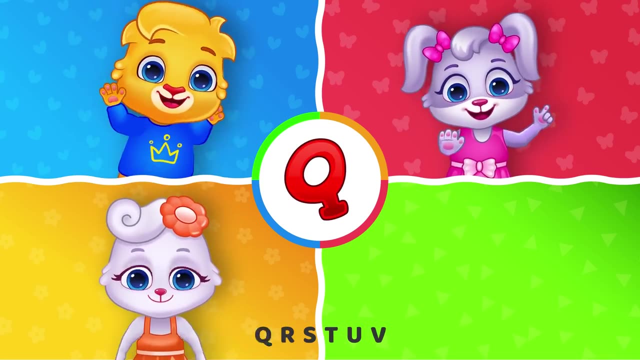 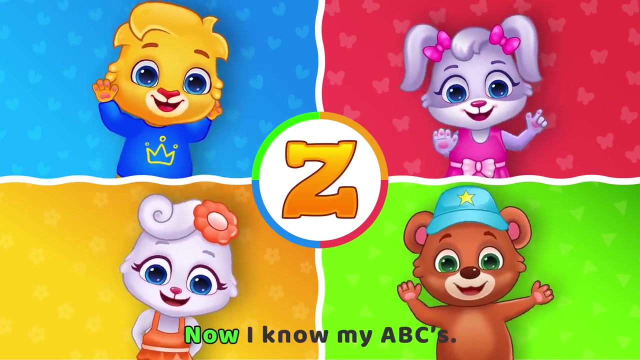 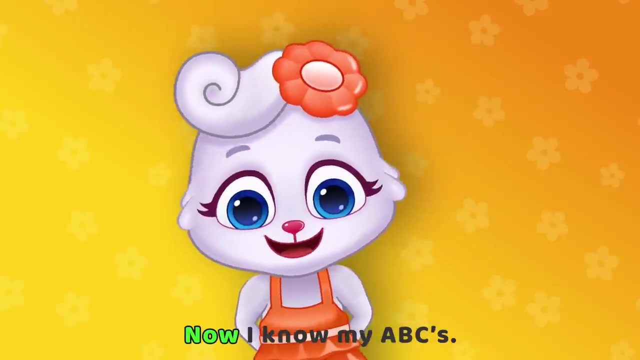 Z, Z, Z Z Z Z. A, B, C, D, E, F, G, H, I, J, K, Z, Q, R, X, T, U, V, W, X, Y & Z. Now I know my ABCs. Next time won't you sing with me? Now, I know my ABCs. Next time won't you sing with me? 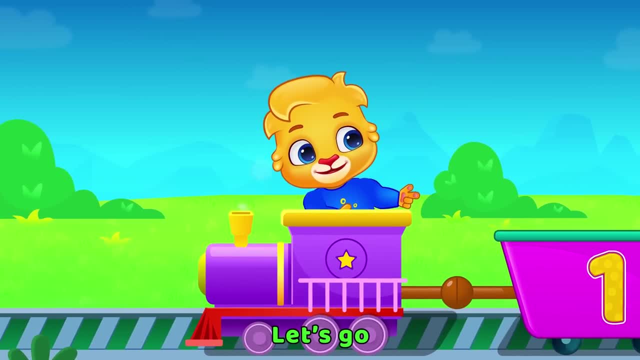 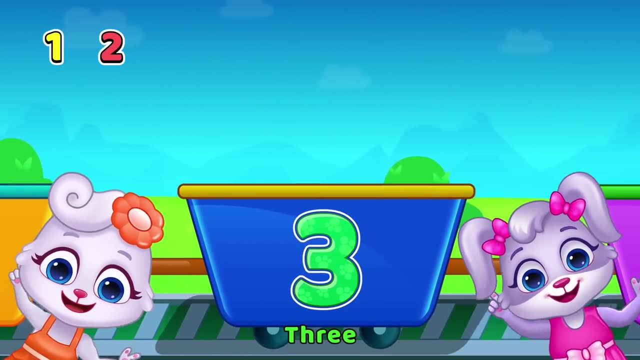 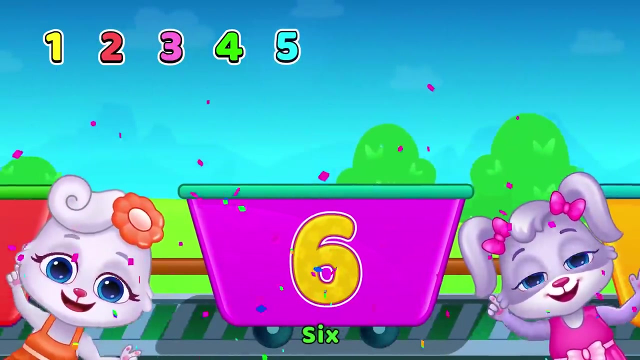 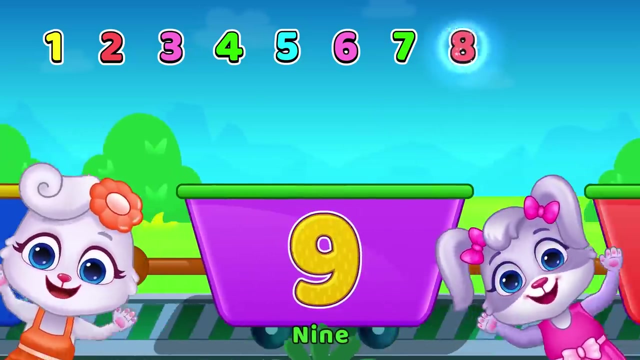 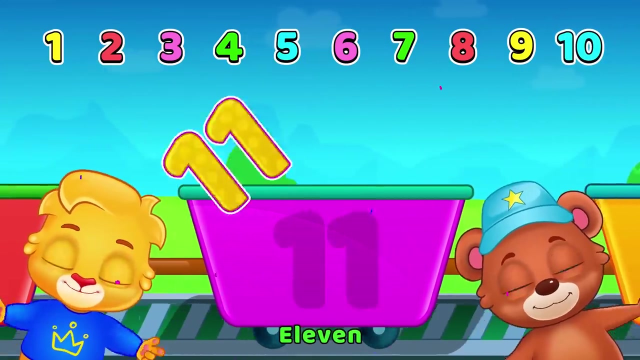 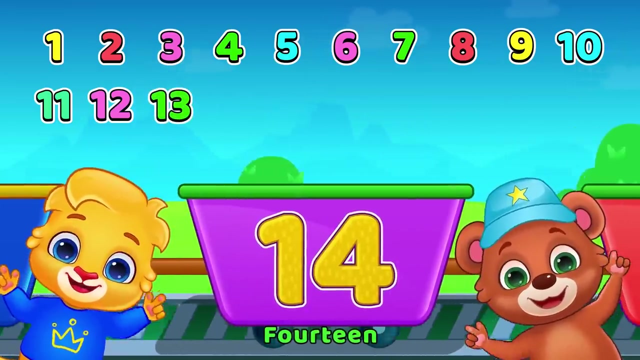 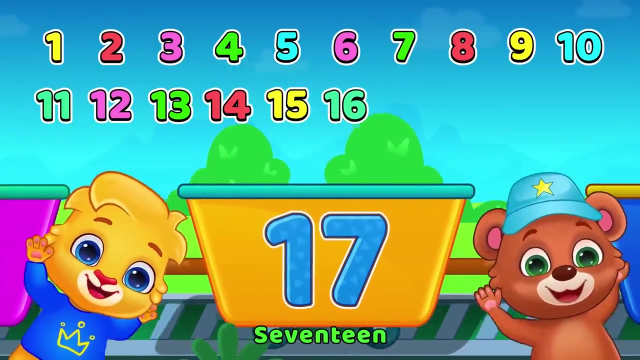 2020. Let's go: 1, 2, 3, 4, 5, 6, 7, 8, 9, 10, 11, 12, 13, 12, 13, 14, 15, 16, 17, 18, 19, 20, 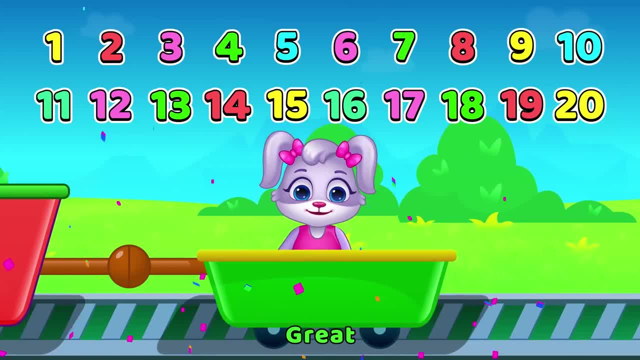 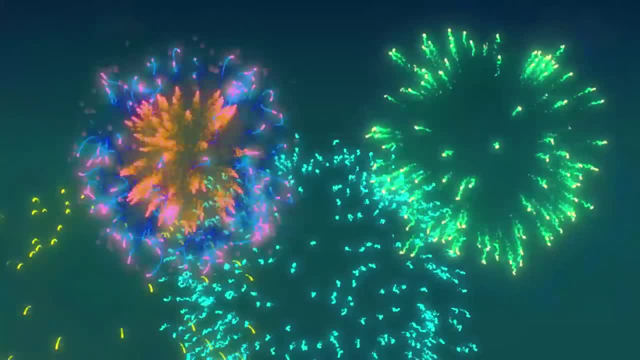 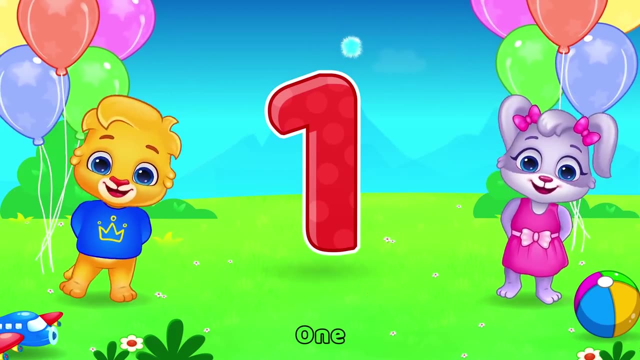 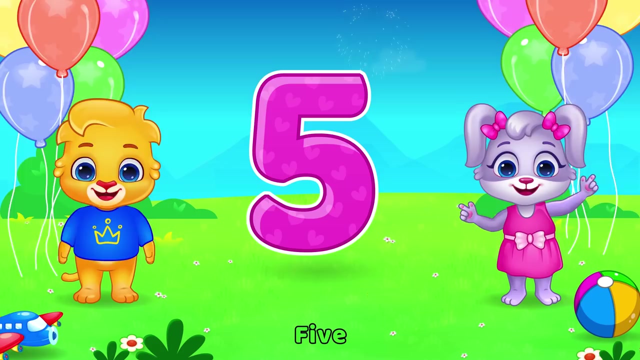 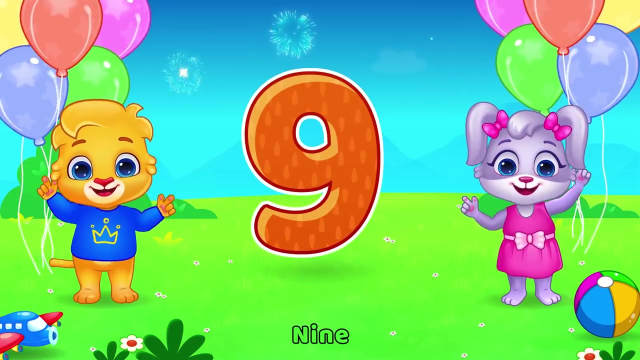 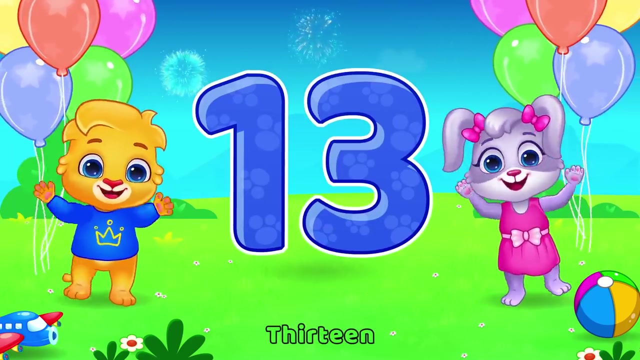 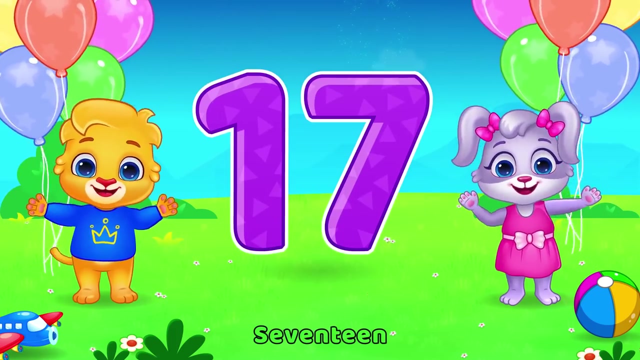 Great, Hey, now let's do it a little faster. 1, 2, 3, 4, 5, 6, 7, 8, 9, 10, 11, 12, 13, 14, 15, 16, 17, 18, 19. 20, 21, 22, 23, 24, 25, 26, 27, 28, 29, 30, 31, 32, 33, 34, 35, 36, 37, 38, 39, 40, 41, 42, 43, 44, 45. 46, 47, 48, 49, 50, 51, 52, 53, 54, 55, 56, 57, 58, 59, 60, 61, 62, 63, 64, 65, 67, 68, 69, 69, 70, 71. 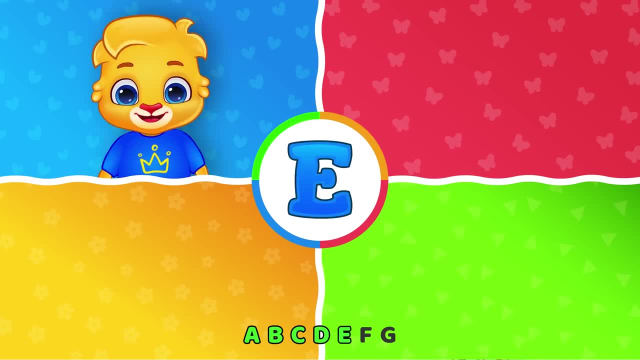 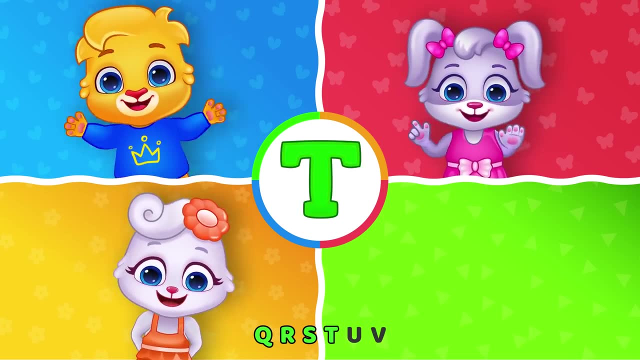 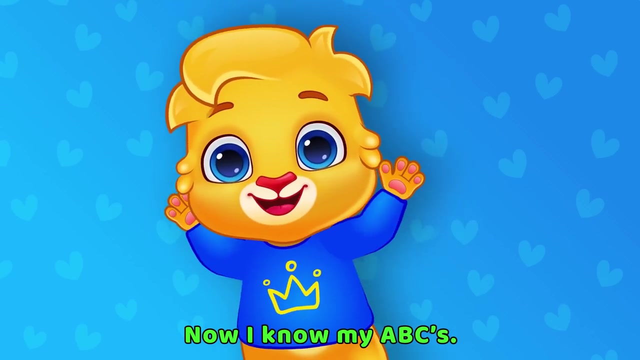 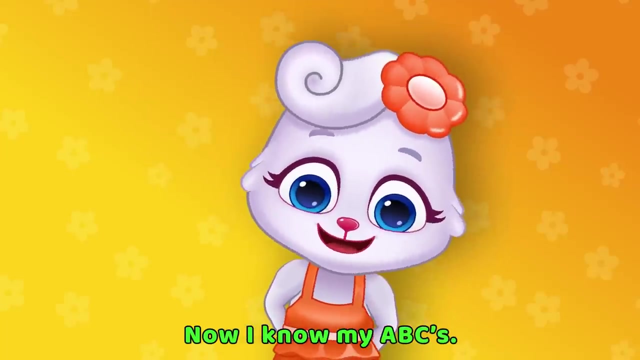 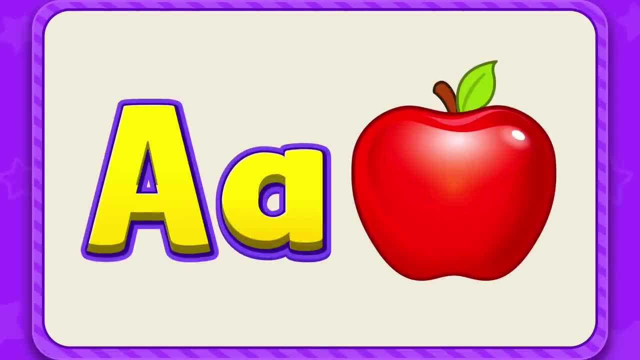 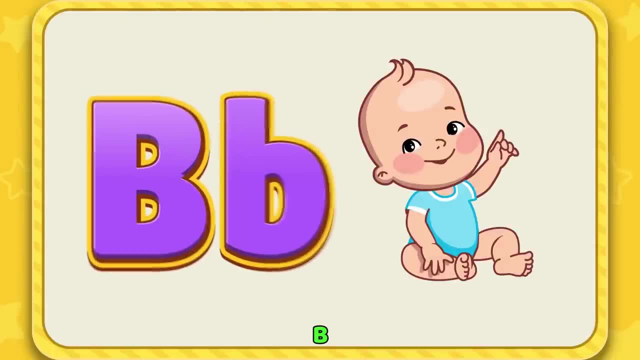 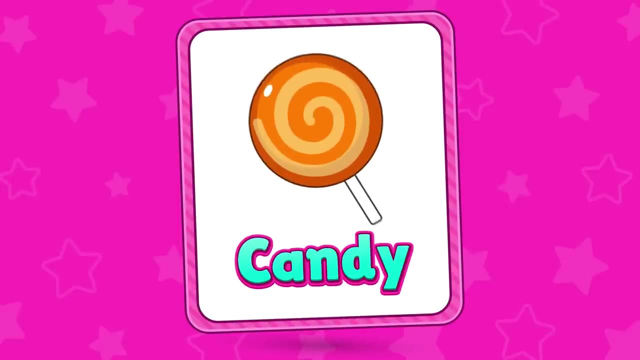 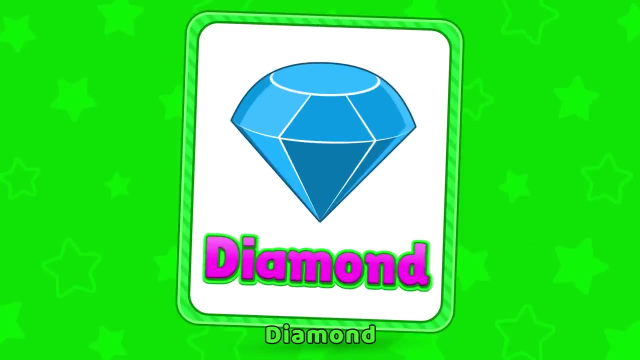 53, 54, 55, 55, 66, 66, 66, 76, 77, 77, 78, 98, 99, 100, 100, 100. Candy c-c-candy. c-candy D is for diamond d-d-diamond d-d-diamond d-diamond. 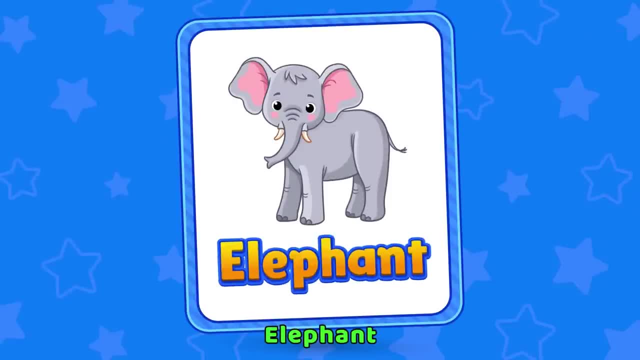 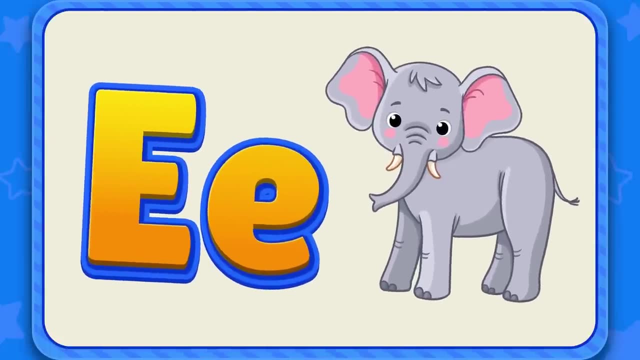 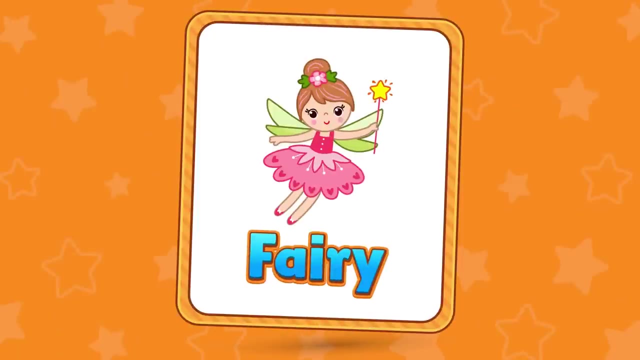 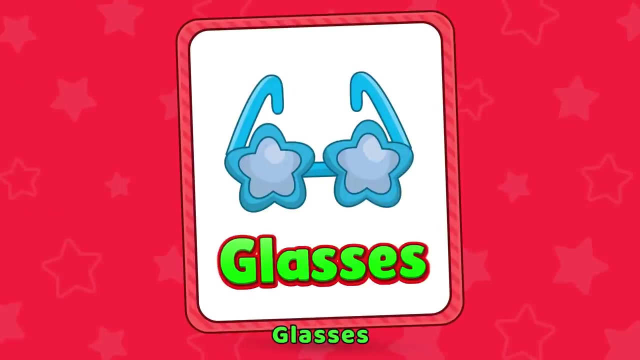 E is for elephant: e-e-elephant, e-e-elephant e-elephant. F is for fairy, f-f-fairy, f-f-fairy, f-fairy. G is for glasses: g-g-glasses, g-g-glasses, g-glasses. 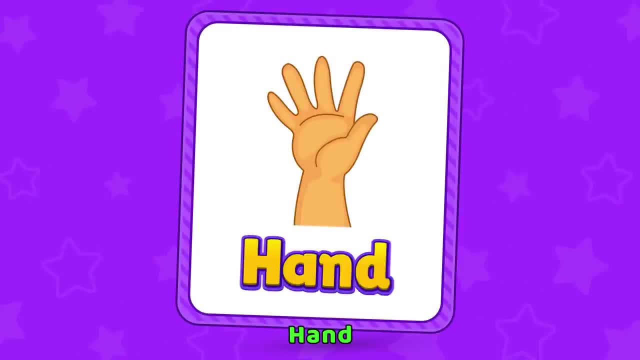 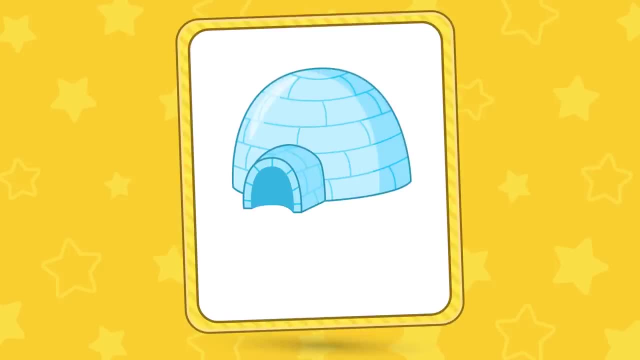 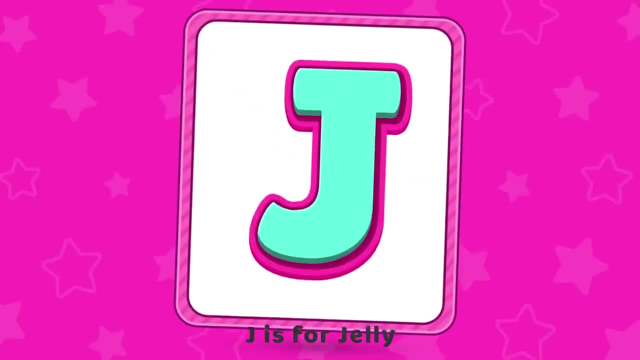 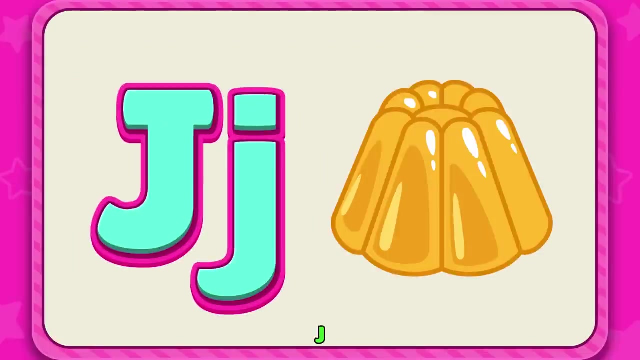 H is for hand h-h-hand, h-h-hand, h-h-hand. I is for igloo i-i-igloo, i-i-igloo, i-igloo. J is for jelly, j-j-jelly, j-j-jelly, j-j-jelly. 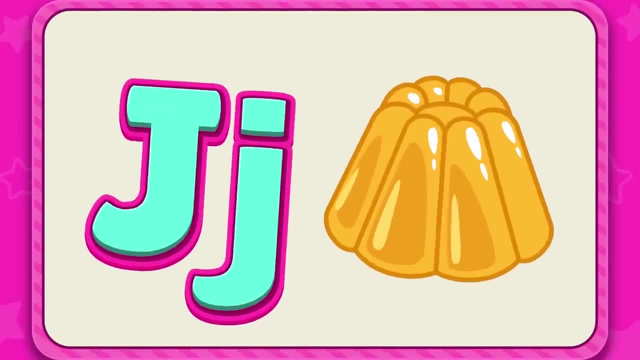 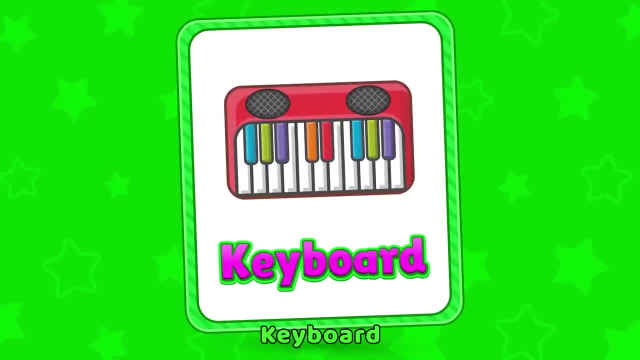 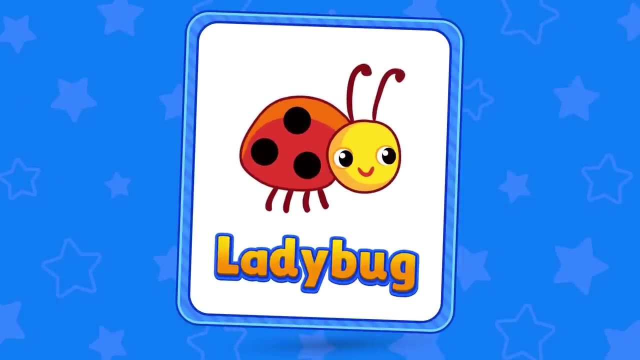 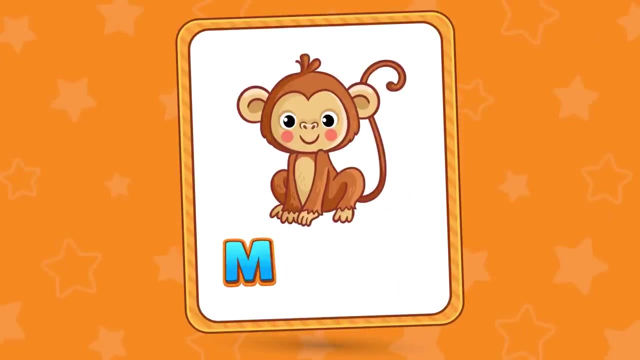 K is for keyboard k-k-keyboard, k-k-keyboard K keyboard. L is for ladybug u-u-ladybug, u-u-ladybug l-ladybug. M is for monkey u-u-monkey, u-u-monkey, m-m-monkey. 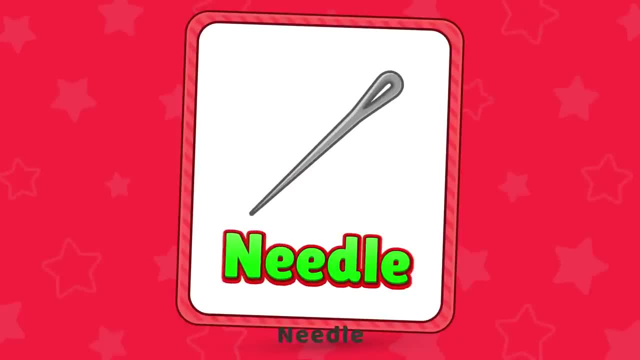 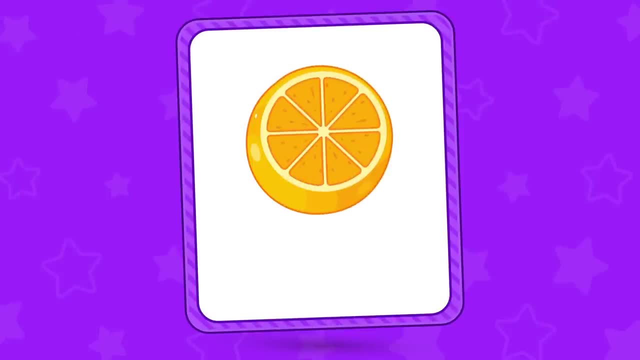 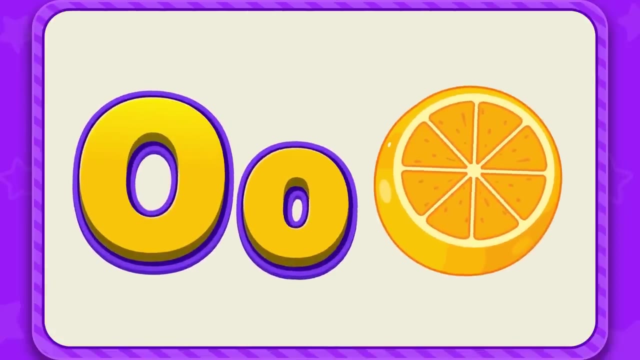 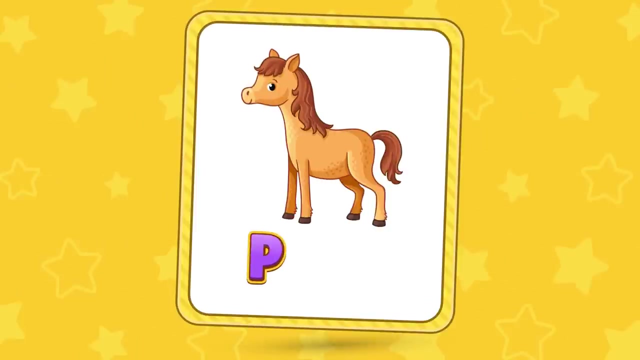 N is for needle u-u-needle, u-u-needle n-needle. O is for orange o-o-orange O-o-orange o-orange. P is for pony, p-p-pony, p-p-pony, p-pony. 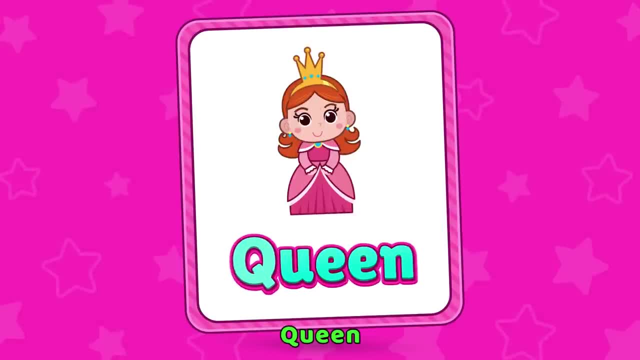 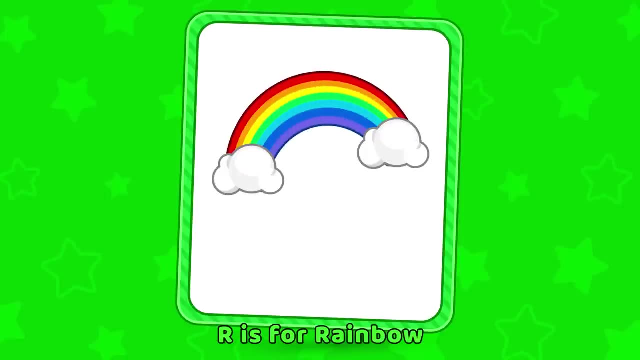 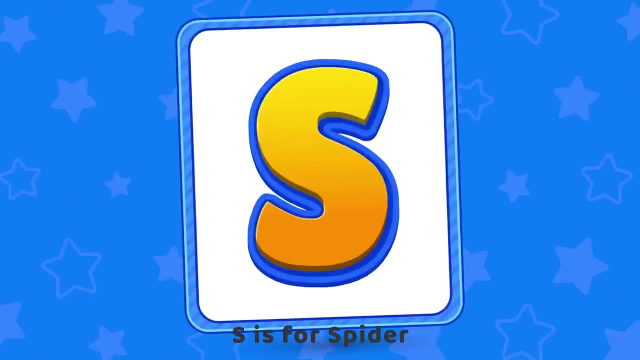 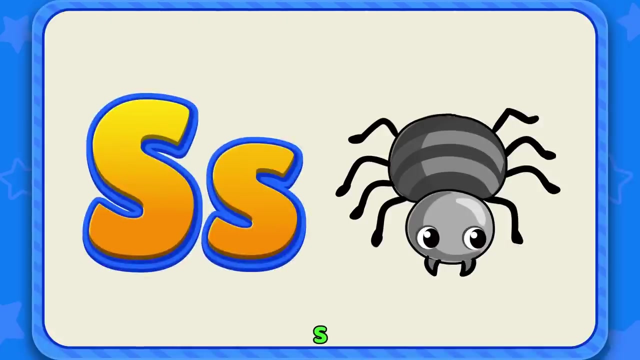 Q is for queen q-q-queen, q-q-queen q-q-queen, R is for rainbow r-r-rainbow R-r-rainbow r-rainbow, S is for spider s-s-spider, s-s-spider s-spider. 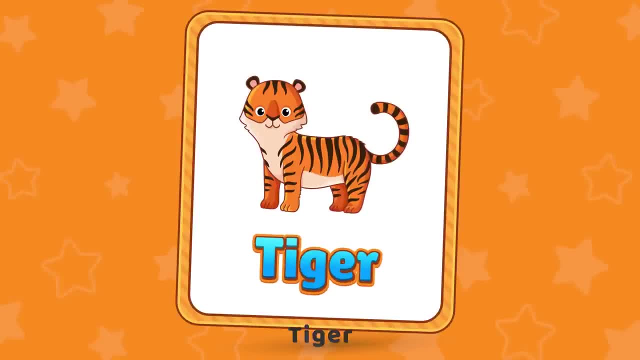 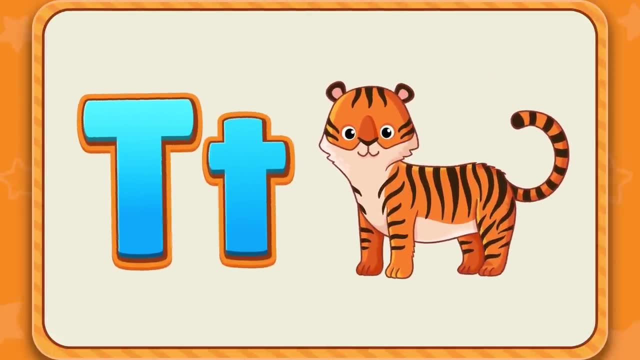 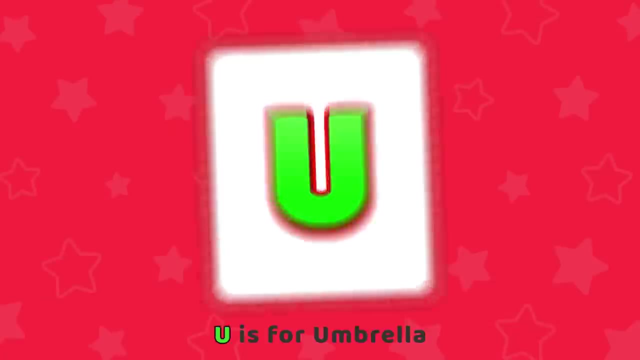 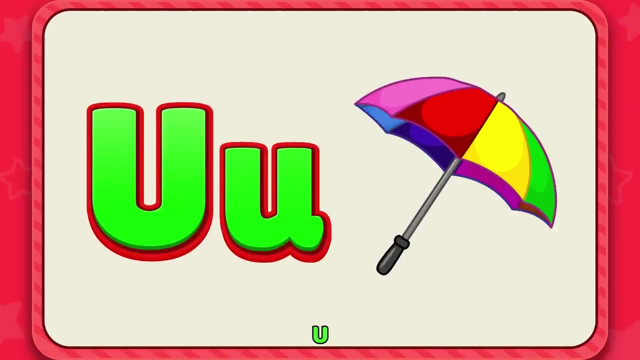 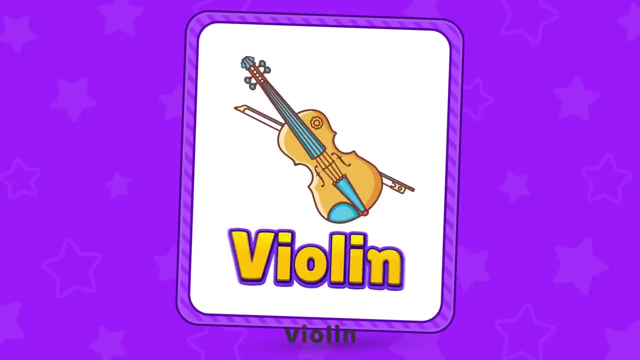 T is for tiger t-t-tiger, t-t-tiger, t-t-tiger. U is for umbrella a-a-umbrella a-a-umbrella u-umbrella V is for violin v-v-violin v-v-violin v-v-violin. 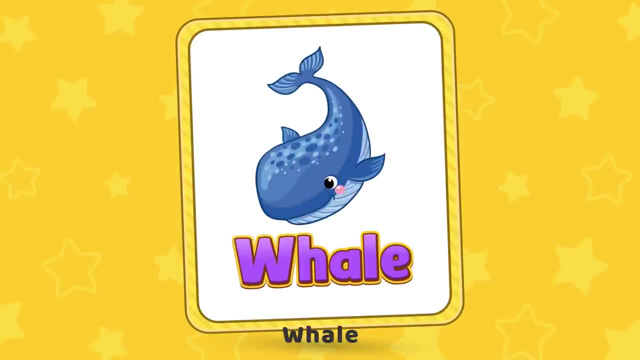 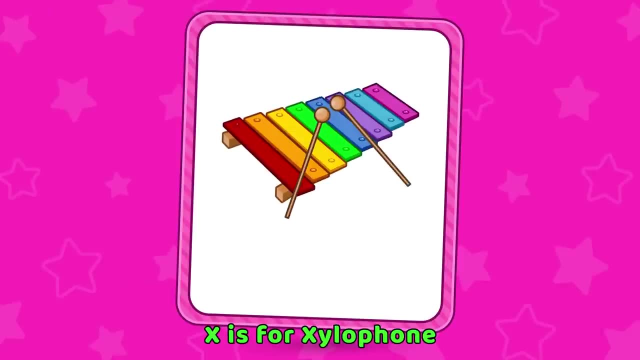 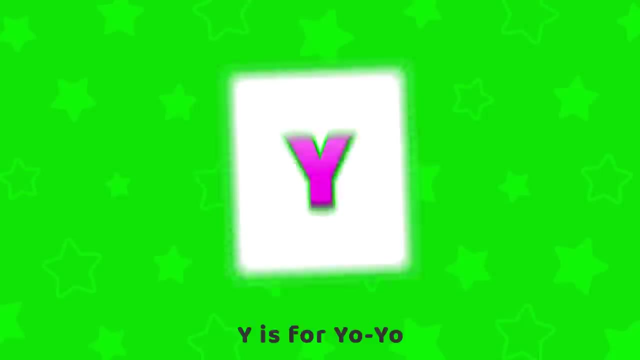 W is for whale, w-w-whale, w-w-whale, w-w-whale, X is for xylophone z-z-zone, Z z xylophone Z z xylophone X. xylophone Y is for yo-yo. 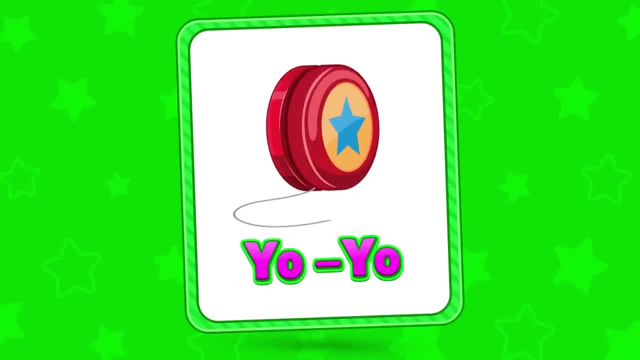 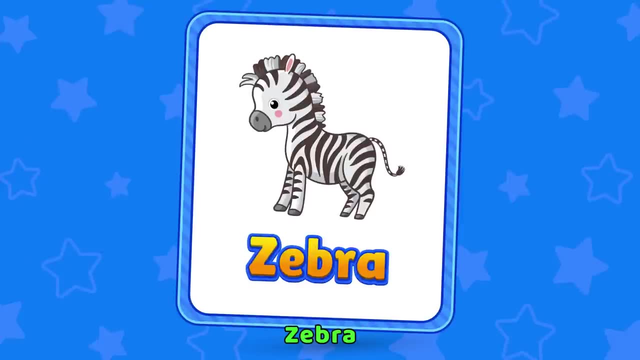 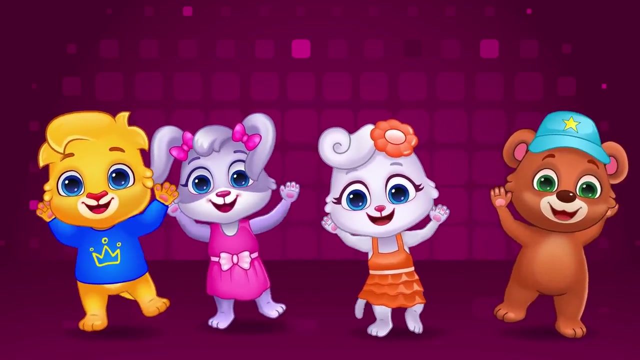 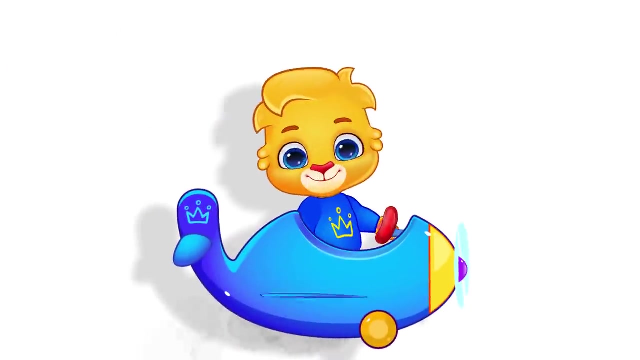 Y y, yo-yo, Y y, yo-yo, Y, yo-yo. Z is for zebra Z z zebra Z z zebra Z zebra Z zebra. Can I get a big smile from you? 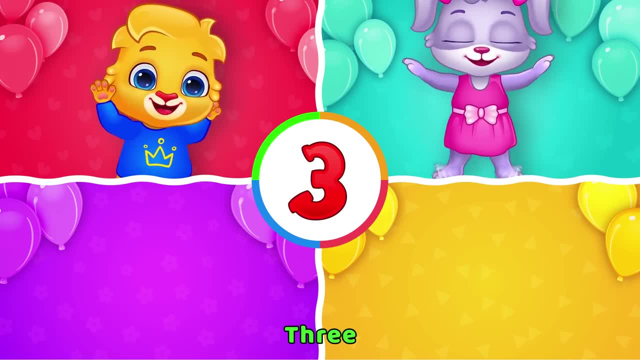 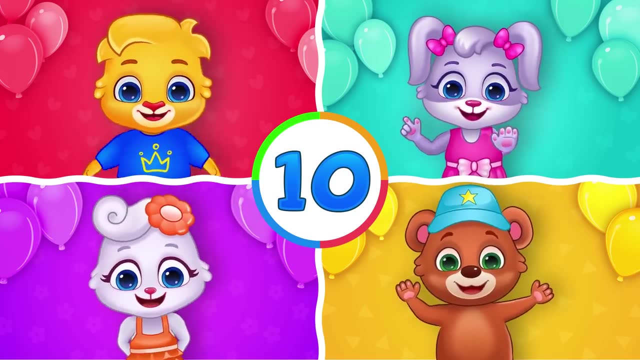 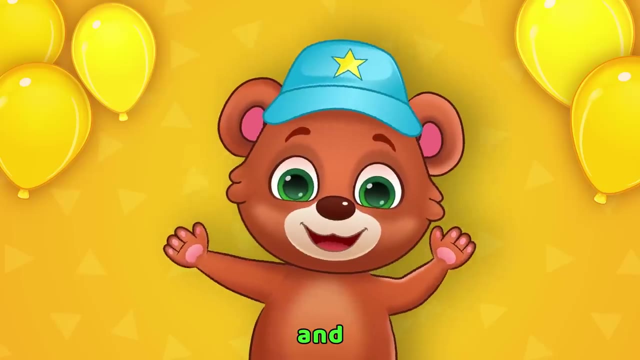 Woohoo. One, two, three, Four, five, six, Seven, eight, nine, Ten. One, two, three, Four, five, six, Seven, eight, nine And ten. You and I my friend, You and I my friend, You and I my friend. 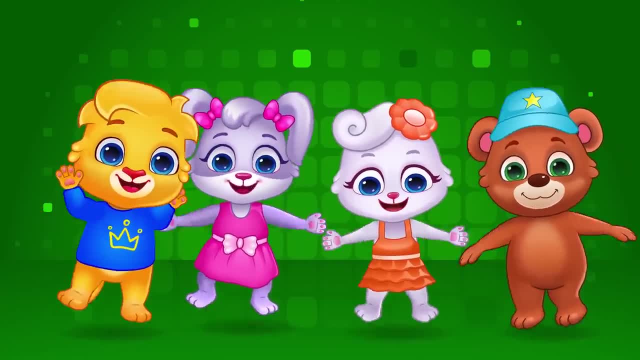 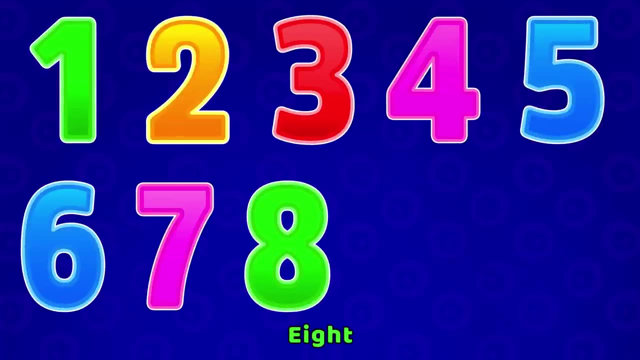 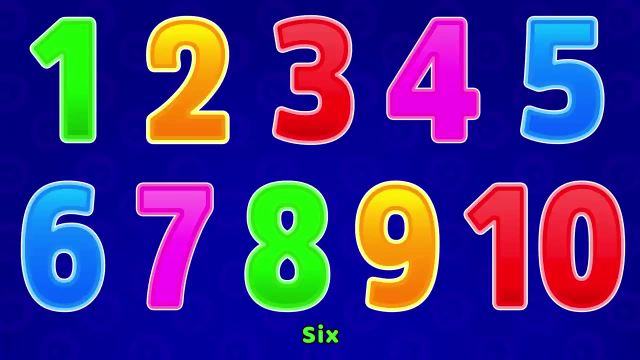 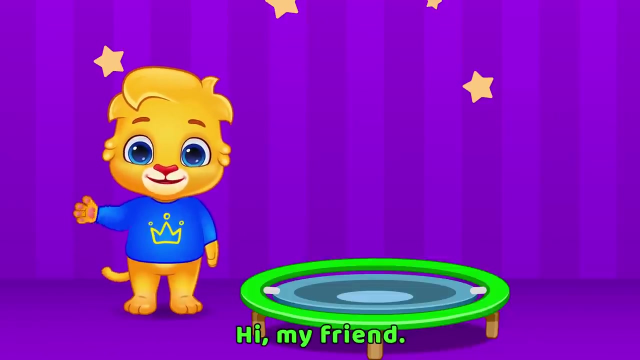 We can count to ten. We can count to ten, Woohoo. One, two, three, Four, five, six, Seven, eight, nine, Ten. One, two, three, Four, five, six, Seven, eight, nine, Ten. Hi, my friend, Today we're going to learn numbers and counting. 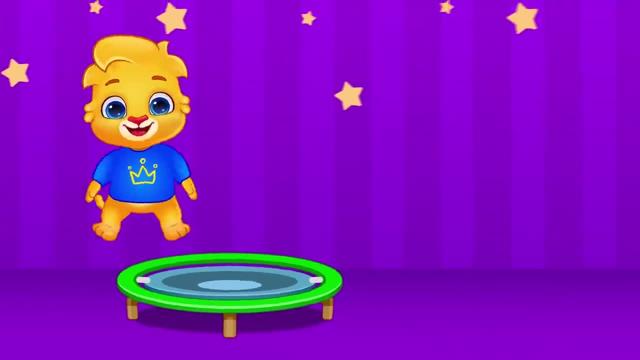 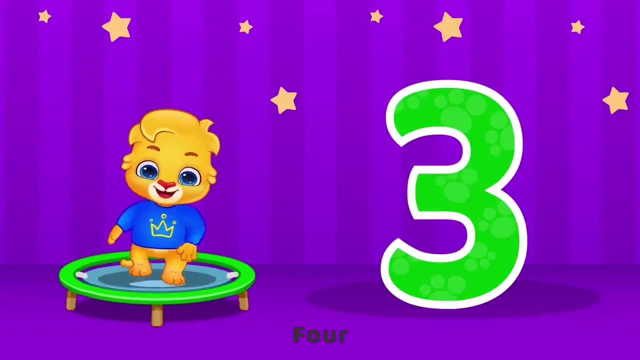 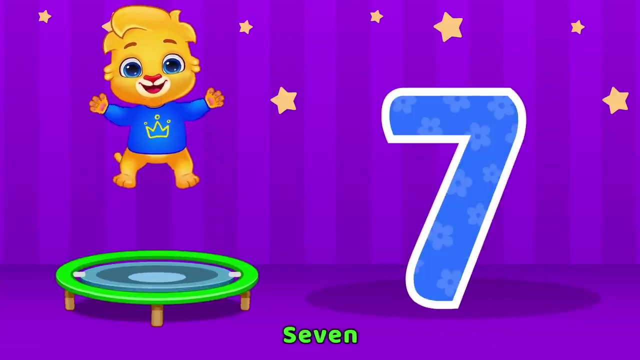 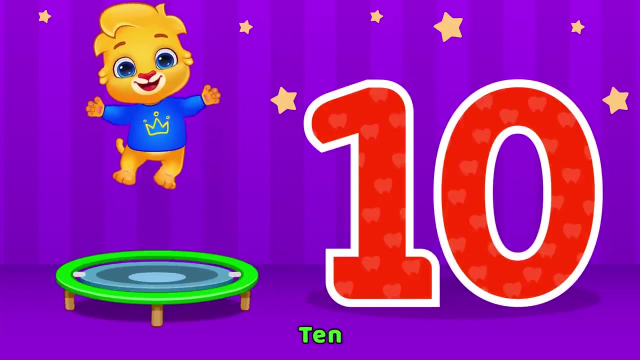 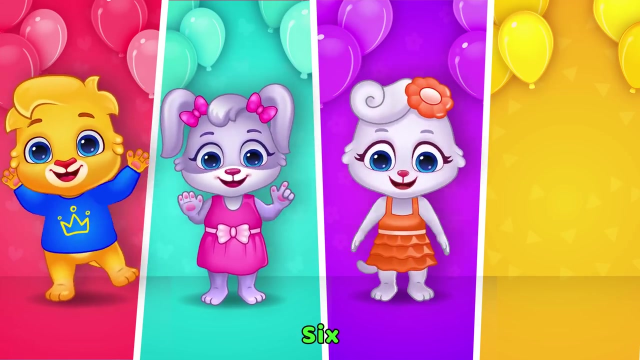 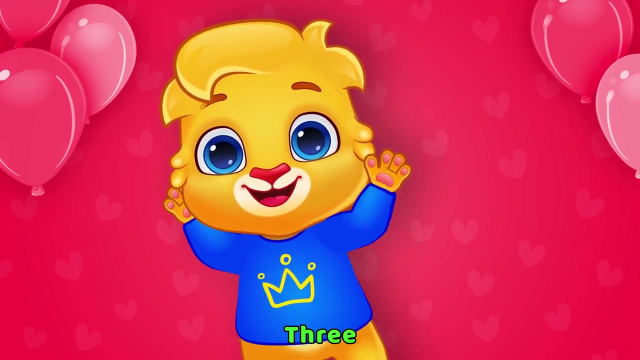 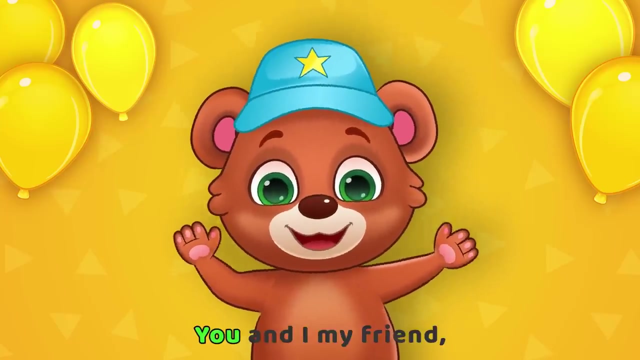 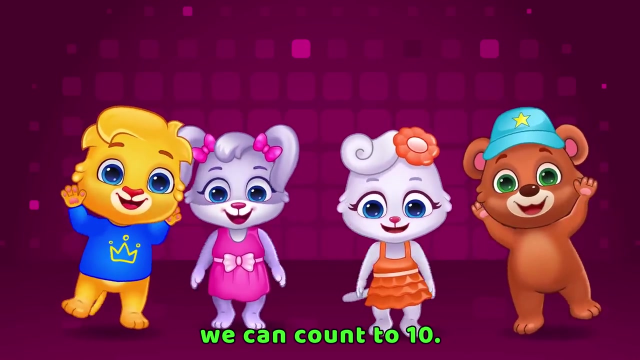 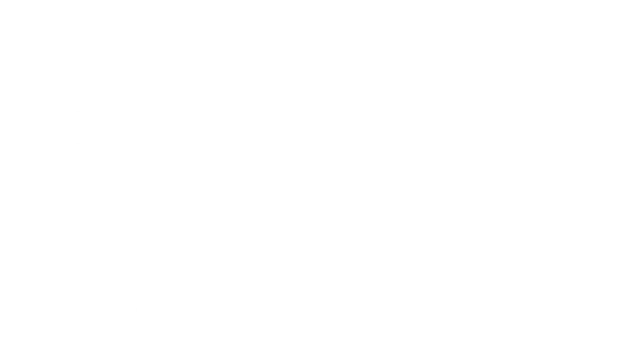 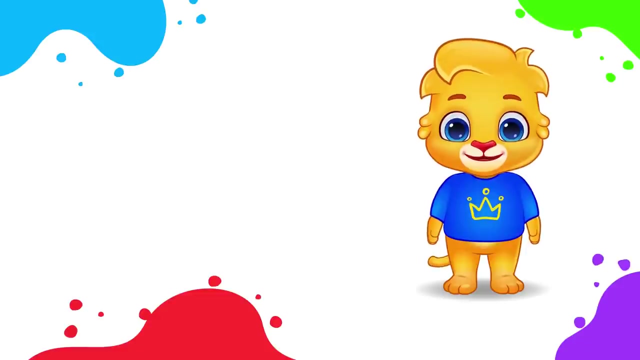 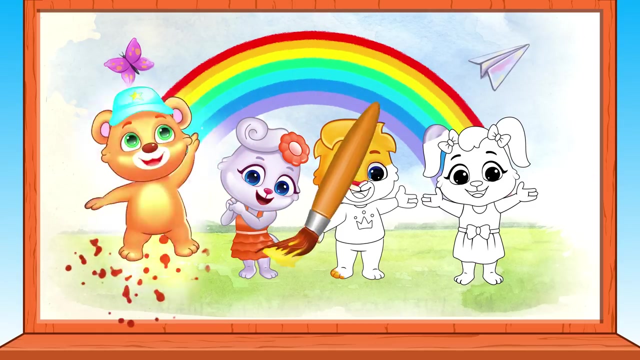 Today we're going to learn numbers and counting. One, Two, Three, Four, Five, Six, Seven, Eight, Nine, Ten. One, Two, Three, Four, Five, Six, Seven, Eight Nine Ten. One, Two, Three, Four, Five, Six, Four, Three, Two. One, Two, One, Two, Three Two. One, Two, Two, Three, Two, Three, Two. 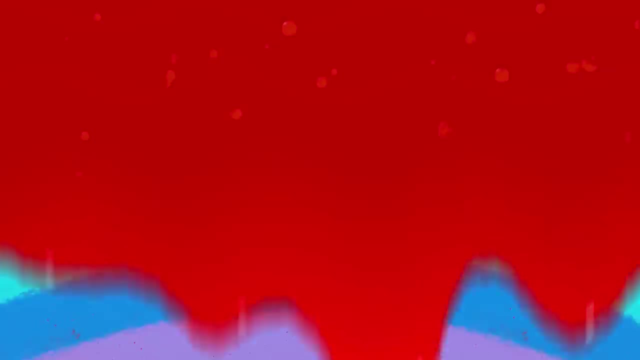 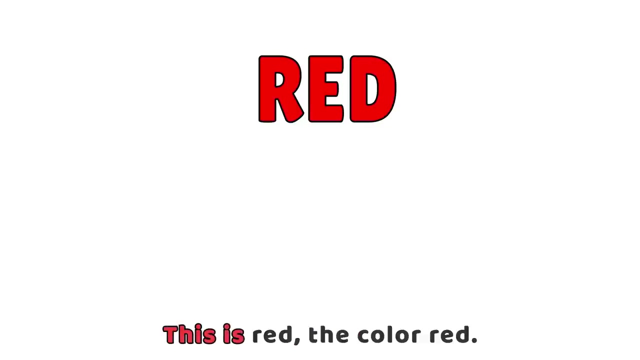 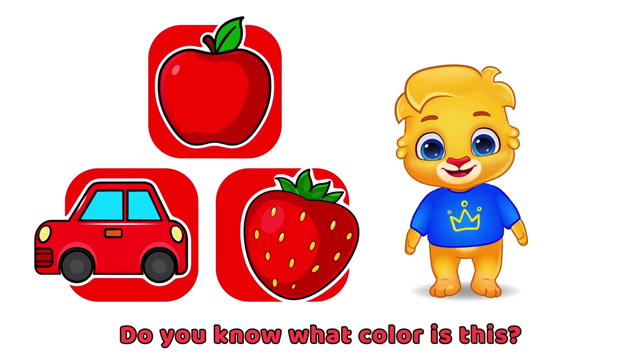 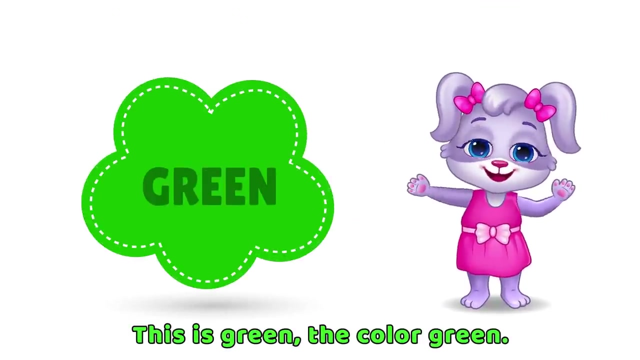 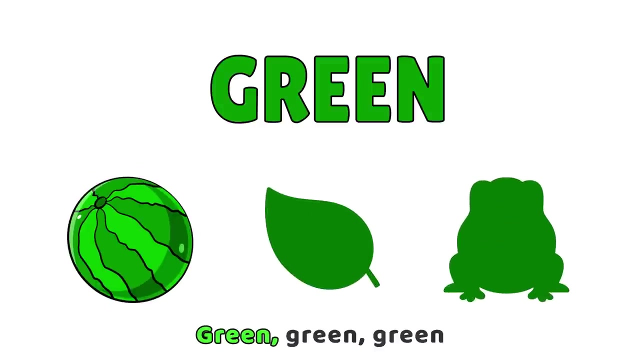 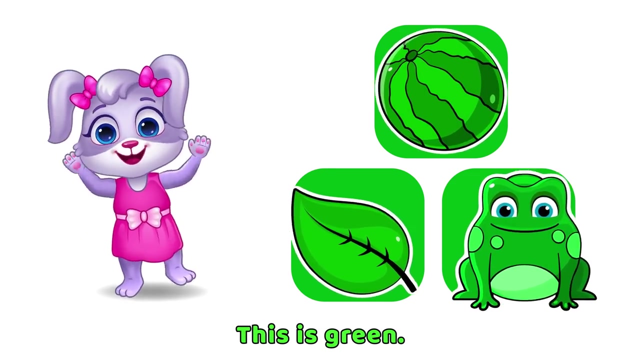 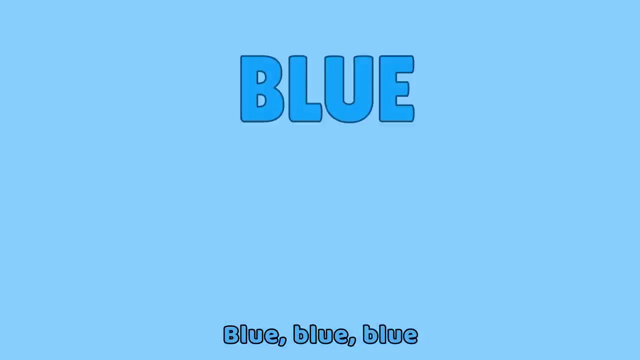 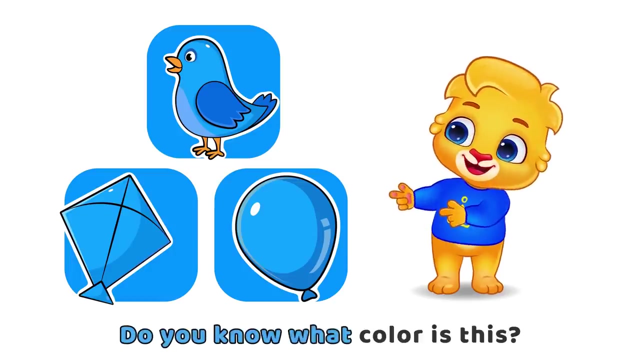 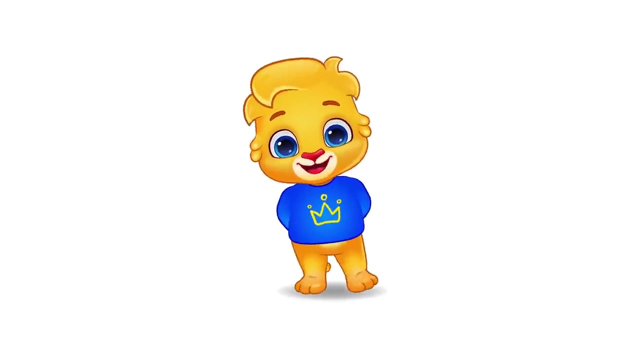 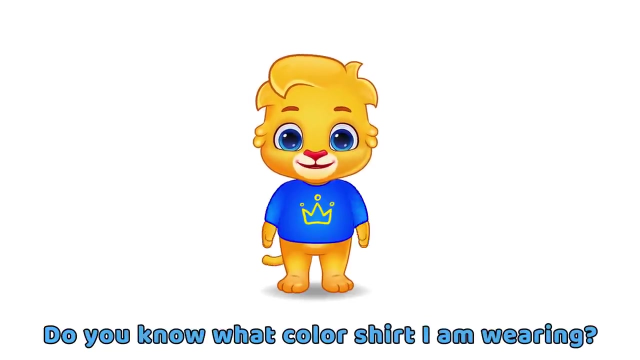 One, Two, Three, Two, Three, Two, Two, Three, Two, Two, Three, Two, Two, One, Two, Three, Two, Two, Three, Two, Three, Two, Two, Two, Three, Two. This is blue. Hey, Do you know what color shirt I'm wearing? Hmm, It's the color blue, Blue, Great. 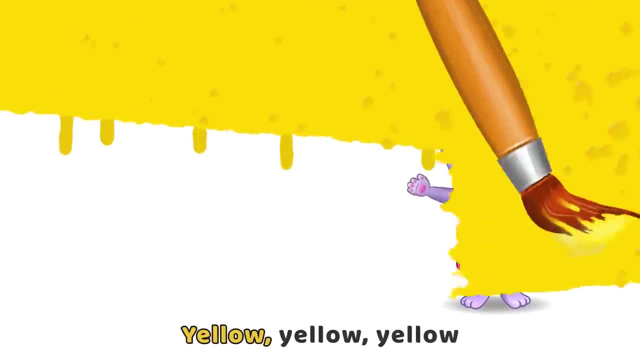 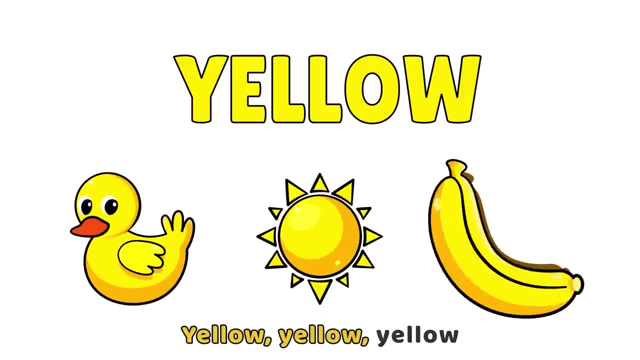 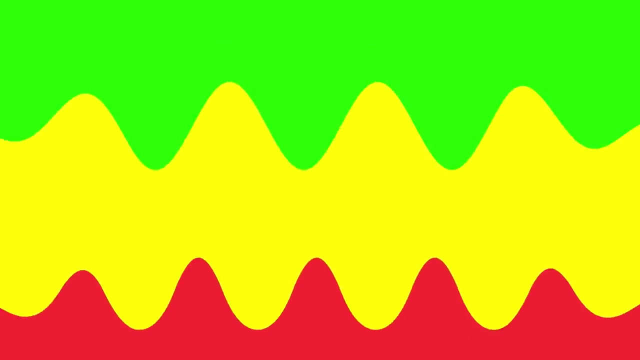 This is yellow. the color yellow, yellow, yellow, yellow. This is yellow, the color yellow, yellow, yellow, yellow. Do you know what color this is? This is yellow. Hey, Can you tell me what color these things are? 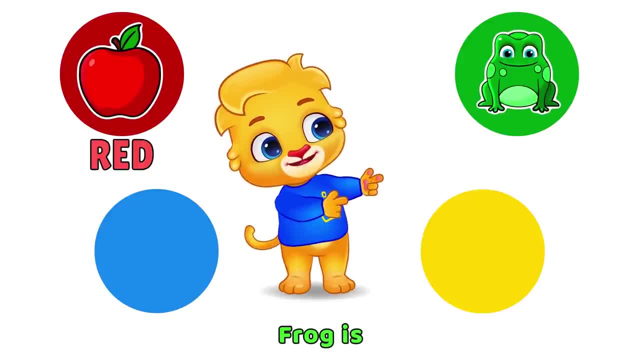 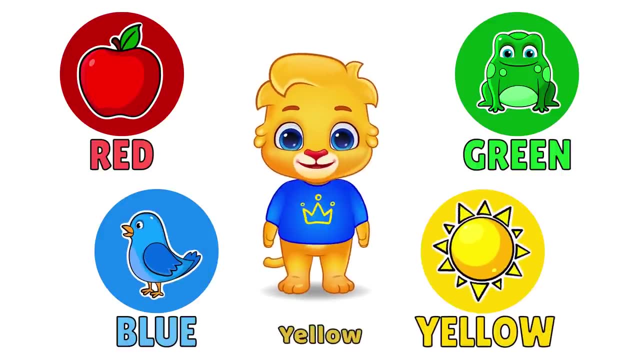 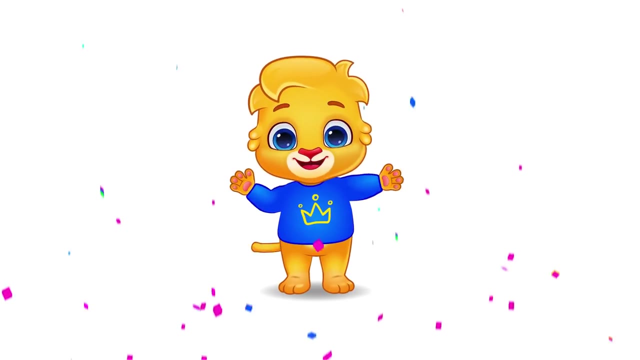 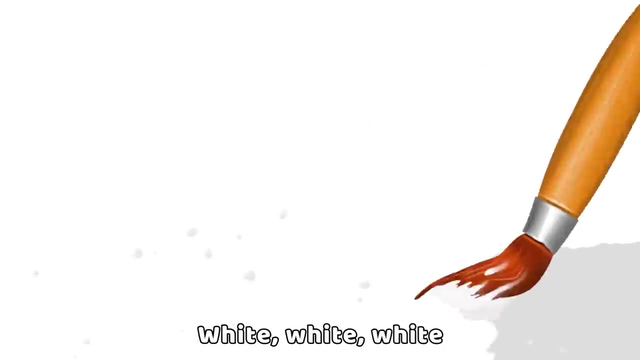 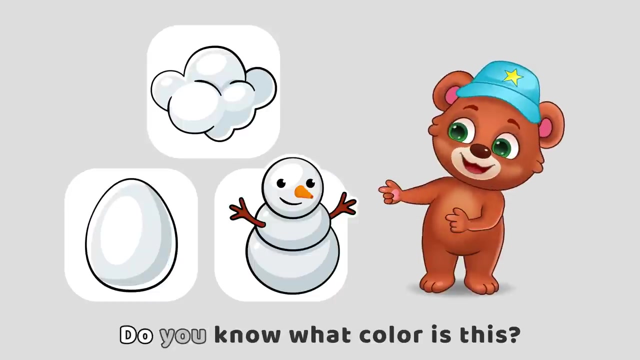 Apple is red, Frog is green, Bird is blue, Sun is yellow, White. Great Woohoo, Yeah, This is white, the color white, white, white, white. This is white, the color white, white, white, white. 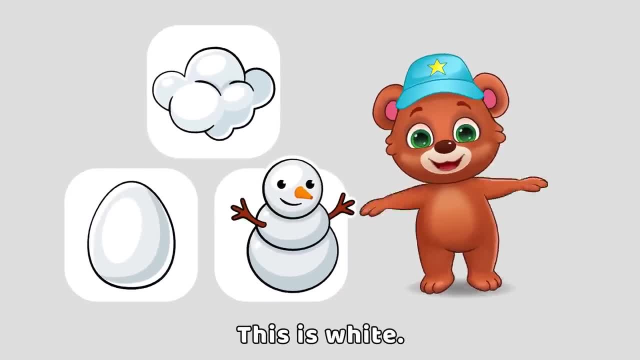 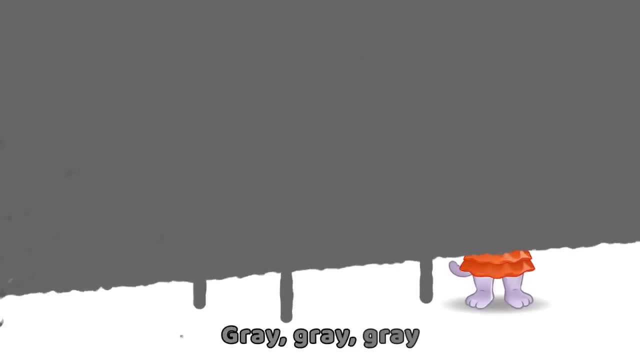 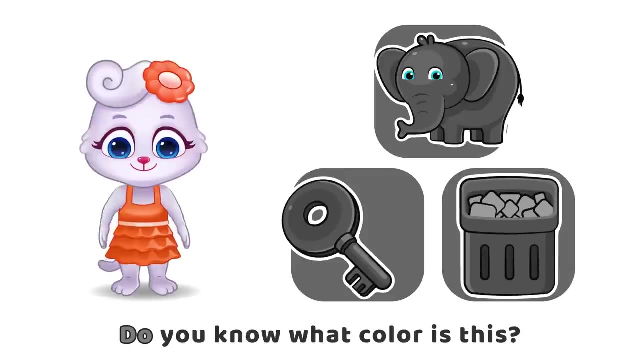 Do you know what color this is? This is white. This is gray: the color. gray, gray, gray, gray. This is gray, the color. gray, gray, gray, gray. This is gray: the color. gray, gray, gray, gray, gray. 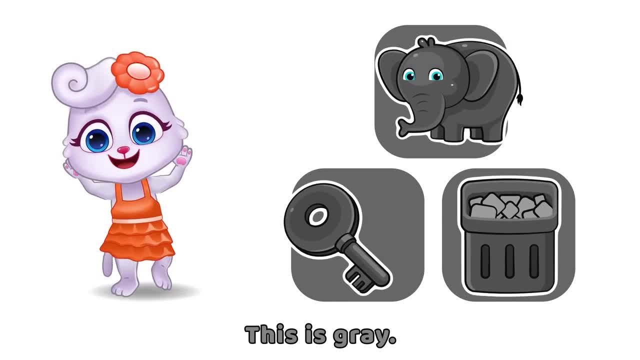 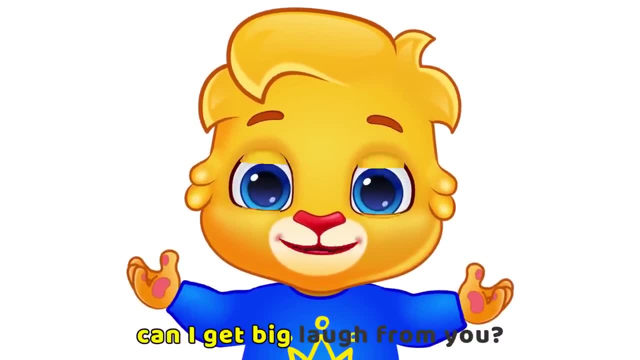 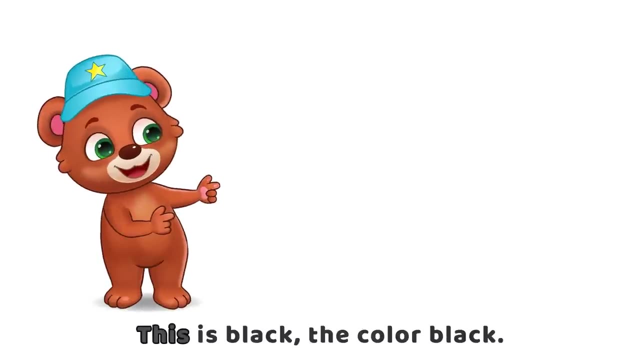 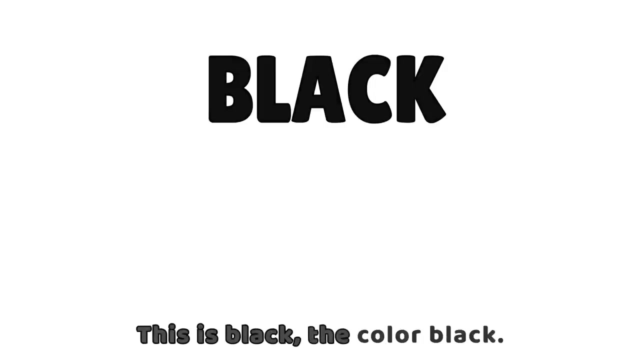 Do you know what color this is? This is gray. Hey, my friend, Can I get a big laugh from you? This is black. the color black. black, black, black. This is black, the color black. black, black, black. 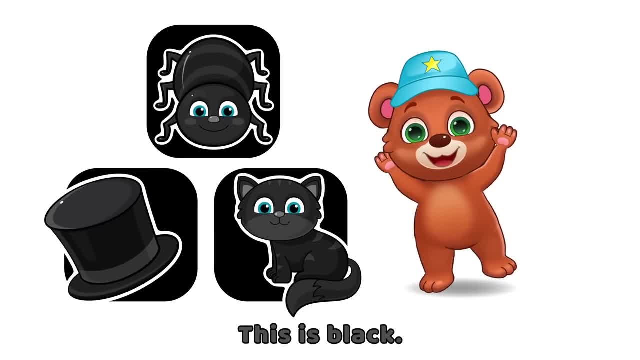 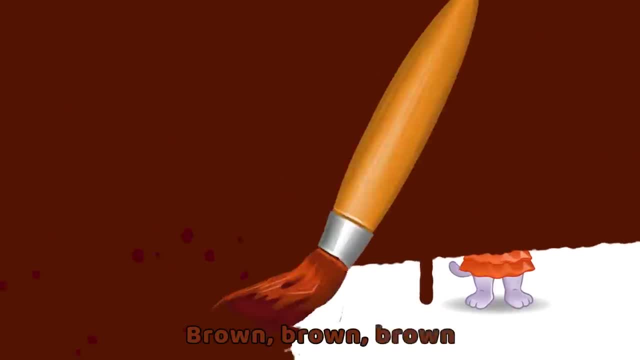 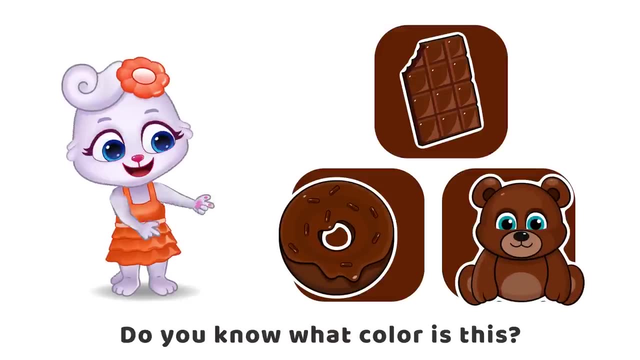 Do you know what color this is? This is black. This is brown. the color brown: brown, brown brown. This is brown. the color brown: brown, brown brown. Do you know what color this is? This is brown. 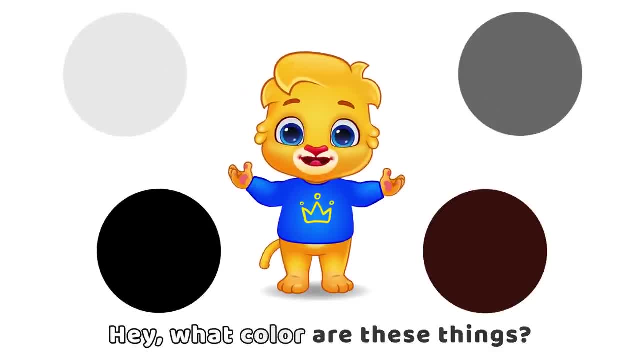 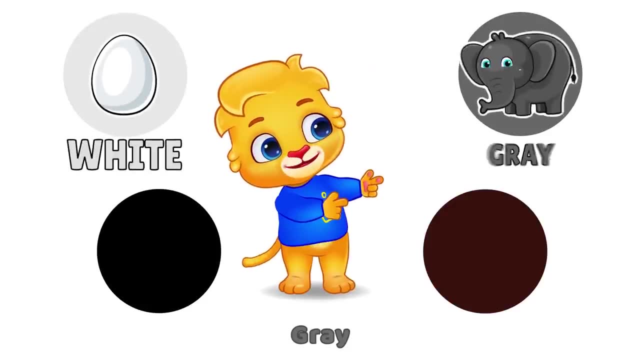 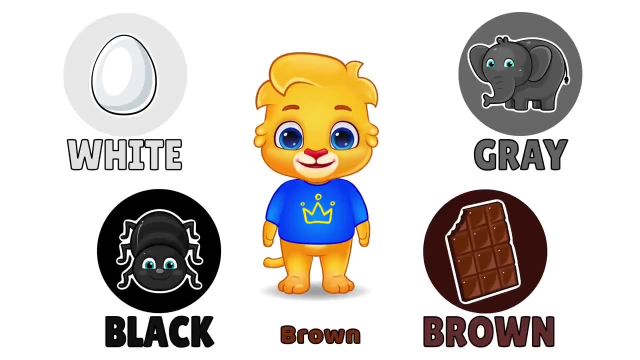 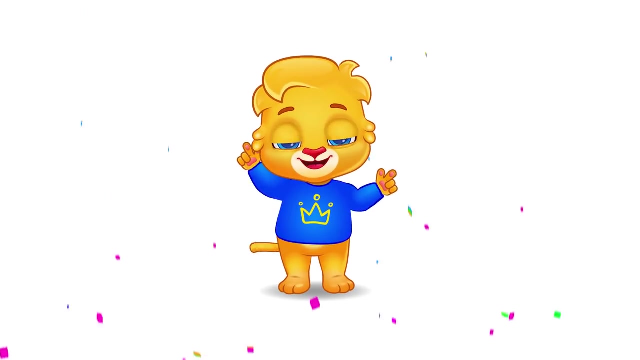 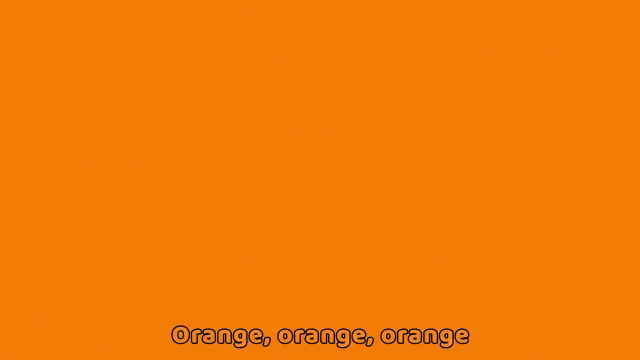 Hey, what color are these things? Do you know? Egg is white, Elephant is gray, Spider is black, Chocolate is brown, Superb, Woohoo. This is orange, the color orange, orange, orange. This is orange orange. this is orange, the color orange, orange, orange, orange. 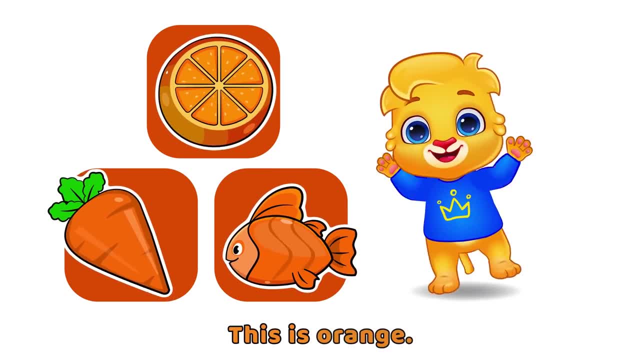 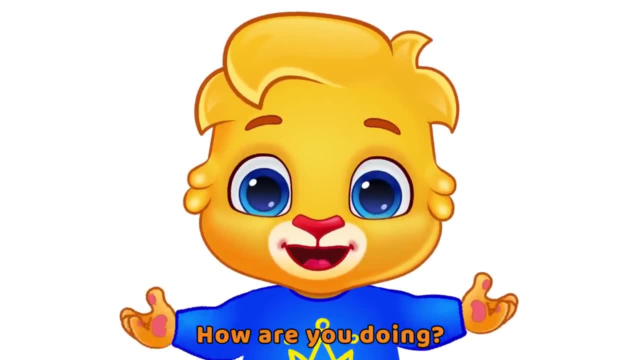 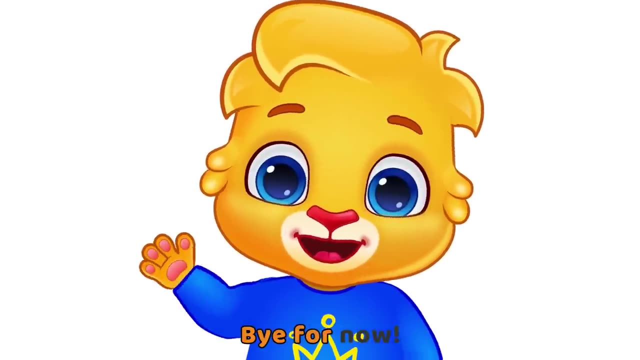 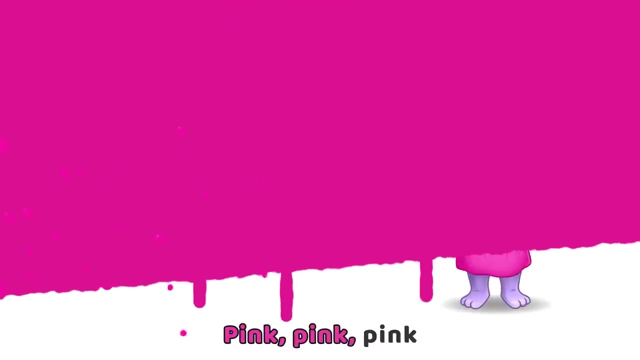 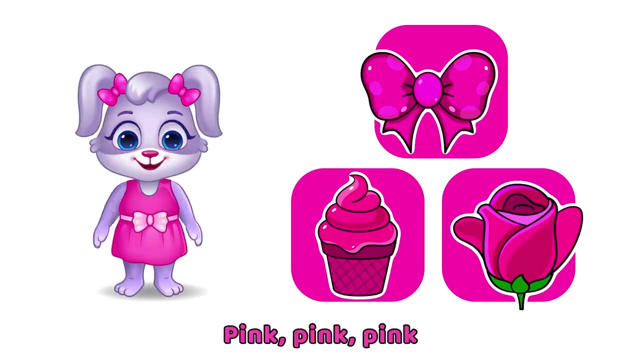 Do you know what color this is? This is orange. Hi, how are you doing? Wanted to say hi, Bye for now. This is pink, The color pink, pink, pink, pink. This is pink, the color pink, pink, pink, pink. 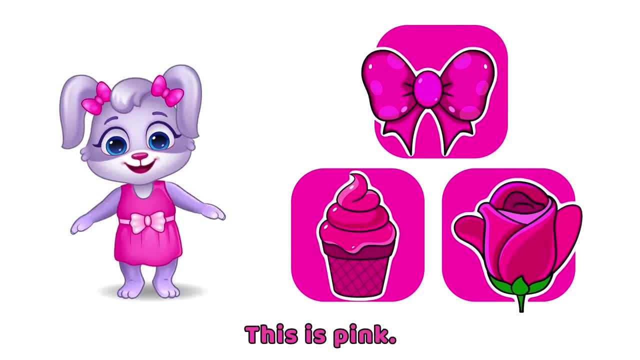 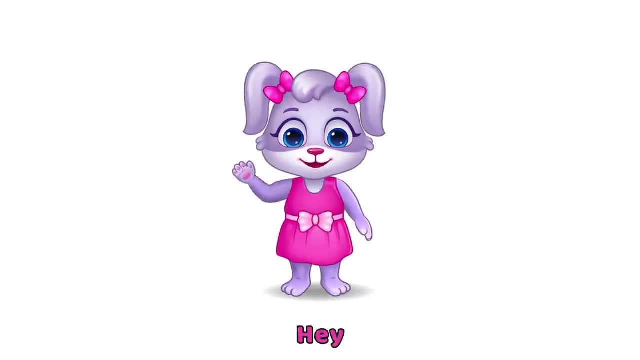 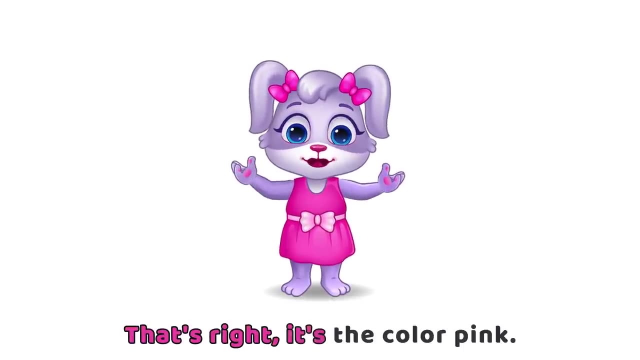 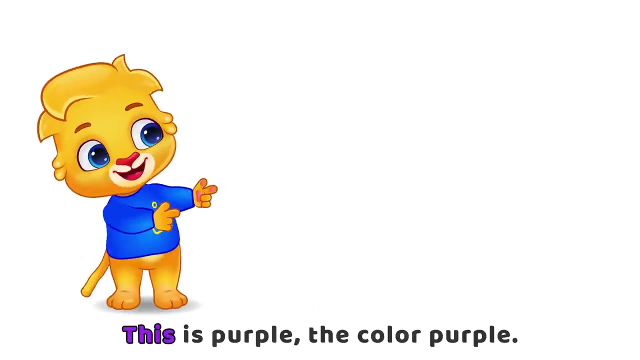 Do you know what color this is? This is pink. Hey, what color am I wearing now? Hmm, that's right, It's the color pink, Pink, pink, Well done, This is purple, the color purple, purple, purple, purple. 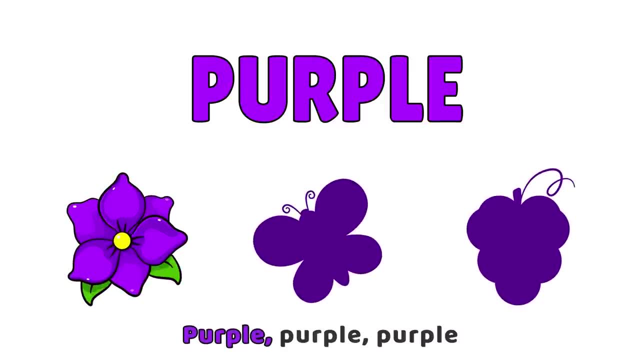 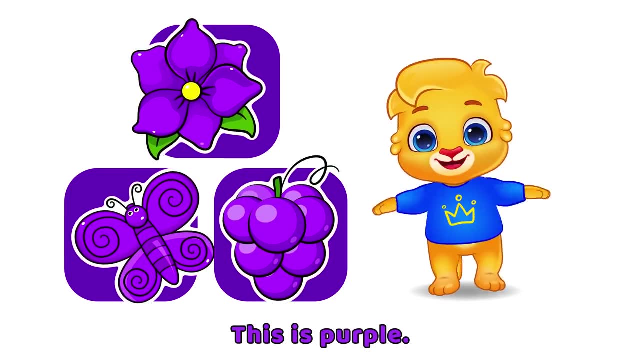 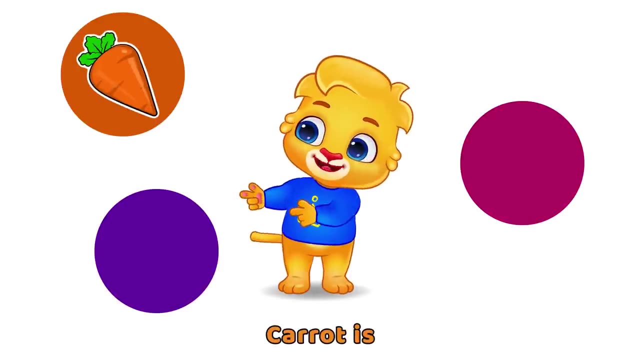 This is purple, the color purple, purple, purple, purple. Do you know what color this is? This is purple. Hey, can you tell me what color these things are? Carrot is Orange, Bow is Pink, Grapes are. 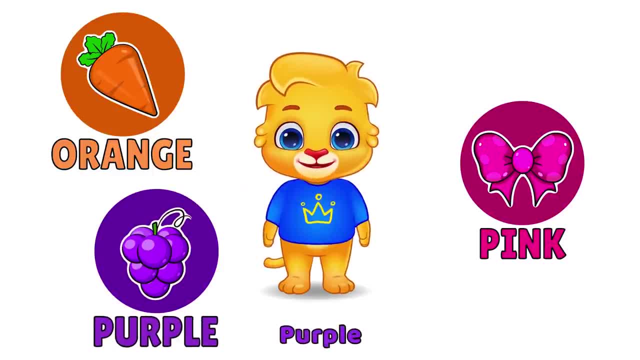 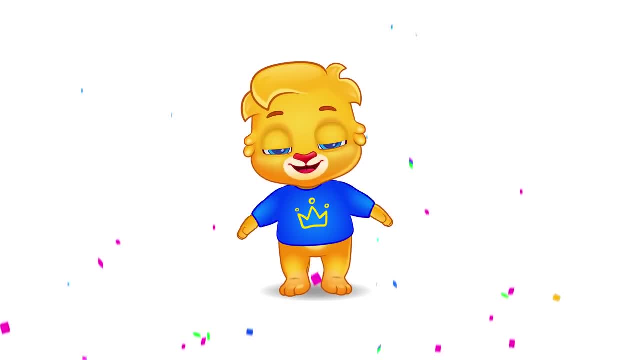 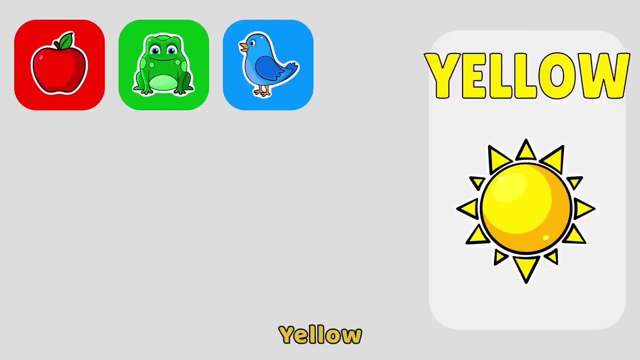 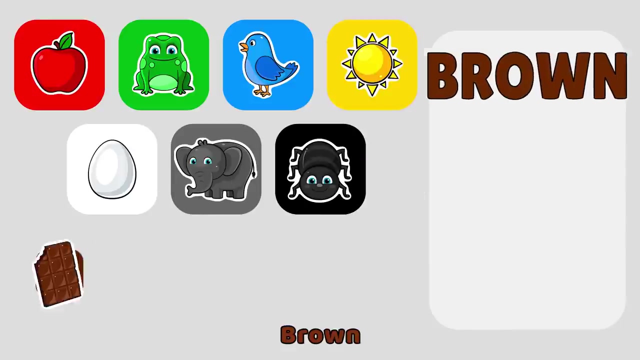 Purple, Awesome Woo-hoo. Red, Green, Blue, Yellow, White, Gray, Black, Brown, Orange, Pink, Yellow, White, Gray, Black, Brown, Orange, Pink, Yellow, Blue, Orange, Pink, Yellow. 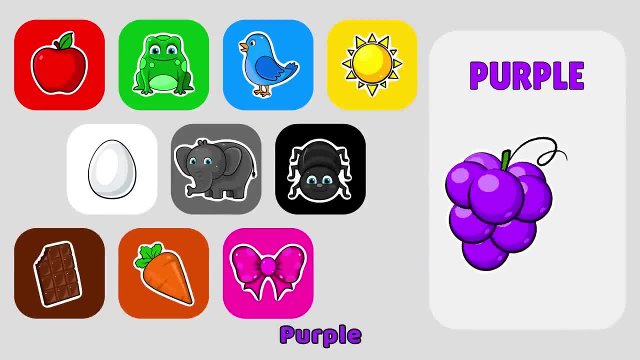 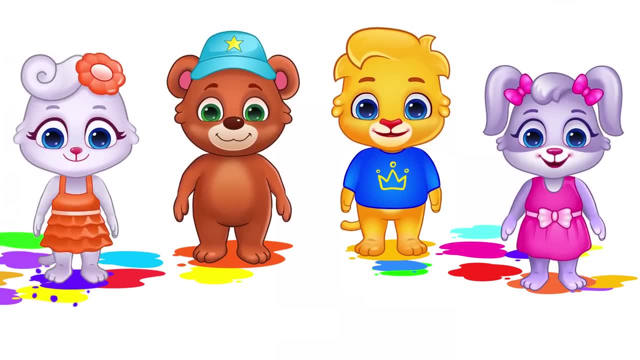 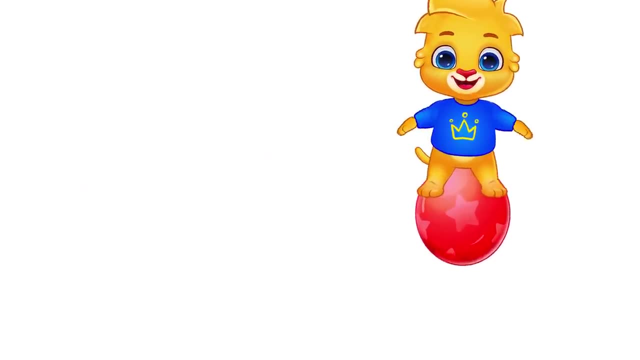 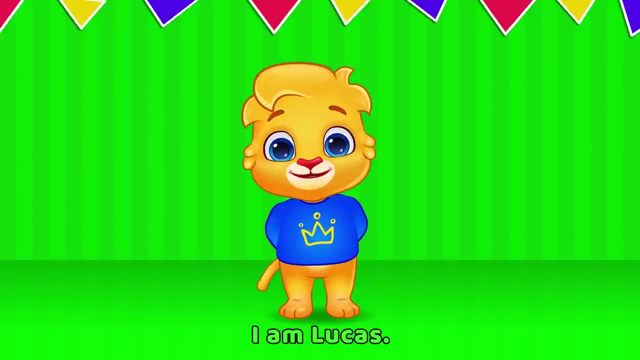 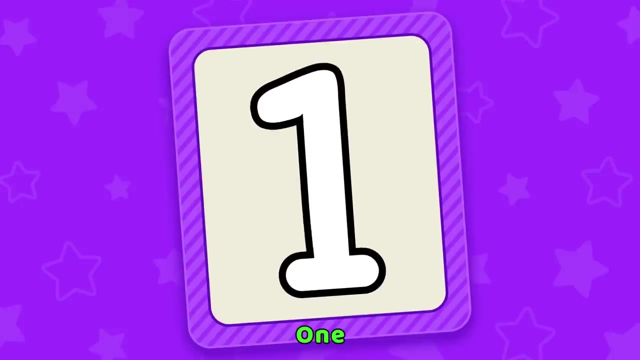 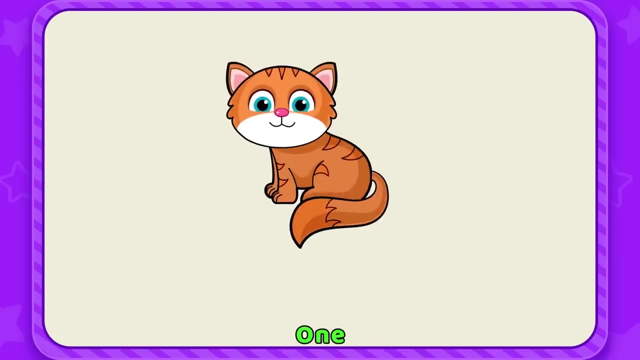 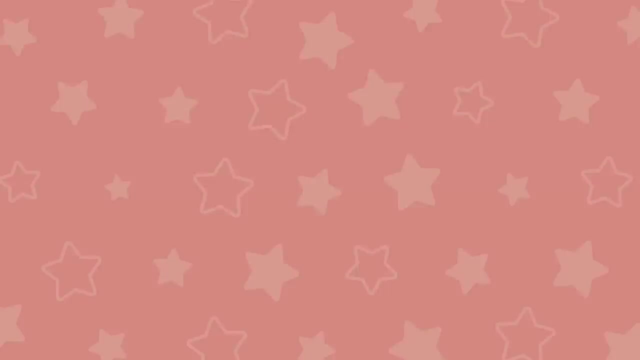 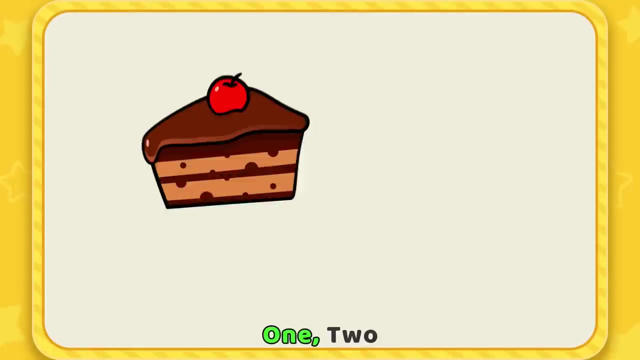 Orange, Pink, Pink, Purple, Purple, Whoa-hoo, Yeah, Whoo-hoo, Hey, kids, I am Lucas. Today we're going to learn numbers and counting. Whoo-hoo, One, One, one, one cat, two, two, one, two, two pastries. 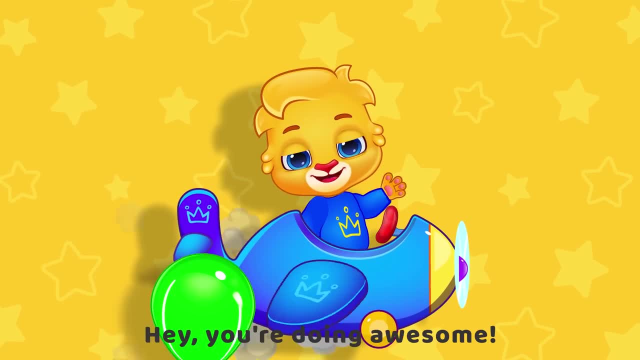 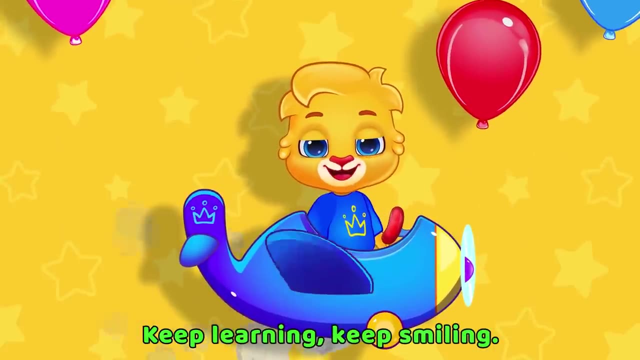 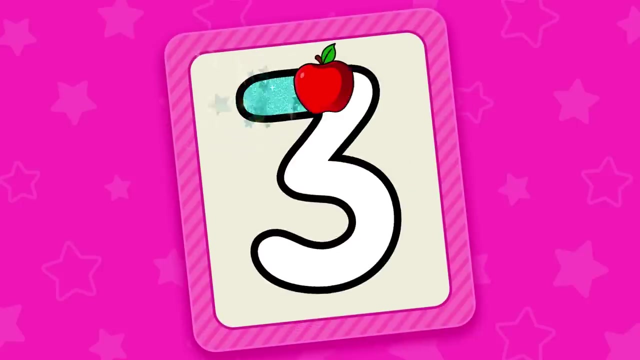 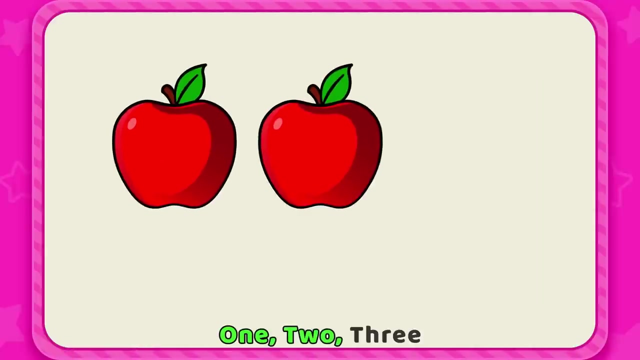 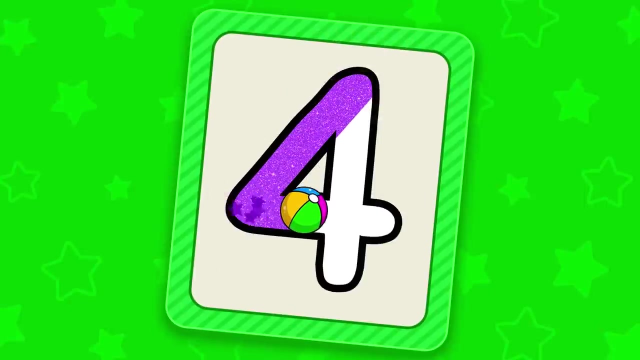 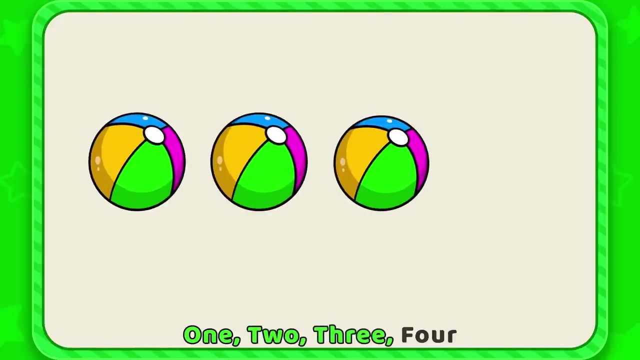 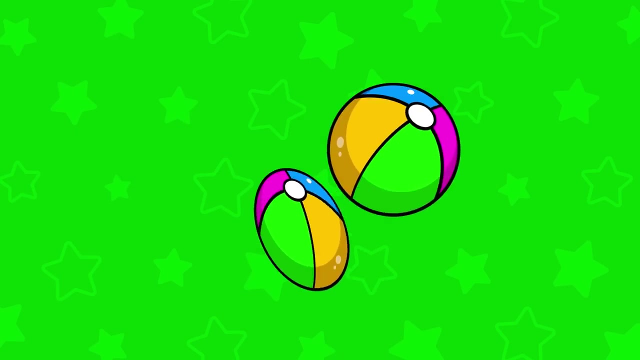 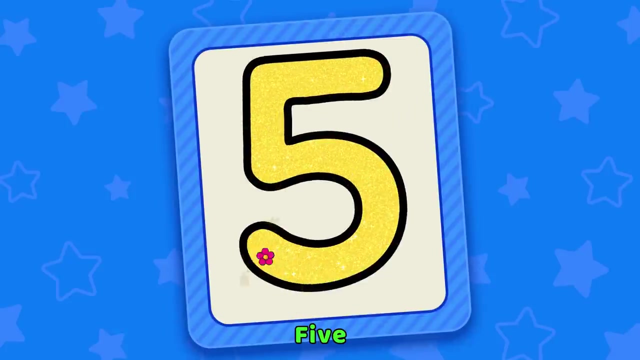 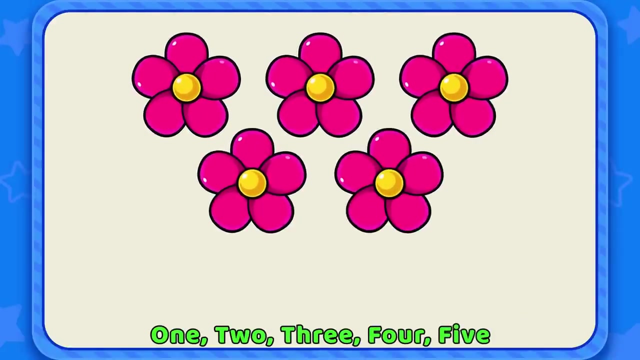 Hey, you're doing awesome, Keep learning, keep smiling. Three: Three, One, two, three, Three. apples Four: One, two, three, four, four. balls Five: Five: One, two, three, four, five. 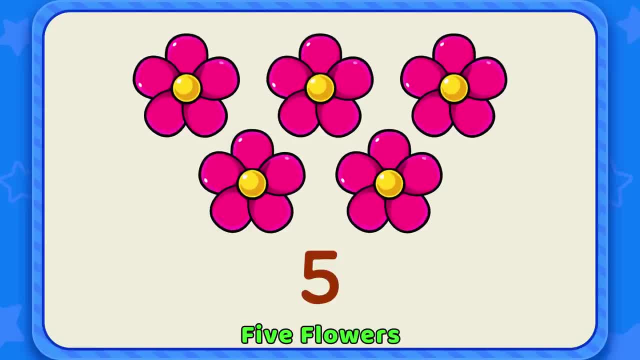 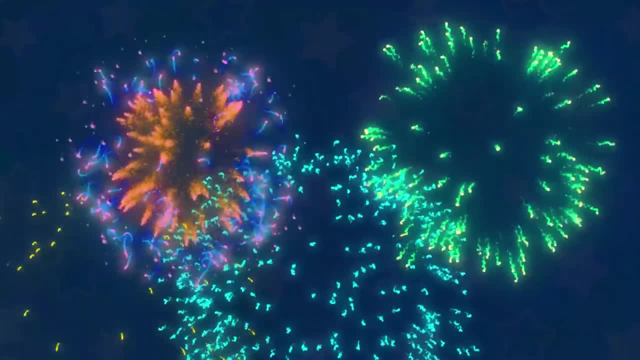 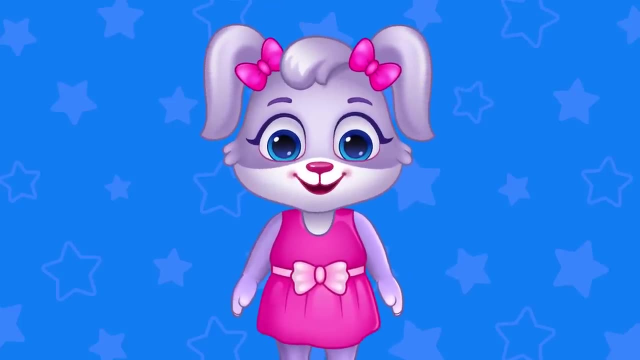 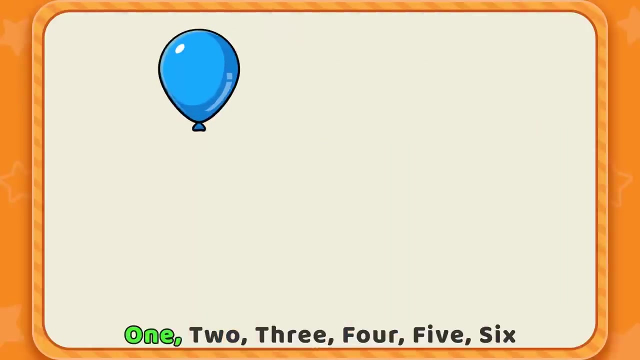 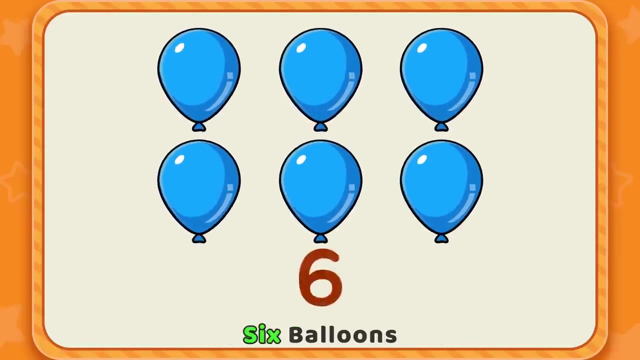 Five flowers, Wonderful Six. One, two, three, four, five, Six. One two, three, four, five Six球 Six. Six One, two, three, four, five, Six, Six, Six balloons. 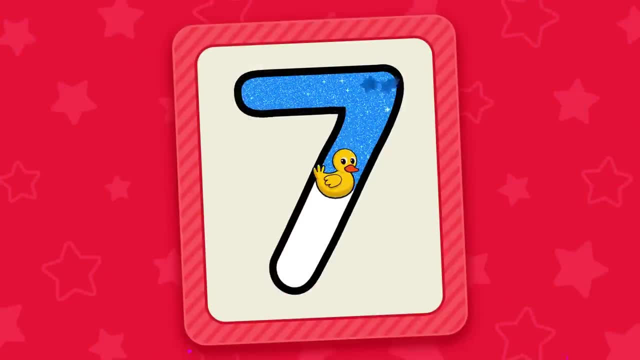 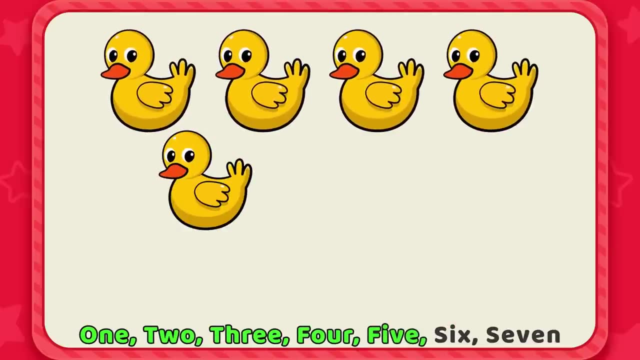 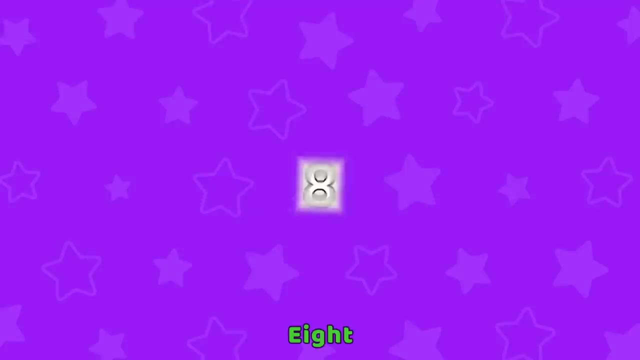 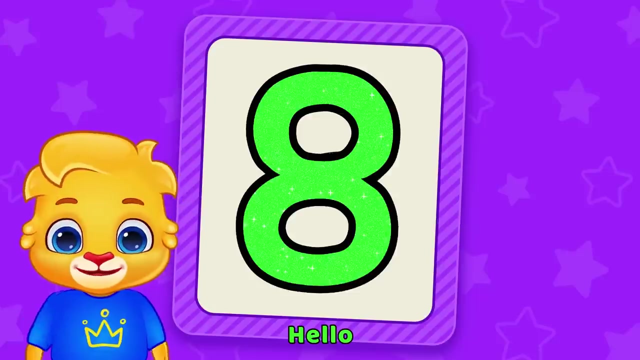 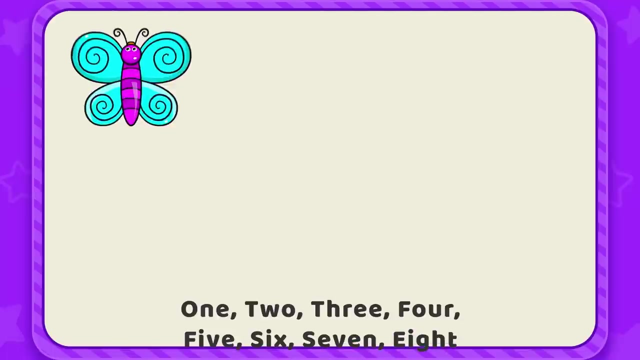 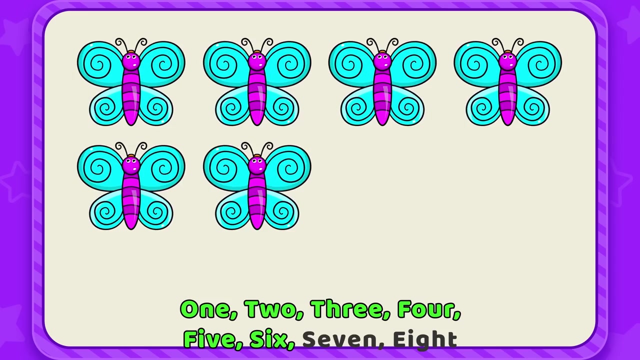 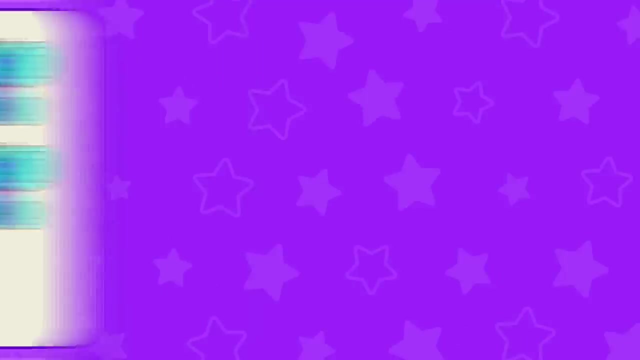 Seven, Seven. One, Two, Three, Four, Five, Six, Seven, Seven ducks Eight, Hello, What's this? Eight, One, Two, Three, Four, Five, Six, Seven, Eight, Eight butterflies, Nine. 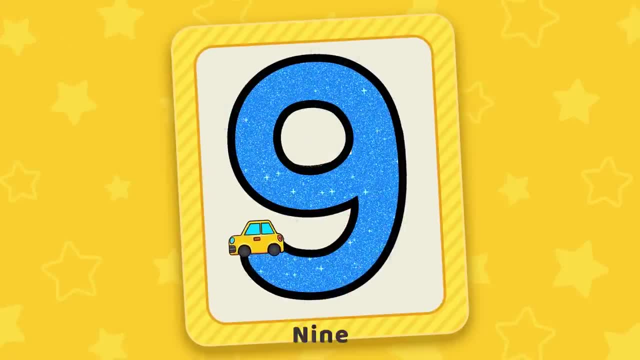 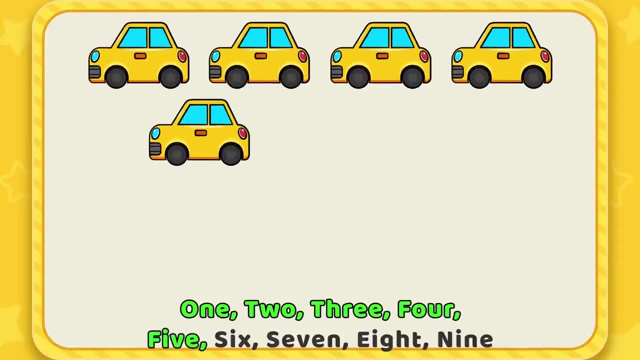 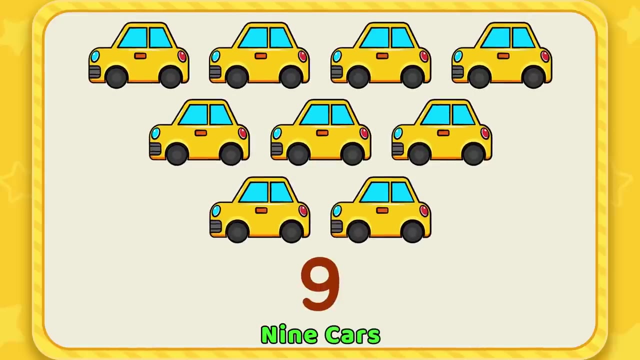 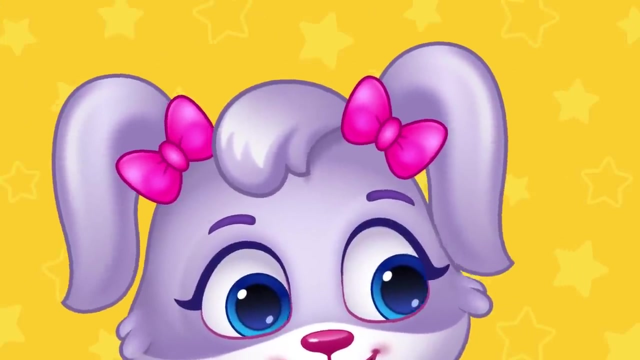 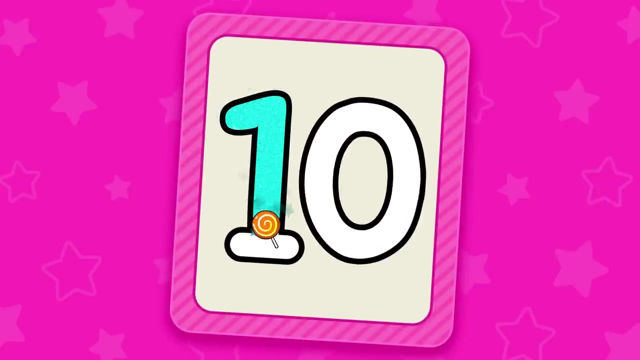 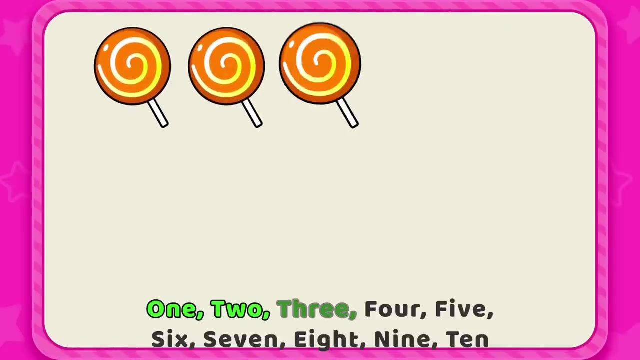 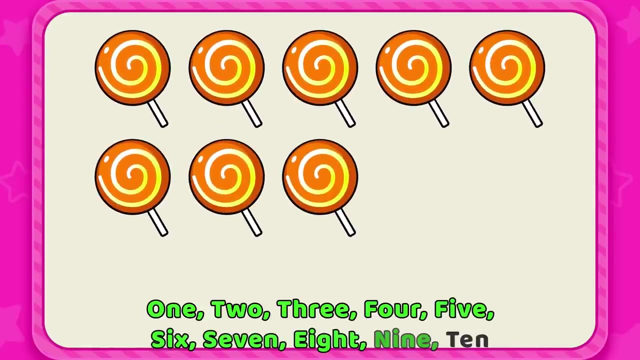 Nine, Nine. One, Two, Three, Four, Five, Six, Seven, Eight, Nine Nine cars: Ten: Two. One, Two, Three, Four, Five, Six, Seven, Eight, Nine, Ten, Ten candies. 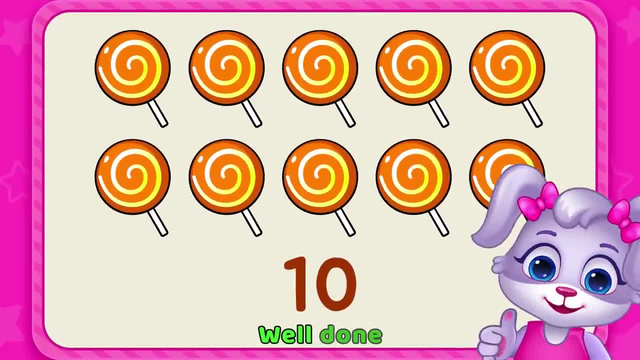 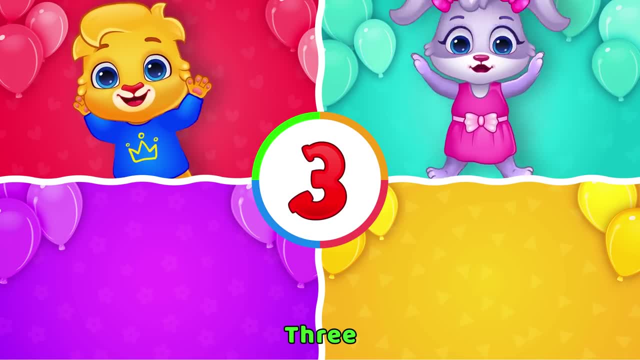 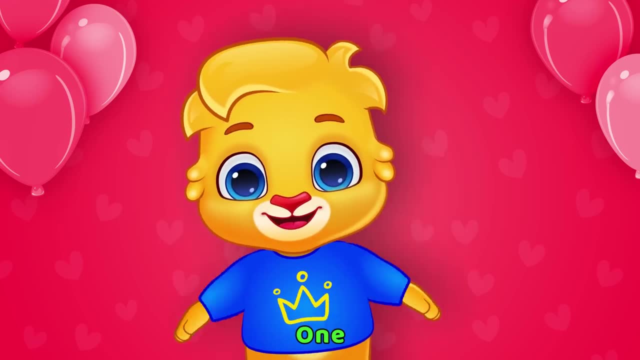 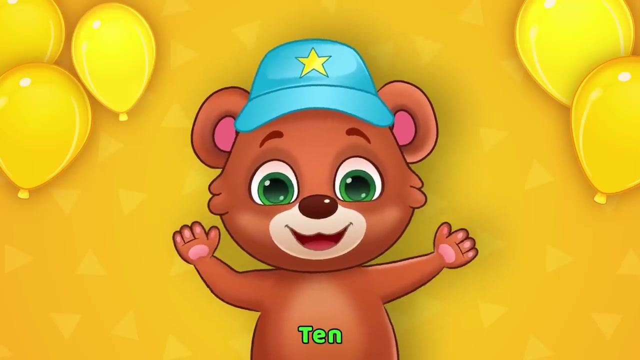 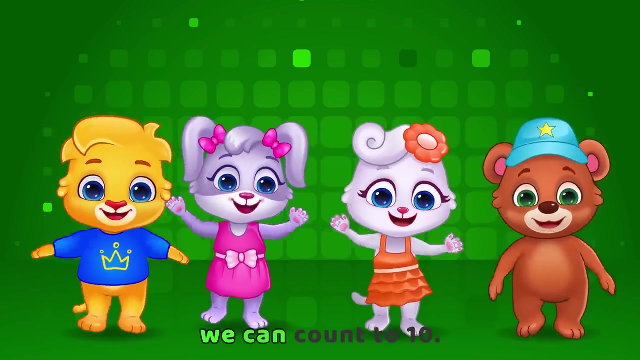 Well done: One, Two, Three, Four, Five, Six, Seven, Eight, Nine, Ten, Ten candies, Well done: One, Two, Three, Four. One, two, three, four, five, six, seven, eight, nine and ten. You and I, my friend, we can count to ten. 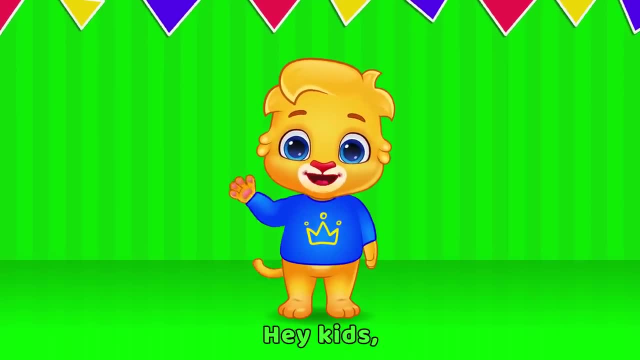 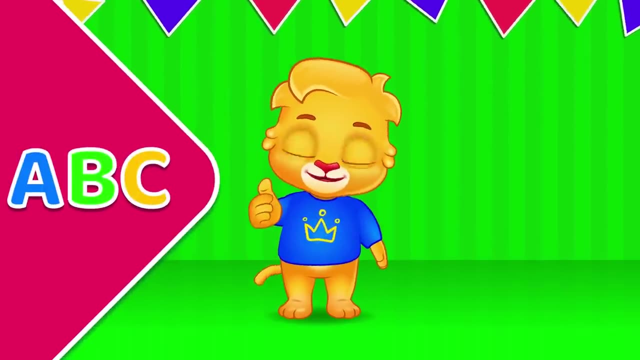 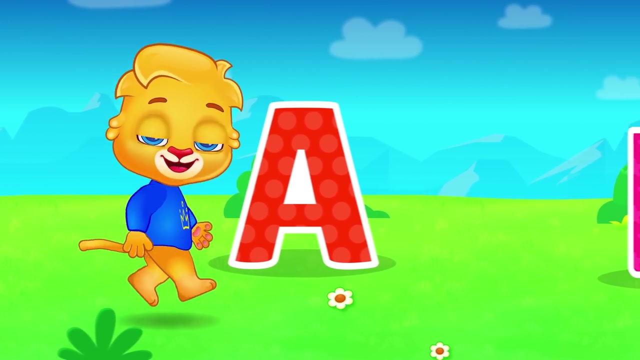 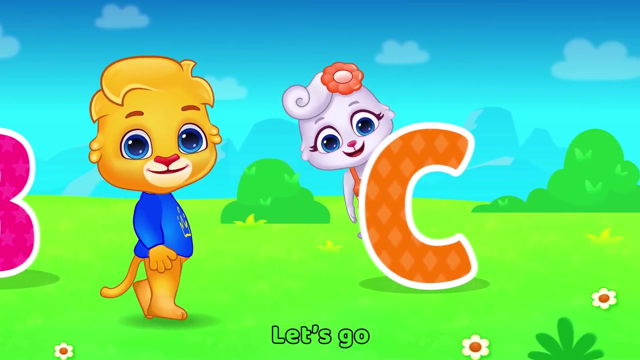 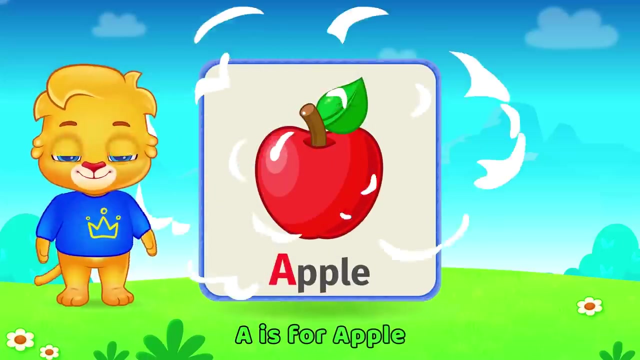 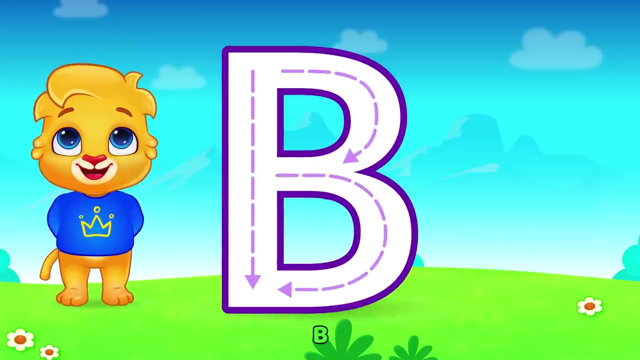 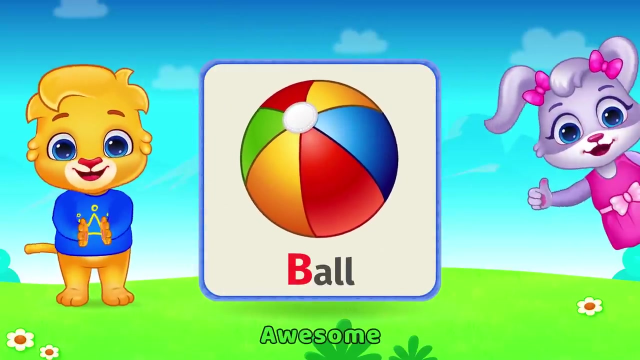 Hey kids, I am Lucas and today I am going to teach you the A, B, Cs. Woo-hoo, Hi, Hello, Let's go. Hey, A is for apple, B B is for ball- Awesome. 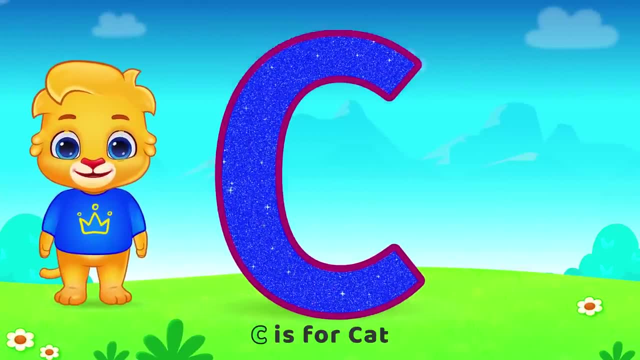 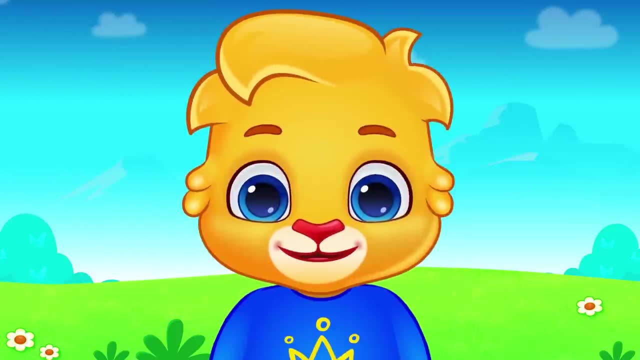 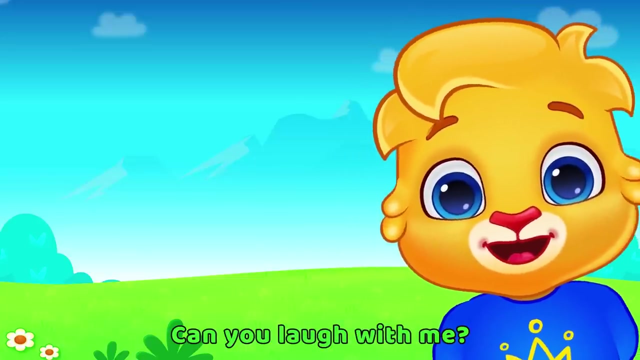 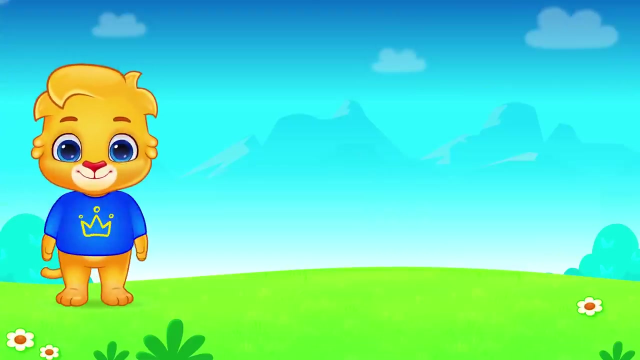 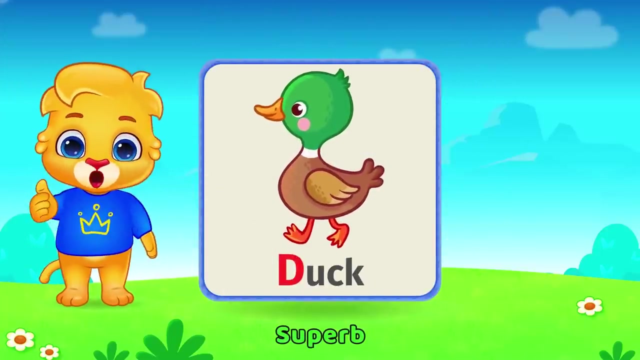 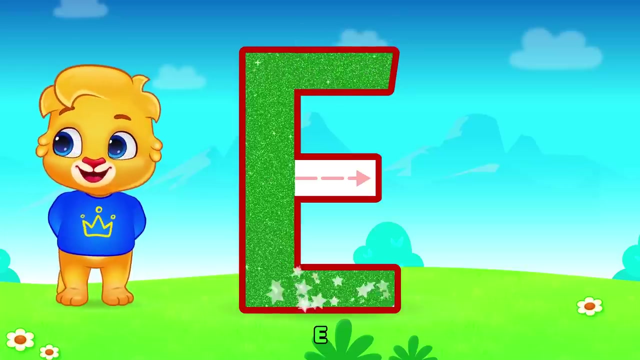 C. C is for cat, Woo-hoo, Hi, I'm back again. Can you laugh with me, Ha-ha-ha. D, D is for duck Superb, E, E, E is for elephant, Hi-oh. 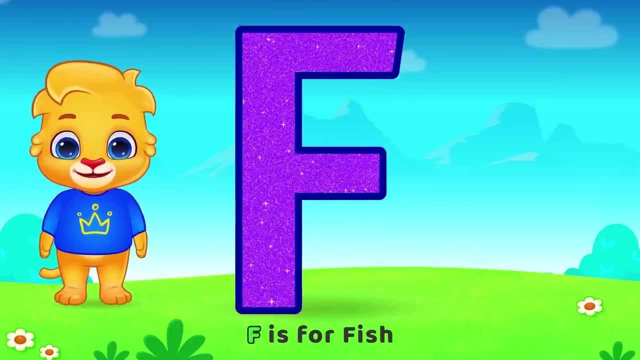 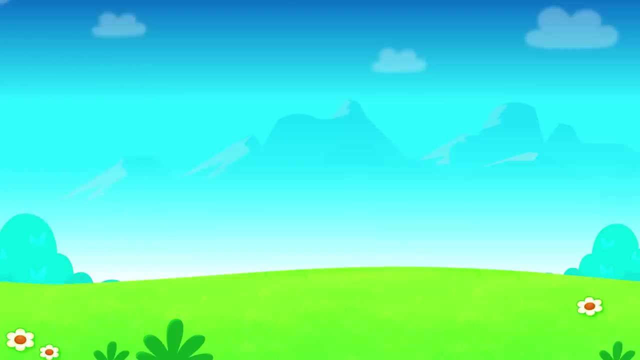 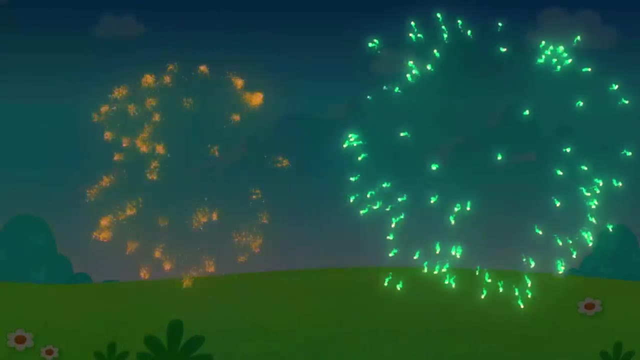 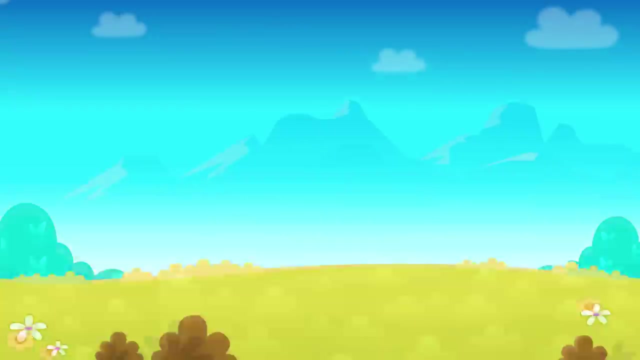 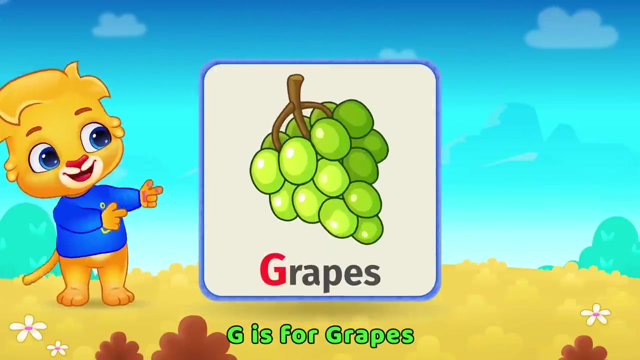 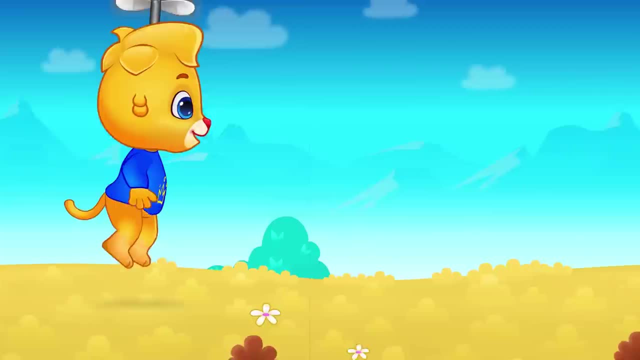 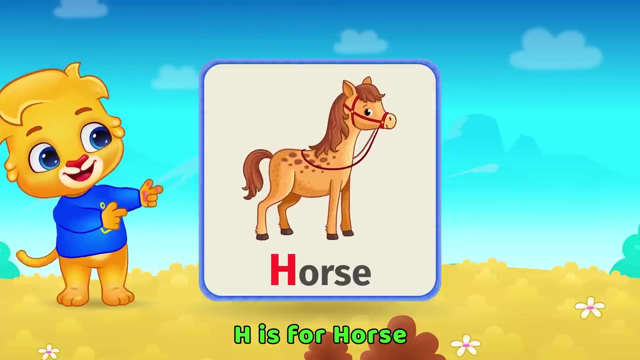 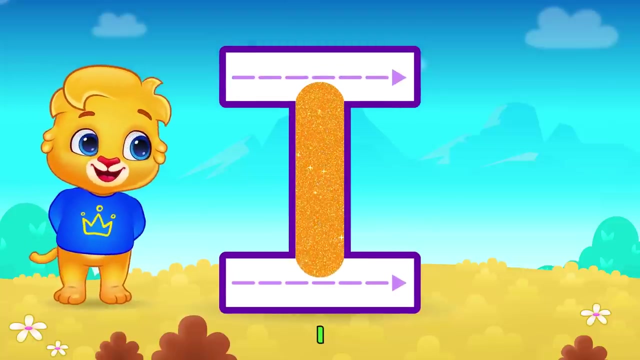 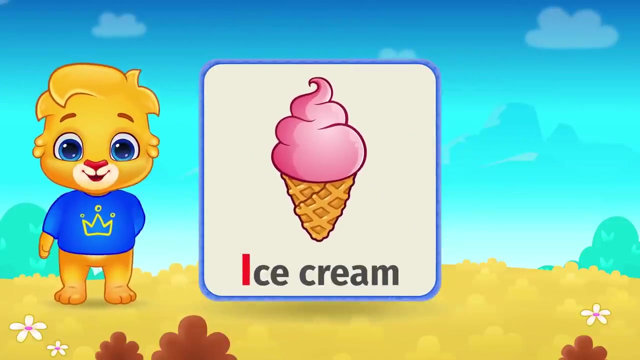 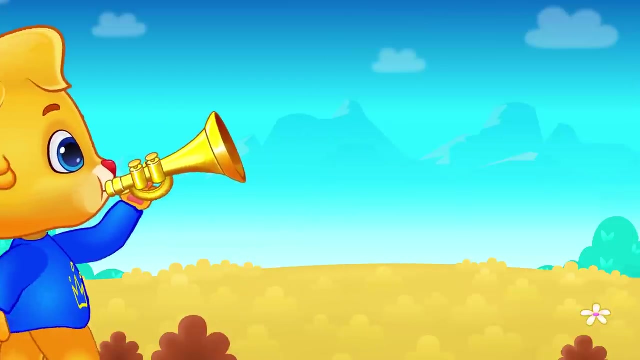 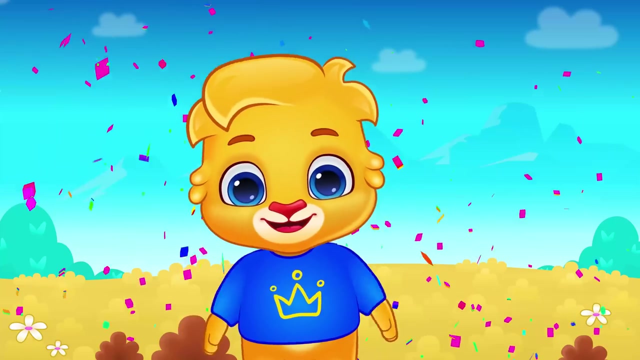 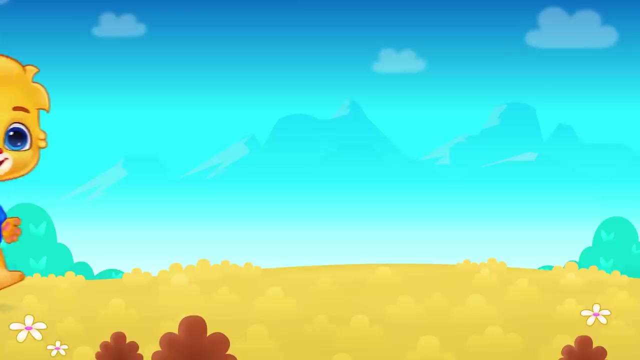 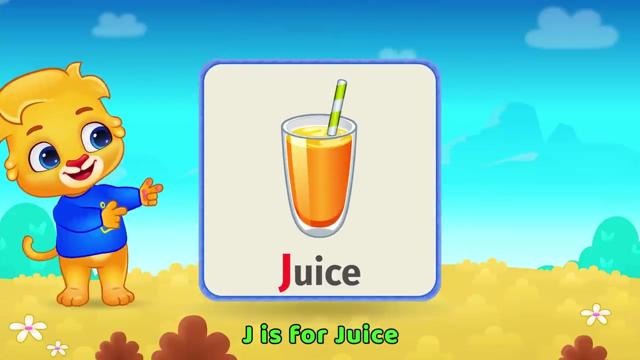 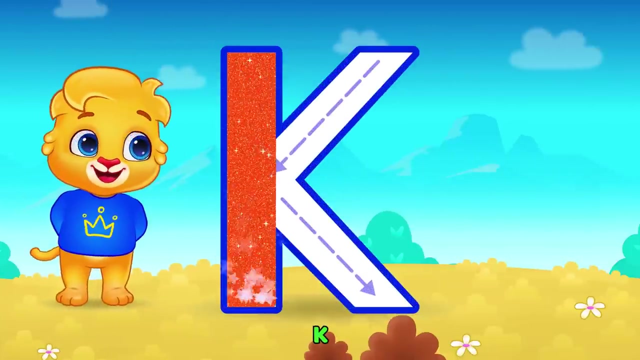 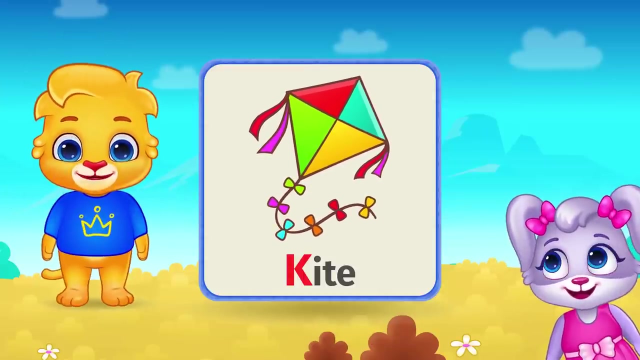 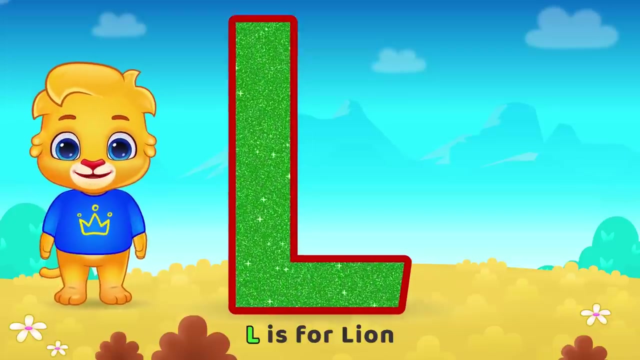 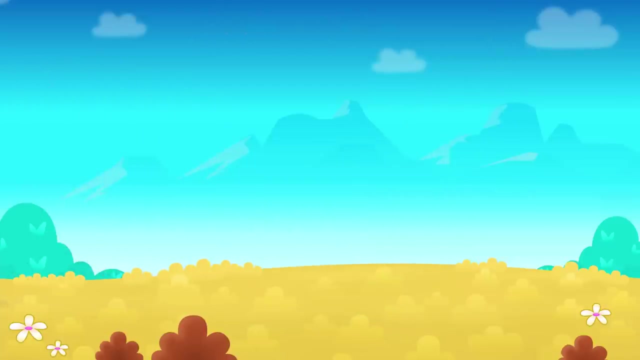 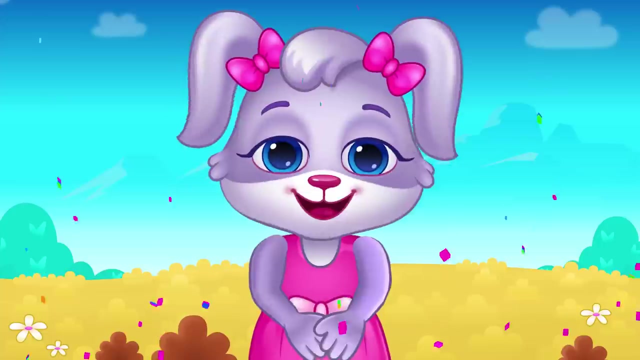 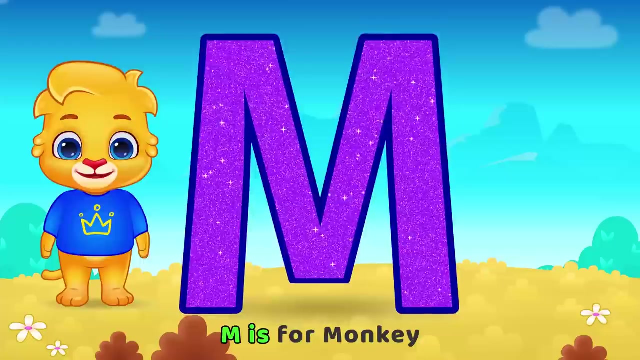 Woo-hoo, H. H is for horse, Great job, I. I is for ice cream, hello, my friend J is for juice. K K is for kite, L is for lion, grateful. El Al is for lion, great, great, great. Oh. M is for monkey. 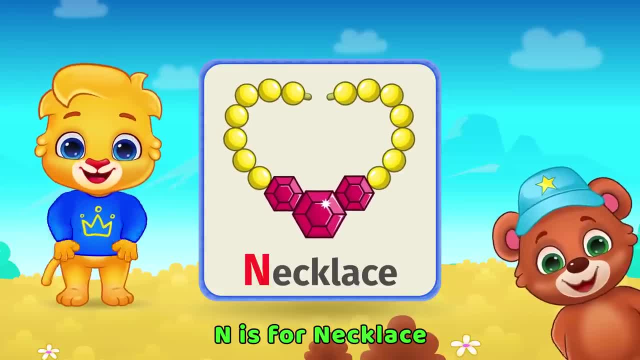 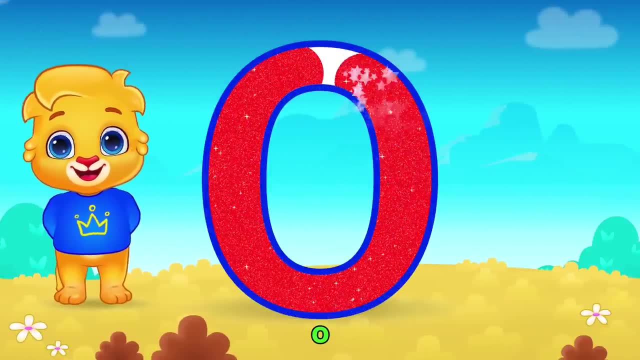 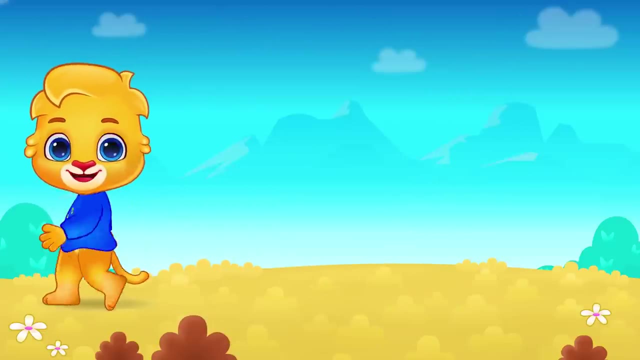 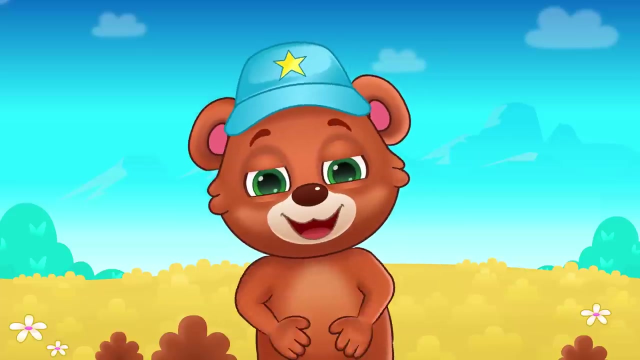 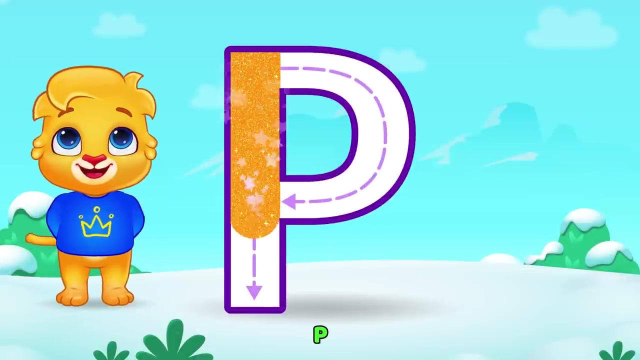 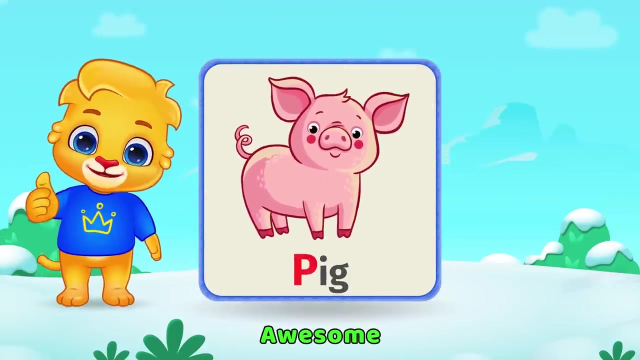 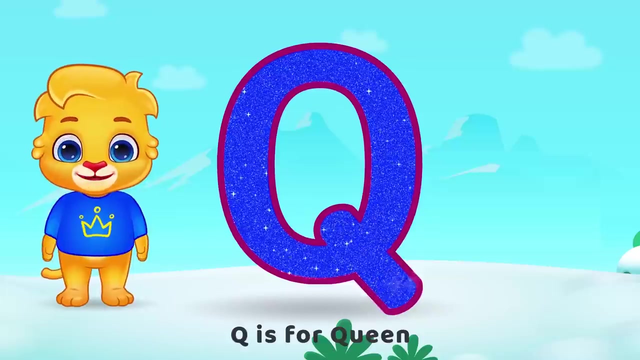 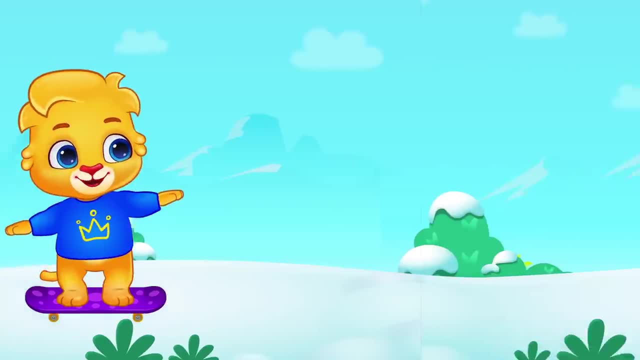 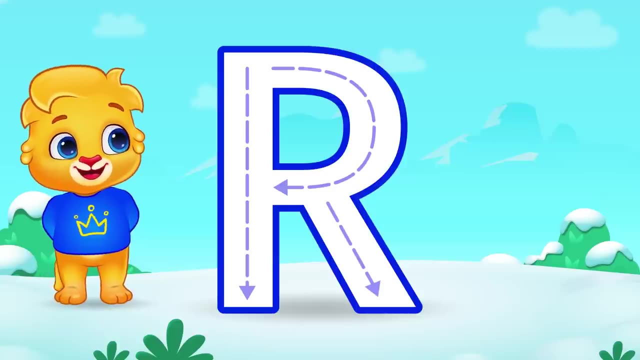 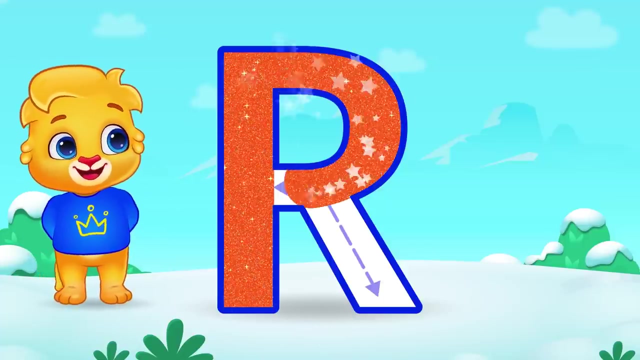 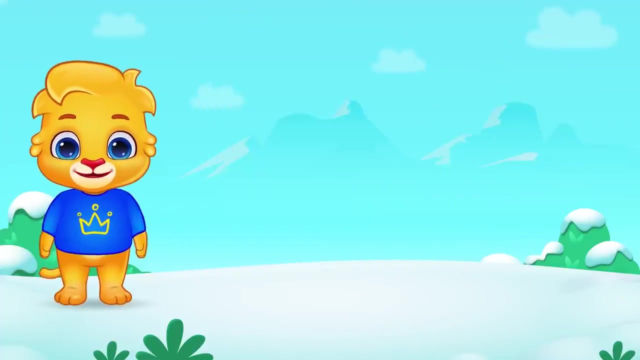 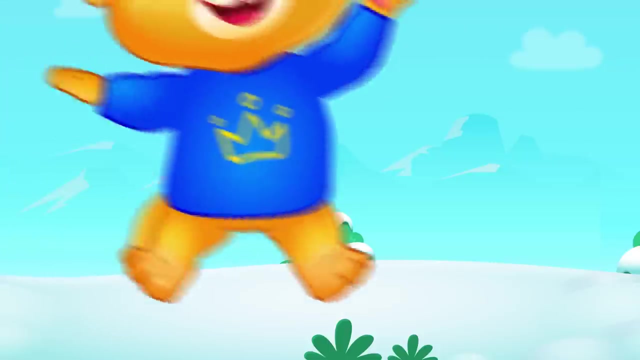 Yay S, No, no, no, no, no, no. R R Great R is for RABBIT, S S is for SUN. Woohoo, Hi, Hi. How are you? How are you doing? 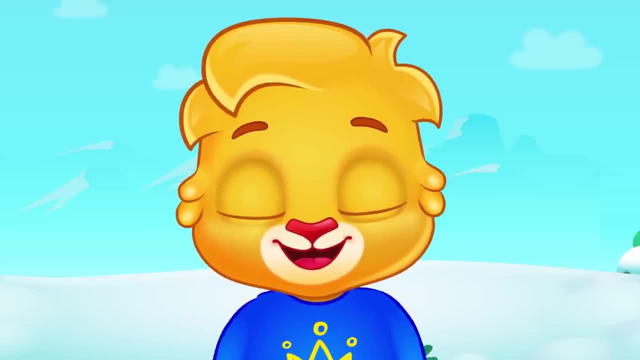 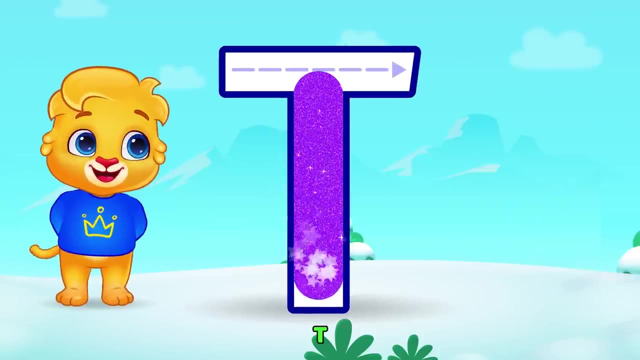 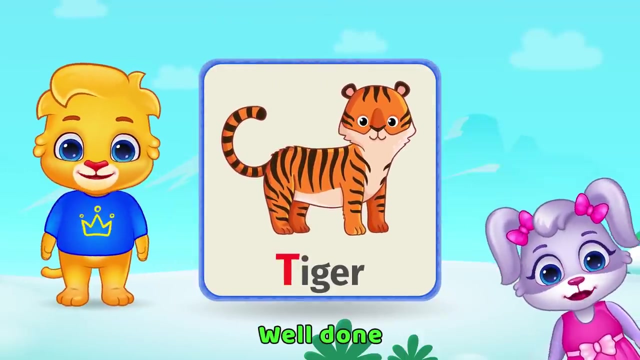 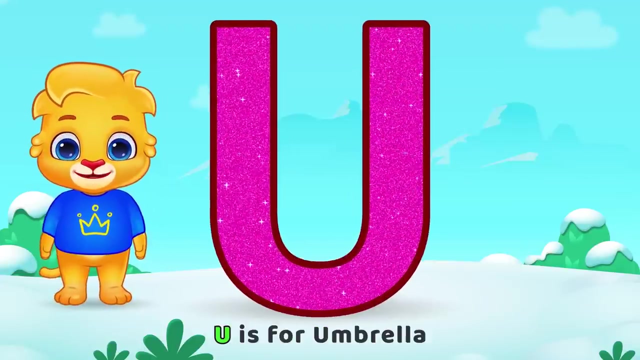 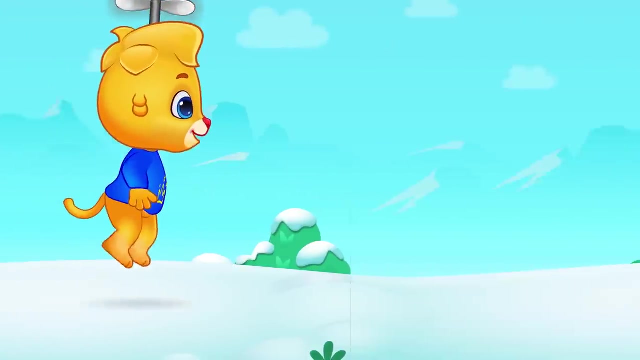 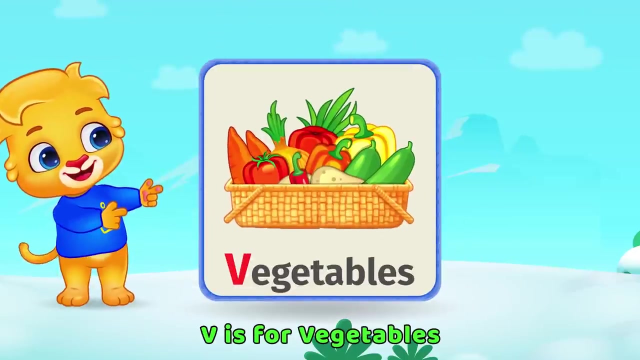 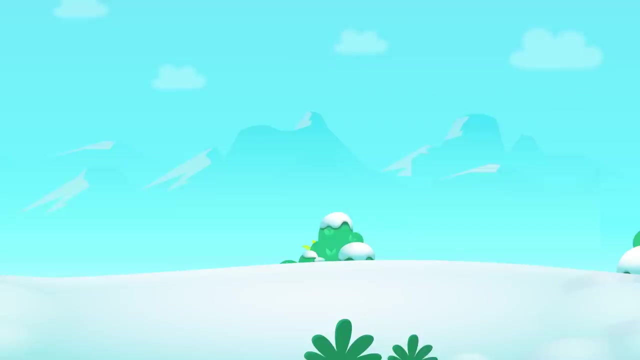 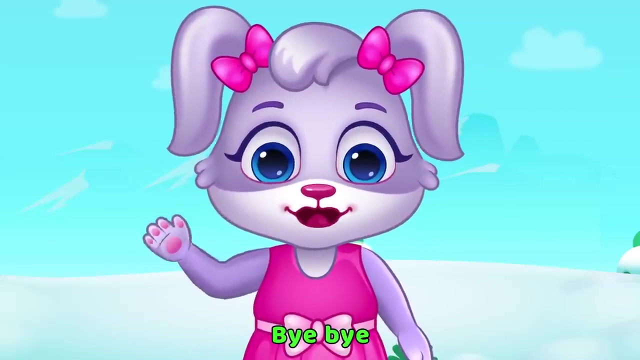 Wanted to say hi, Bye for now. T. T is for TIGER, Well done, U. U is for UMBRELLA, V, V is for VEGETABLES. Hello, Hello, Hello, Bye, Bye. 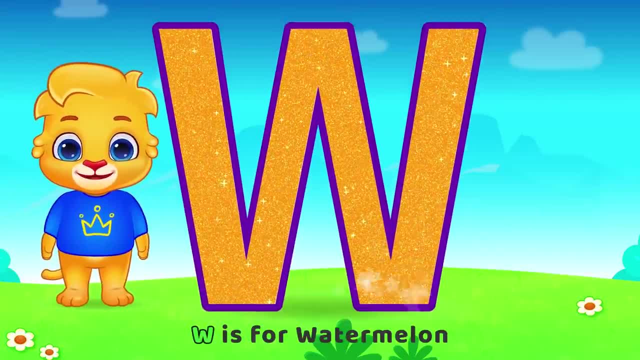 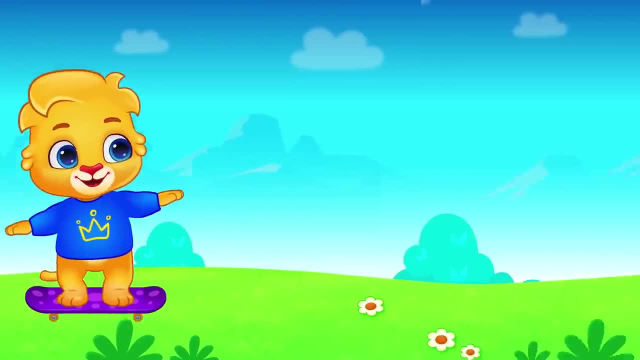 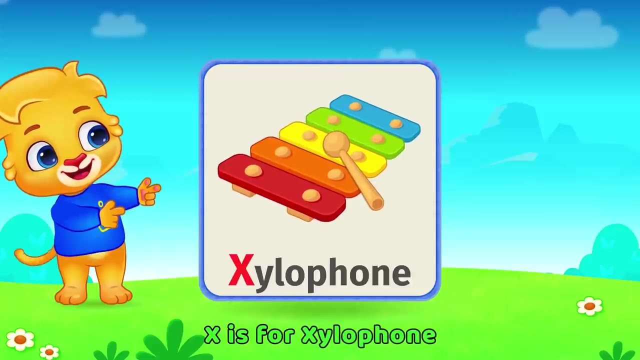 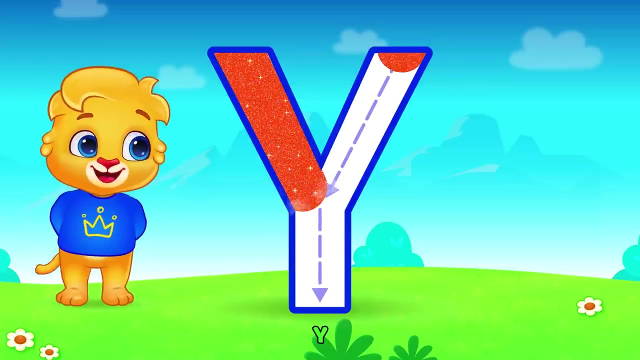 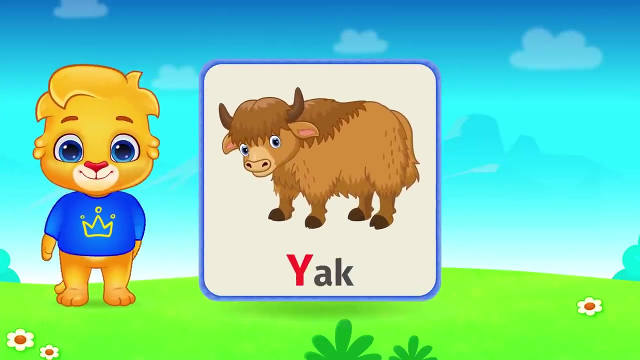 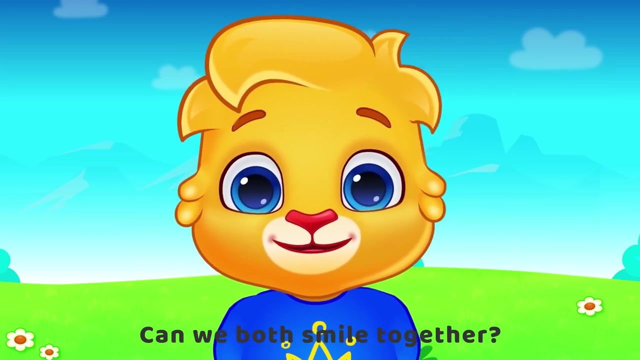 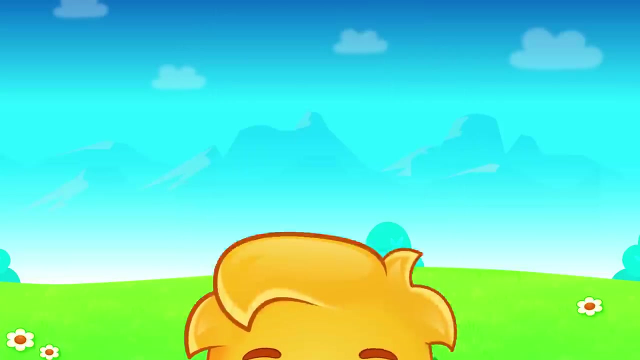 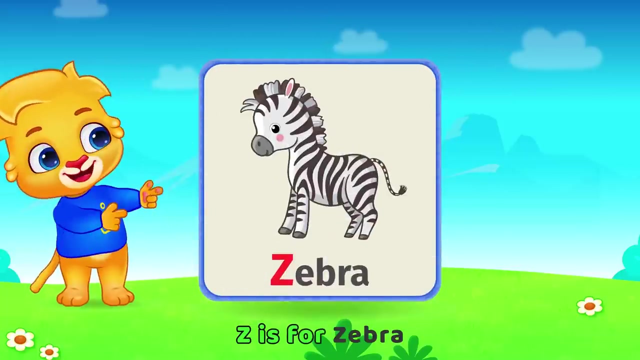 Don't you, Don't you? W is for WATERMELON, X- X is for XYLOPHONE. Wonderful Y. Y is for YAK. Hi friend, I am Lucas. Can we both smile together? Z? Z is for ZEBRA. 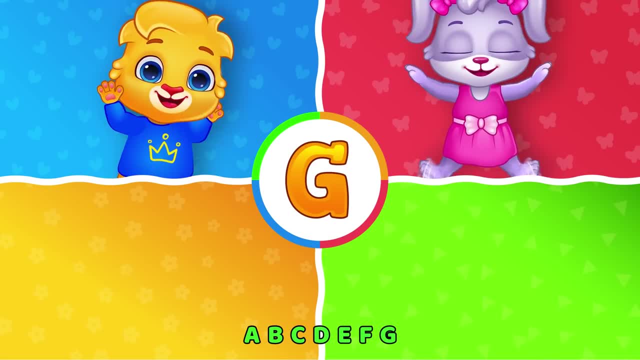 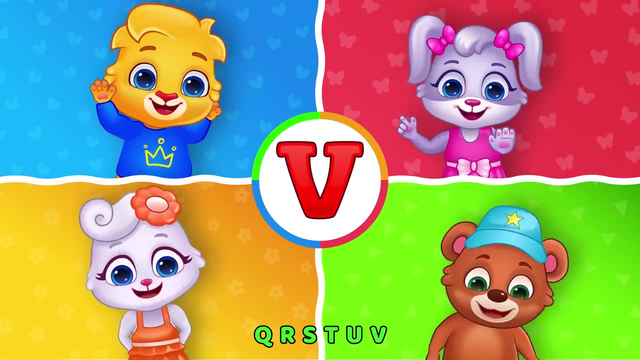 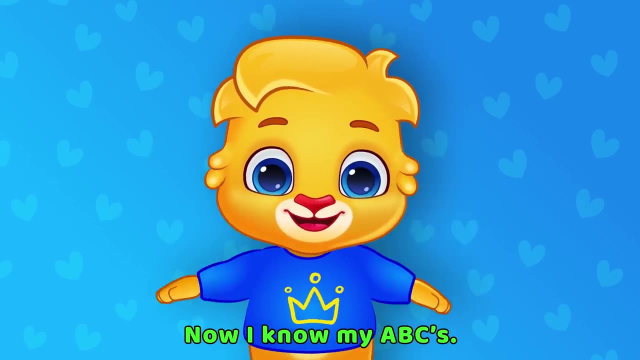 A, B, C, D, E, F, G, H, I, J, K, L, M, N, O, P, Q, R, X, T, U, V, W, X, Y and Z. Now I know my ABCs. 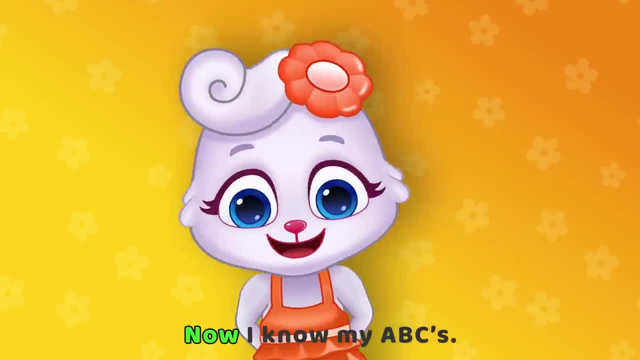 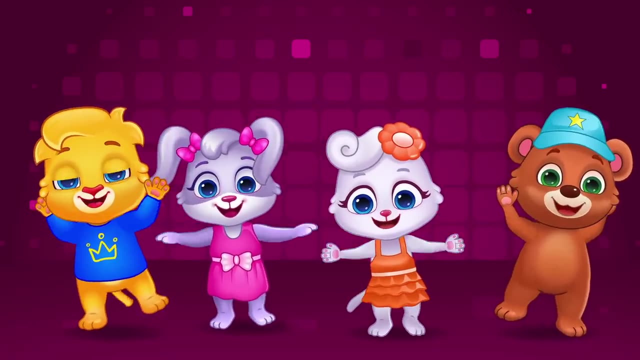 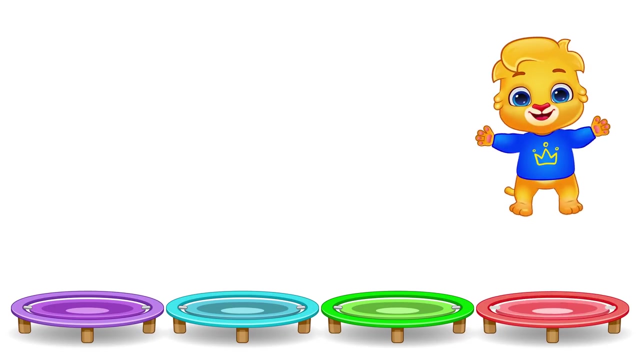 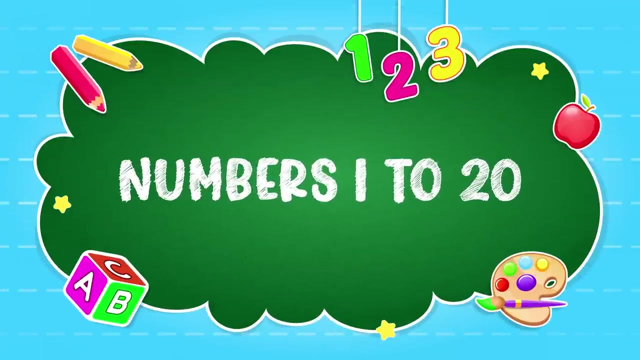 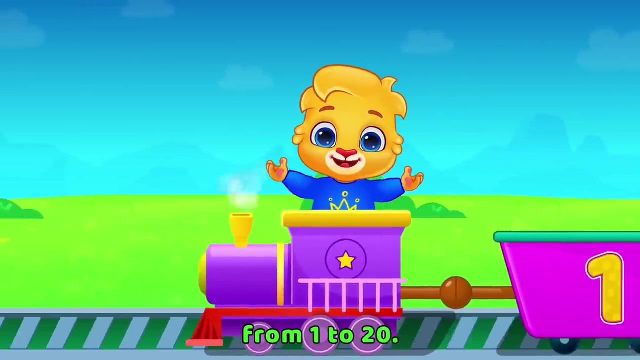 Next time won't you sing with me Now, I know my ABCs. Next time, won't you sing with me? CHIMMY, Whoo hoo, Yeah, Woo, Who, Yeah, Hi, I'm Lucas. We're going to count from 1 to 20.. 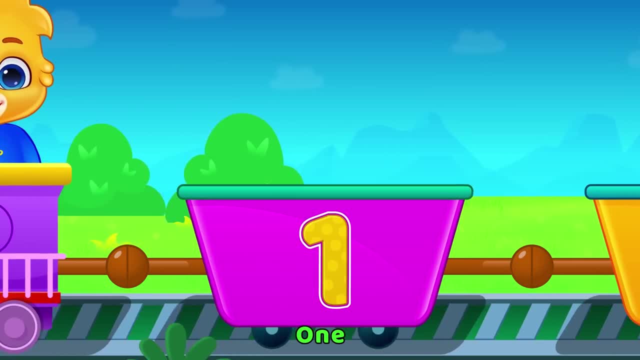 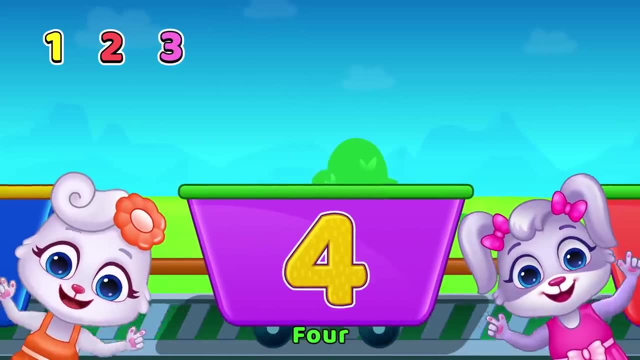 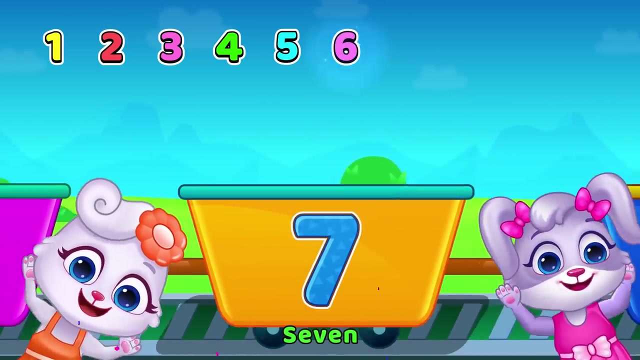 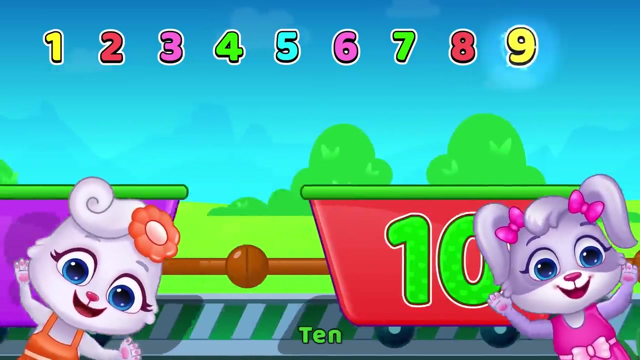 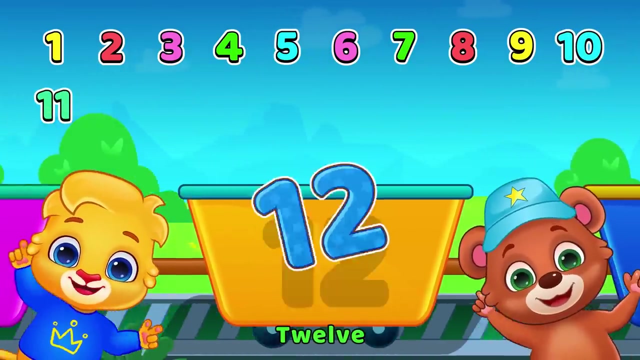 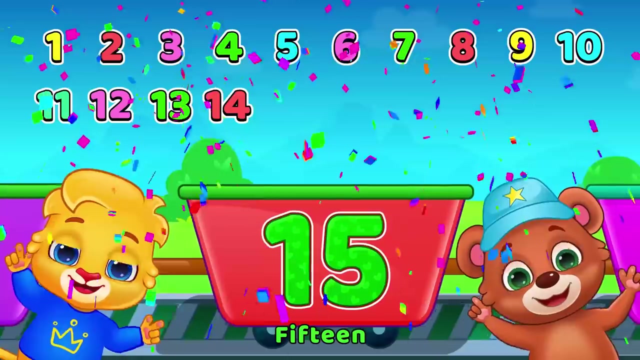 Let's go: 1, 2, 3, Four, five, six, seven, eight, nine, 10,, 11,, 12,, 13,, 14,, 15,, 16,, 17,, 18,, 19,, 20.. 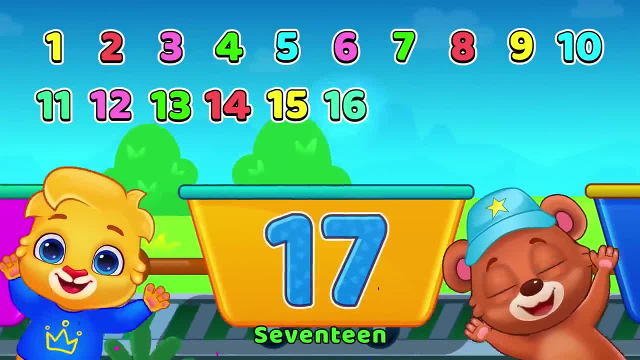 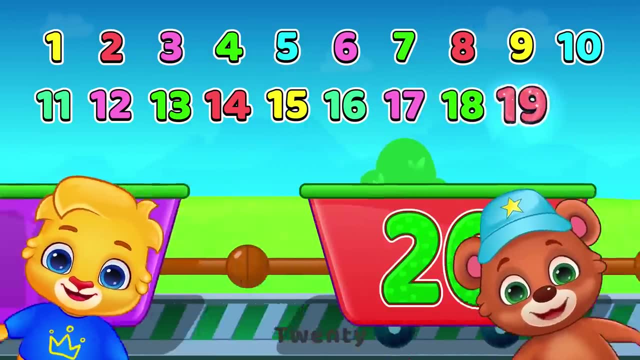 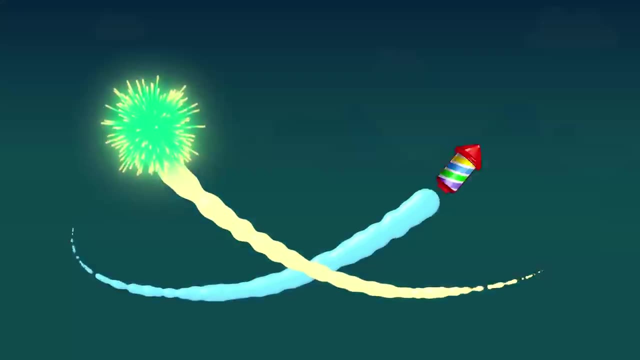 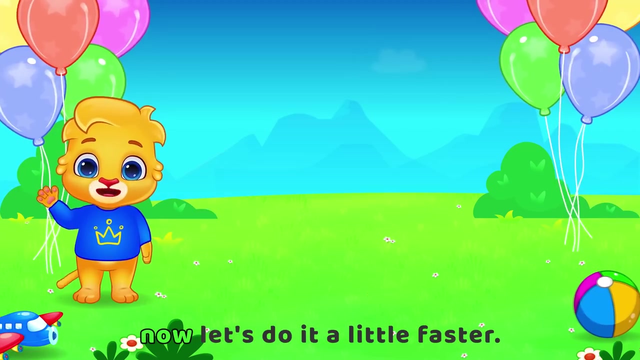 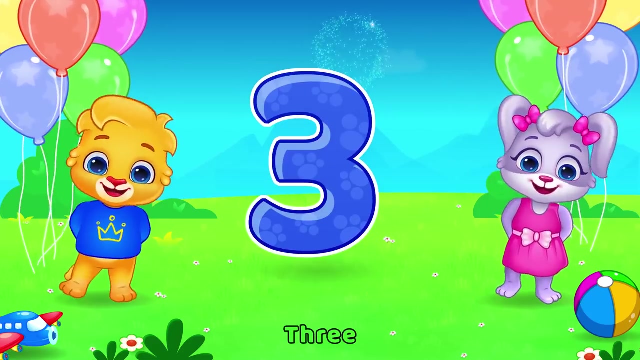 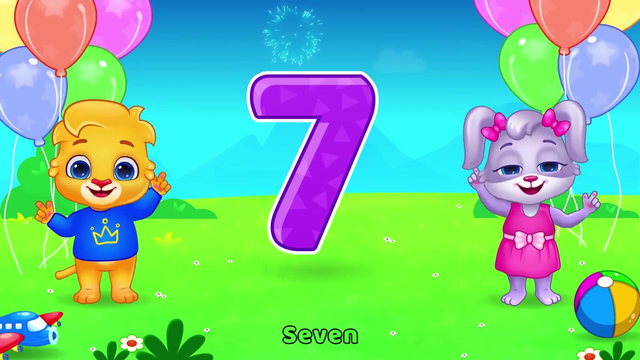 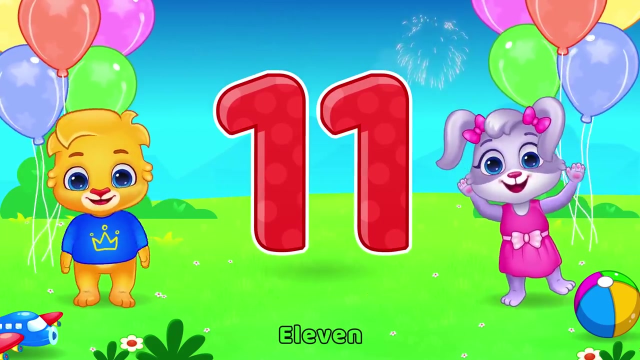 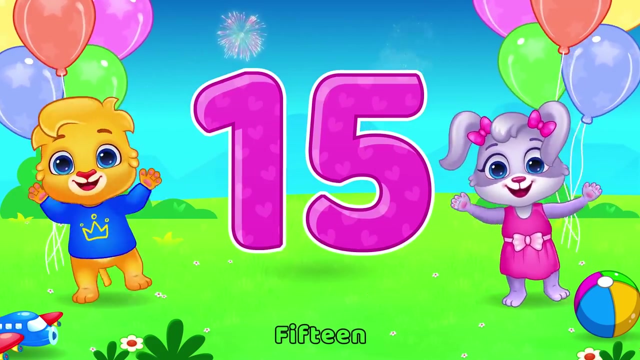 16,, 17,, 18,, 19,, 20.. Great, Okay, now let's do it a little faster: One, two, Three, four, five, six, seven, eight, nine, 10,, 11,, 12,, 13,, 14,, 15,, 16,, 17,, 18,, 19,, 20.. 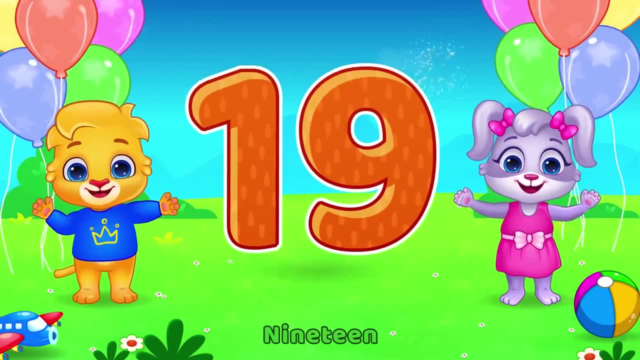 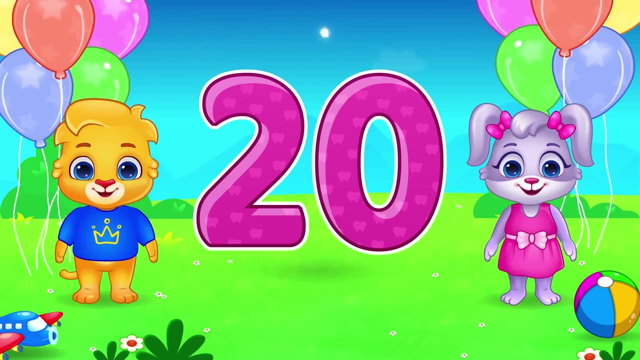 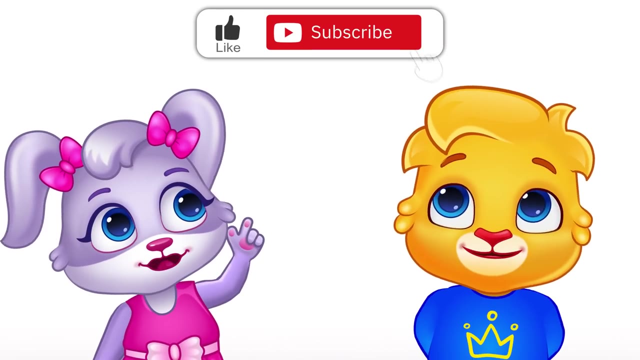 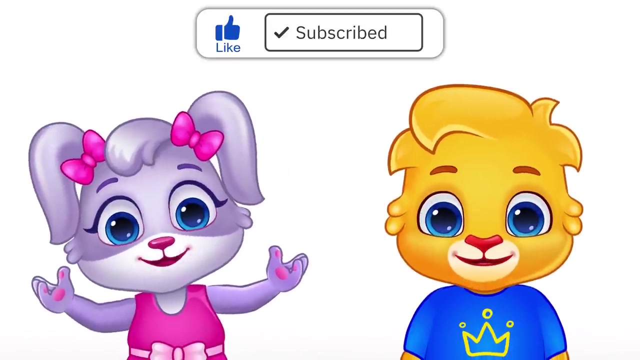 17,, 18,, 19,, 20. 20!. Hey kiddos and parents, Hope you enjoyed the video. Can you subscribe to our channel and hit that like button? It really, really, really helps recommend our video to other parents on YouTube. 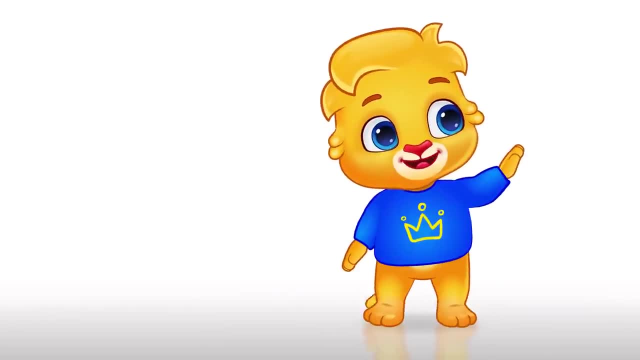 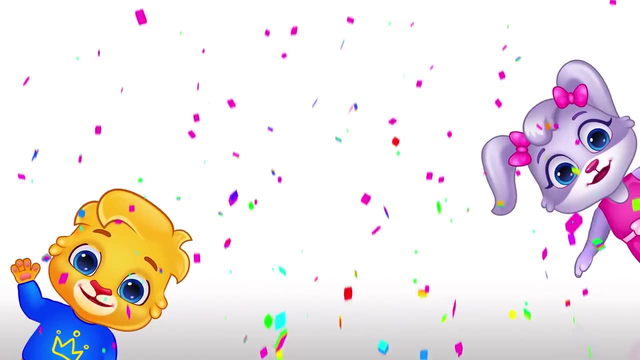 Bye-bye. Hey, Ruby, Wait for me. Bye-bye, Surprise, We're back. Thanks for watching. Can you give me a big smile before I leave? Bye-bye, Bye-bye, Bye-bye, Bye-bye. 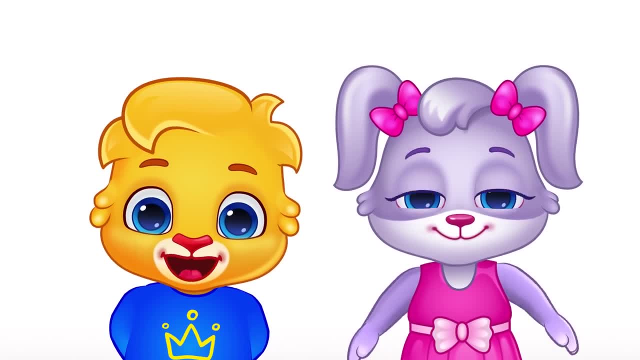